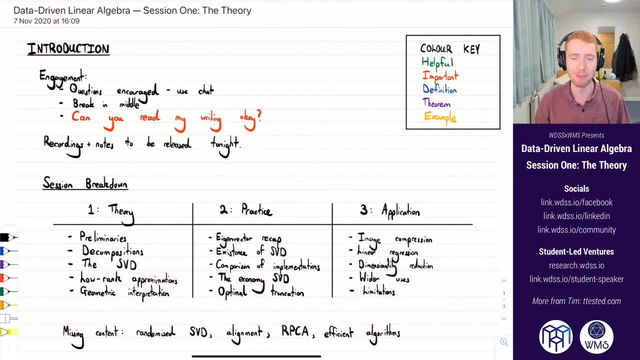 part. We're just going to have a short break in the middle just to give you a bit of time to take everything in and just relax for a second. The first question that I want to ask is just: can you read what's on this screen? all right? 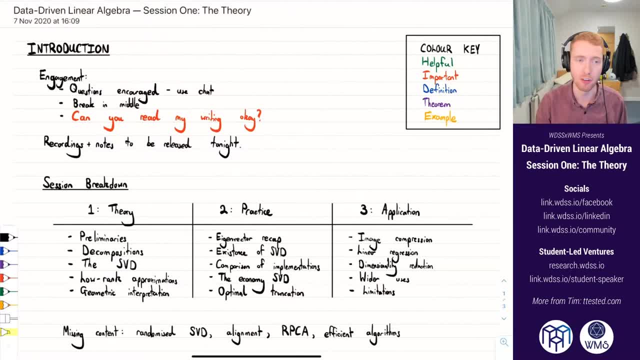 If you can't or if you can't hear me. if there's any issues with that, please pop that in the chat right now. We can get that sorted before we get started. And so also obviously, because we're streaming to YouTube, there may be some technical issues. I have prayed to the Wi-Fi gods, but 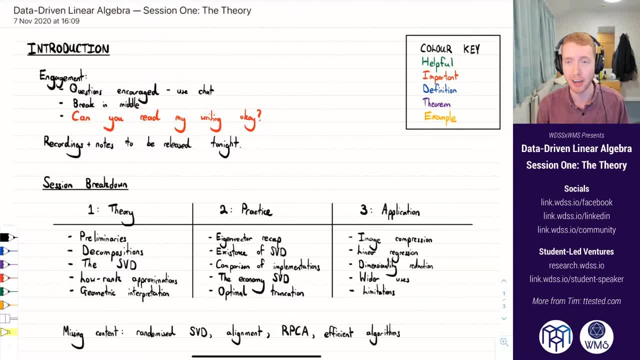 being on campus Wi-Fi. no promises there. So if there are any issues, please shout it right away. I can go back and repeat things that were lost if there's any issues. So naturally the recording of this event will be straight to my YouTube after, If people want the. 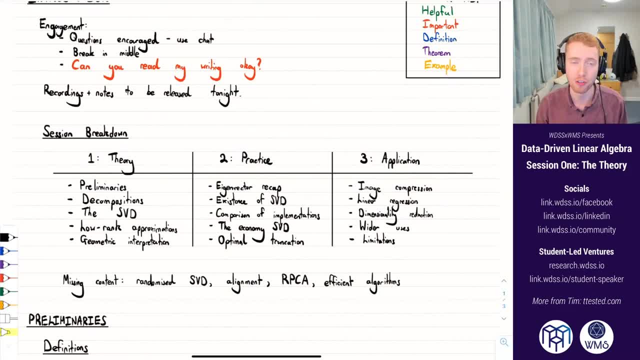 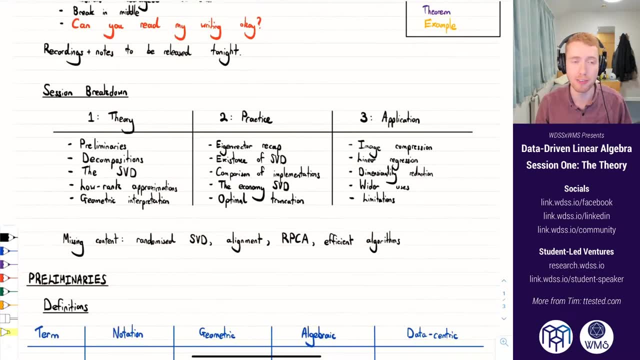 notes that I make. then I can get them sent out as well. Just send the society a message on Facebook. Okay, so let's start by. I'll just introduce myself, say a bit about my background, my motivation for running this workshop. So I'm Tim. I am the president of World Data Science Society. I am a third year. 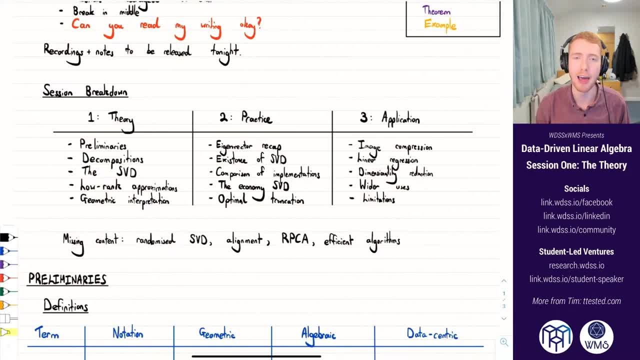 Maths- DATS student in the fourth year of my degree, having done a placement year over the last year, And so, even though my degree is in mathematics and statistics, my background is pretty maths heavy. I'm a big fan of algebra and analysis, And so I have very much an appreciation of that more heavy. 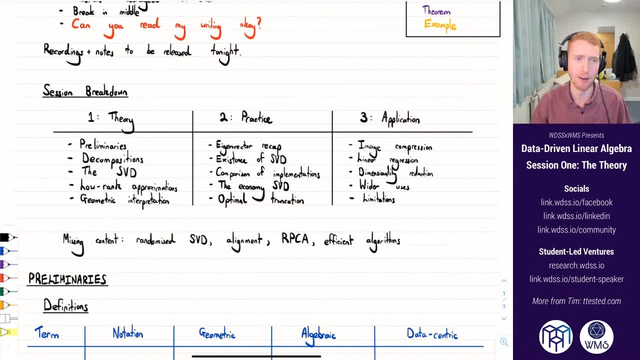 theoretical side of maths, And so some projects that I worked on related to linear algebra. just, I guess you know my qualifications for teaching. this is: I'm a developer for this package known as MyTrix, Which is a linear algebra package in Python that uses multiple dispatch in the same way that MATLAB would. 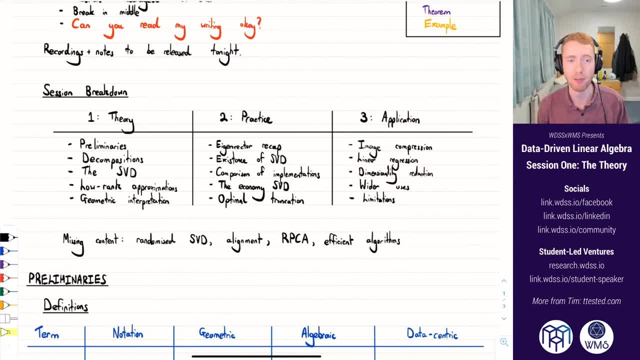 And I've also done some work in portfolio optimization in finance using kind of analytical matrix optimization methods. So in terms of my experience, I've worked at Bet365, at Dun West Hunby, which is a data science consultancy firm, And last year I spent at AstraZeneca, a pharmaceutical firm. 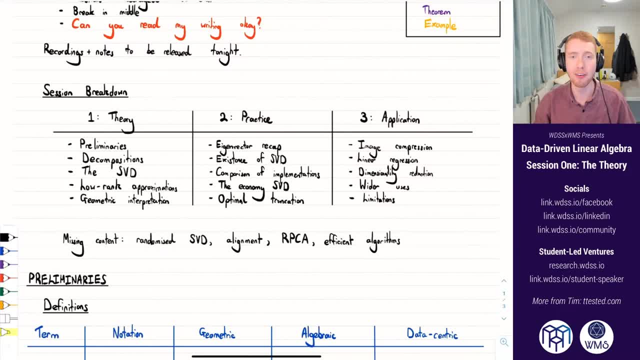 And so from that I think I have quite a wide understanding of the different applications of mathematics and statistics, And so this workshop is not going to be overly theoretical. I want to kind of focus on the actual applications and data-driven uses of linear algebra, and so hopefully that helps me in doing so, And so just 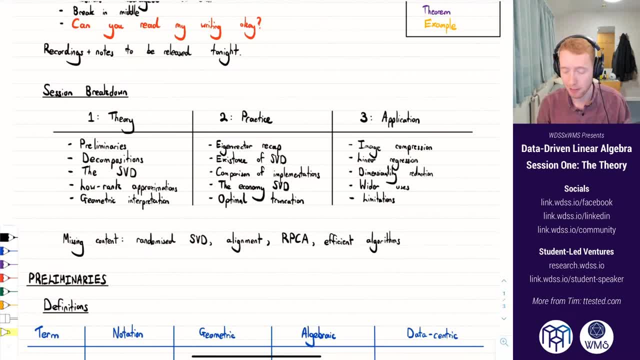 some examples of the way that I've used linear algebra in the past, just as, I guess, the motivation for why linear algebra is such an important topic to know, even if you're not a hardcore mathematician. So I did a lot of work last year at AstraZeneca on smoothing of signals, and so you might, you know not. 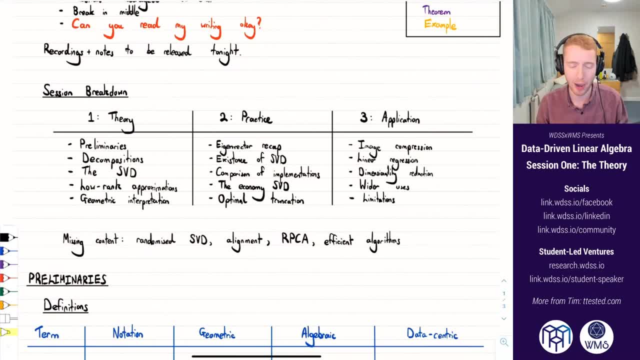 immediately see how that relates to linear algebra. but turns out that you have these complicated signals and you want to try and figure out, I guess, the fundamental signal without the noise, and there are linear algebraic techniques you can use to do that. Also lots of work on regression, so fitting lines or 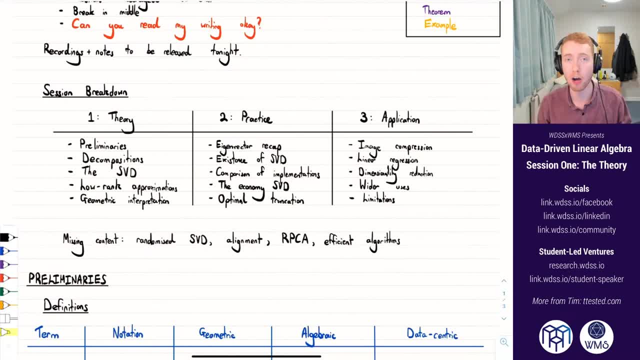 curves that best fit some data, or these things called particle filters, which are technique used to model systems that have kind of an underlying process with an added measurement: noise and process noise. And so the actual motivation for this workshop- you know why I want to teach about linear algebra- is because really linear algebra is an incredibly 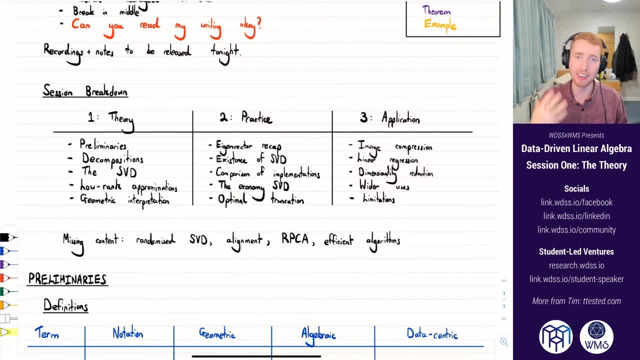 powerful toolset and, even more importantly, it's very standardised tool set. And if you can take a problem and reframe it in the language of linear algebra, then suddenly you have this wide range of tools and techniques you can apply to. actually, you're knowing those, knowing what sorts of things you can do once you have your problem. 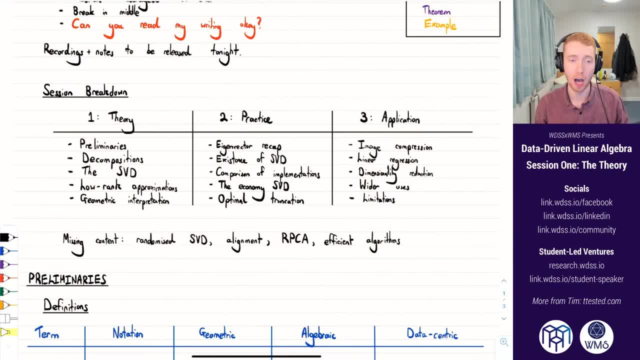 in a matrix-based form is really important and opens up a lot of applications. an example i want to share- you can have a look at later if you pop the link to this in the chat. um, this is kind of like a motivating example of why linear algebra is important. it's um a blog post i wrote about. 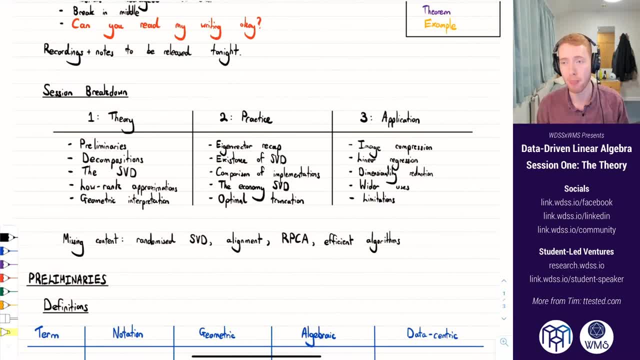 a coding question that google use um for their interviews, and the normal approach, this computer scientific approach, is using either dynamic programming or kind of some variants of that. quite you know heavy computer science techniques, um, but it turns out you can actually represent this problem as um, as a linear algebra problem, just as some matrices, and then you have access. 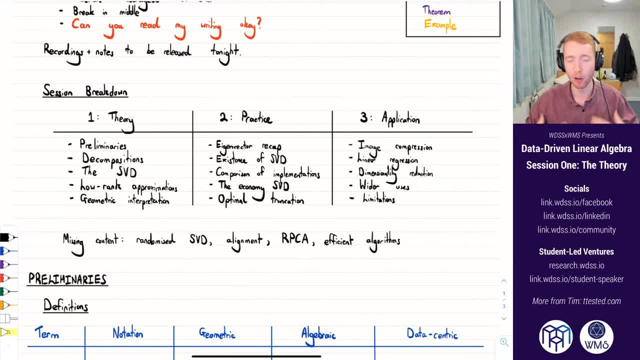 to this whole suite of linear algebra tools that, um, we learn at university and kind of in courses like this, and it actually becomes a really simple to solve problem. i think i solved in about seven lines of code compared to the normal. um, you know, uh doesn't. 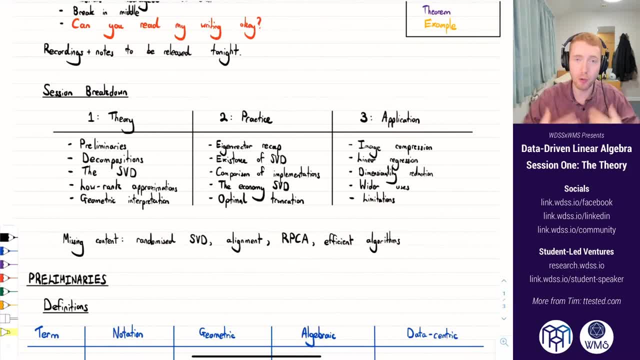 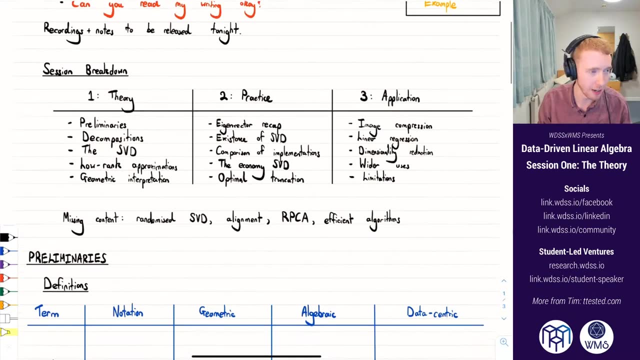 of lines, And so that's just one example of how, if we use linear algebra, we can really solve some interesting things in simple ways. Okay, so about this actual workshop. So this is split up into three parts, taught on Monday, Wednesday and Friday. So I have on my screen here what the 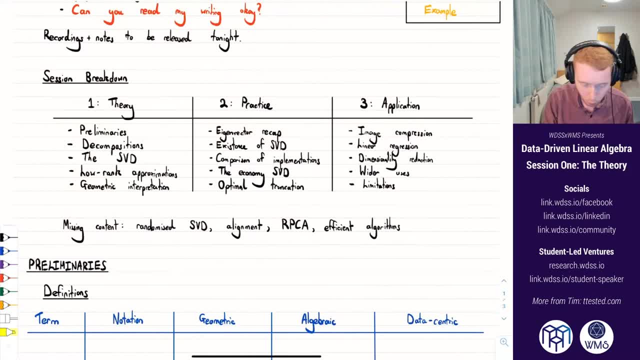 content is for the three parts. So today we're in session one and that's going to be about the theory. It's not going to be overly theoretical, it's more kind of setting up our motivations and kind of what our aims are in using data-centric linear algebra, And then we'll focus on actually. 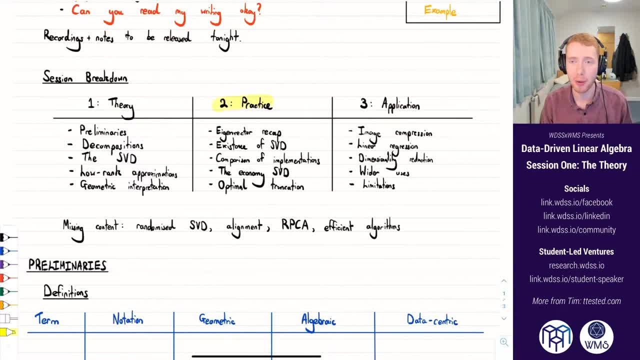 kind of the practical application on Wednesday how we can actually by hand compute some of these things we're talking about, And then on Friday we'll look at the application of these using coding. So we'll use a bit of Python. we'll also get translations in other languages. 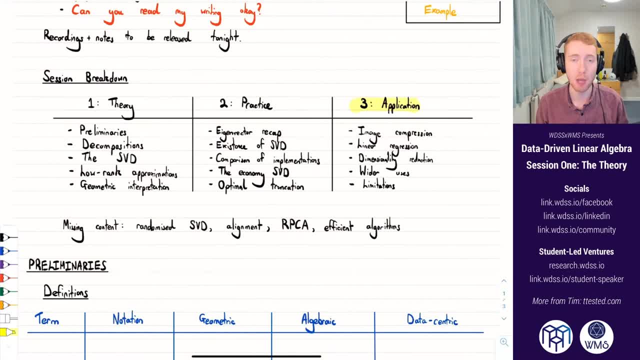 and actually see how we can apply these to some real problems. And you may have seen on WDSS's Facebook, This is an example of using these techniques to compress the image of a cat. We'll look at examples like that, And so we'll return to talking about exactly what we're going to be doing in session two. 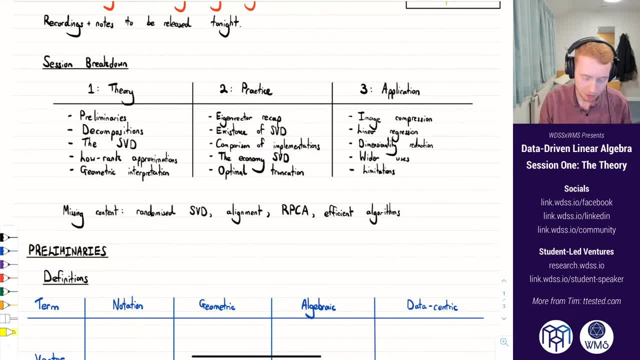 and three when we get to those sessions. But today we have five things to look at. So first, some preliminaries, just getting everyone up to the same standard. We're expecting very little prior knowledge for the session, so we're going to just work through a few things. We're then going to look. 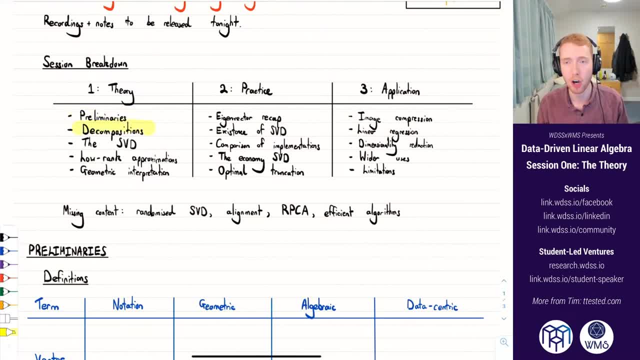 at this thing called well, these things called the singular value decompositions, and kind of explain what a decomposition is And then learn about this specific decomposition called the singular value decomposition. And that's really the prime focus for this entire workshop series. This thing called the singular value decomposition. it's a really 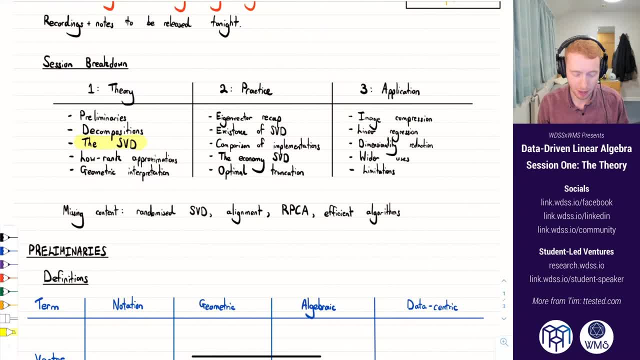 important tool in a wide variety of fields. I'm going to learn what it is and how to use it in practical examples. We're then going to look at this thing called low rank approximations. That will make more sense when we get to that. 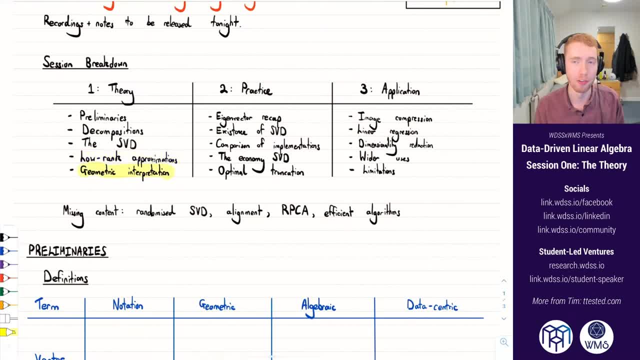 And then, finally, a geometric interpretation of what the singular value decomposition means, And so a few notes on the style of this workshop series I'm going to be presenting in a similar way to how a normal lecture would be taught, but hopefully being a bit more open to questions. So, if there are any, 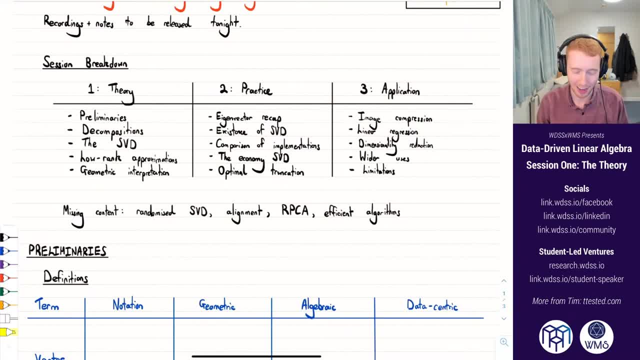 questions, please do ask up. It's very important to catch any issues early rather than just trying to go along if you're not following completely. I try to kind of improvise when I'm teaching a bit more. I think just copying out from notes is a bit boring and unengaging. 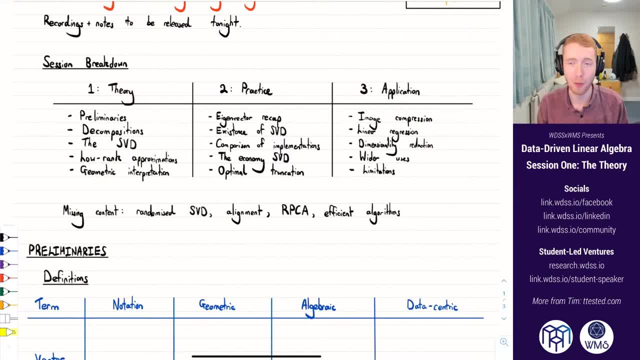 But the side effect of that is that I will make mistakes. So if you do spot anything that looks a bit strange, either point it out or just say: you know, can you explain that thing again And I might spot it for myself. 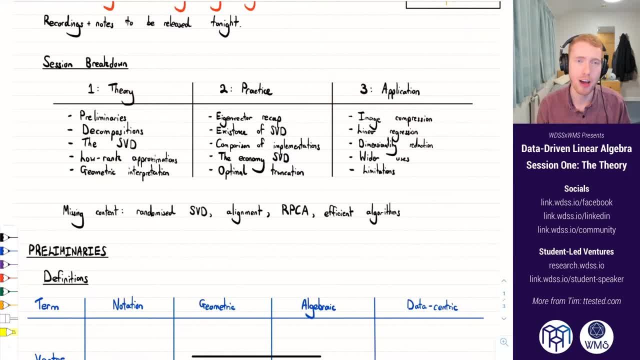 And so we are going to go through this content fairly quickly because we want to discuss this whole topic and its applications in three workshops, So I wouldn't worry too much about taking notes. That's not really the idea of this. You can come back later and review it. This will always be up on YouTube. 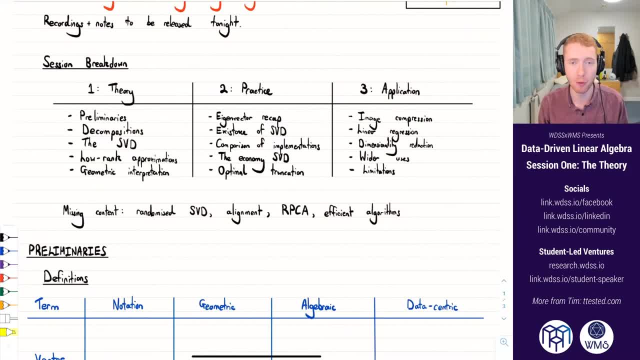 But you might want to jot down some key ideas. If there's something you haven't seen before, especially definitions, then it might be a good idea to just put them down on some paper somewhere so you can refer back to them if you need it. 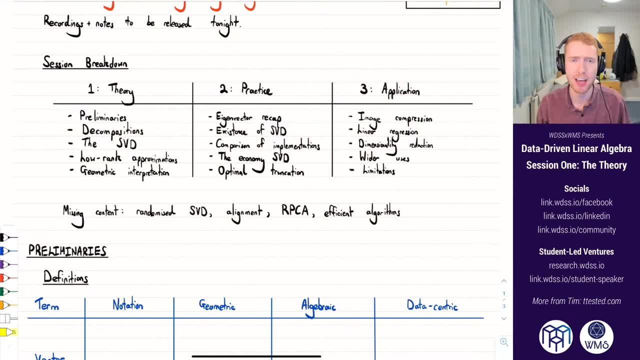 But yeah, you can come back to the recording at any point. So really, just sit back and try and take it in. And so yeah, prerequisites: they really are none. If you have an A-level understanding of matrix algebra, that's wonderful. 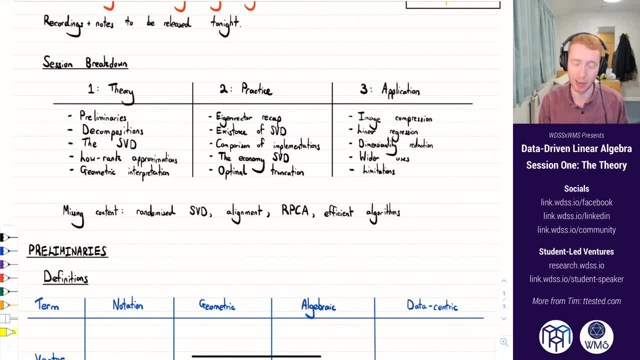 The important thing to bear in mind, though, is that if you don't have a good understanding of matrix algebra, you're not going to be able to do it. If you have a good understanding of matrix algebra, that's wonderful. The important thing to bear in mind, though, is that each session depends on the last. 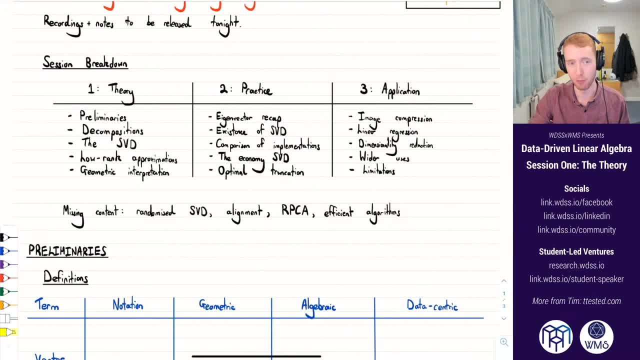 So to do session two and three you will need to have watched the previous ones, And also we'll be doing a bit of coding in session three. There's going to be no prerequisites for that. I'll make the code as clear as possible so you should be able to follow along even without knowing how to code. 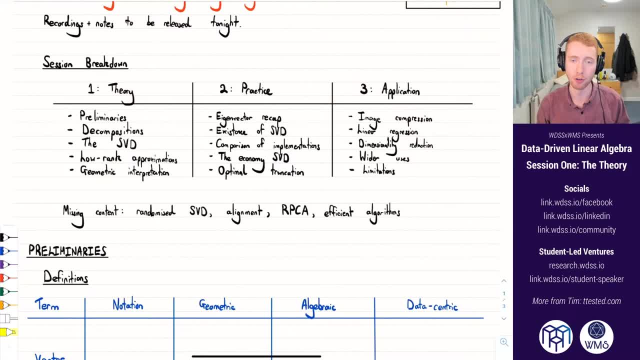 That will be in Python, but we'll get translations in MATLAB, Julia and R sorted. Those will go up on the Facebook event page at some time fairly soon. OK, so the actual motivation for learning about data centric code. OK, so the actual motivation for learning about data centric code. 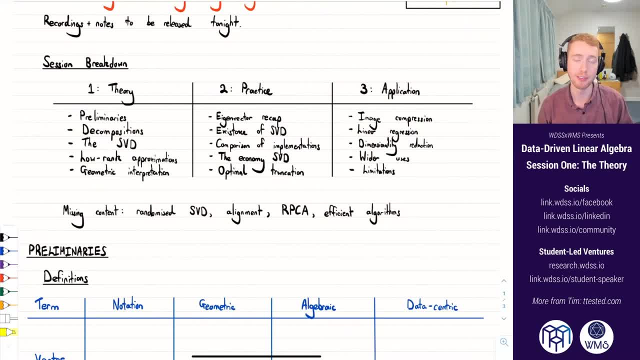 OK, so the actual motivation for learning about data centric code. So if you want to learn more about linear algebra and specifically about this thing called the singular value decomposition, So if you want to grow your system- remember, I've gone through alphabets like Goobledy and being really crazy- 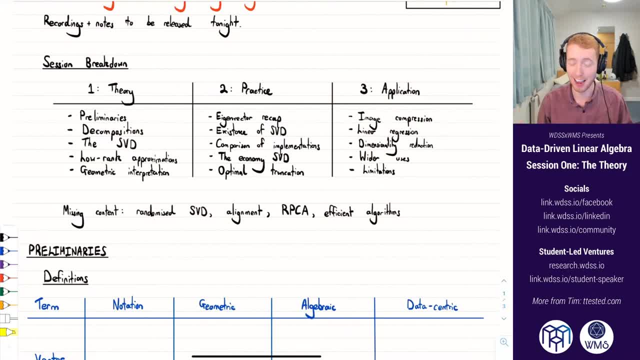 You're just constantly getting theě. The singular value decomposition is probably the best way to do that. The singular value decomposition is probably the best way to do that because it's used in a wide variety of fields: in statistics, in signal processing, machine learning. it's critical. optimisation problems, managing portfolios in finance. there really is a massive variety of things it's used for, And it's also useful in theoretical maths. you can use it as a more elegant way of solving problems that would otherwise be a bit tedious. 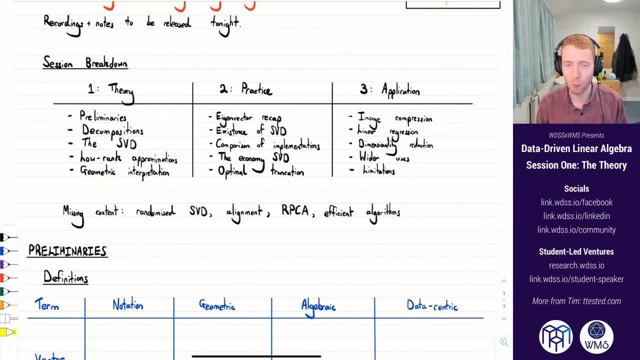 And so you may be wondering: okay, this sounds very important, why haven't I heard of it? If it's so important, why isn't it in my first year algebra course or something like that? And the reason is, you know, it just takes time for universities to update their syllabus and change to a new world. 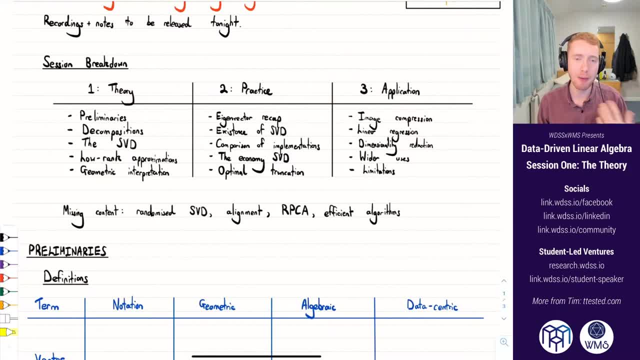 because the thing about decomposition: it's very powerful for data centric applications And often when you want to apply in practice you'll need a computer to actually calculate the values. But that's not a problem. now we have fast computers and we have lots of data. 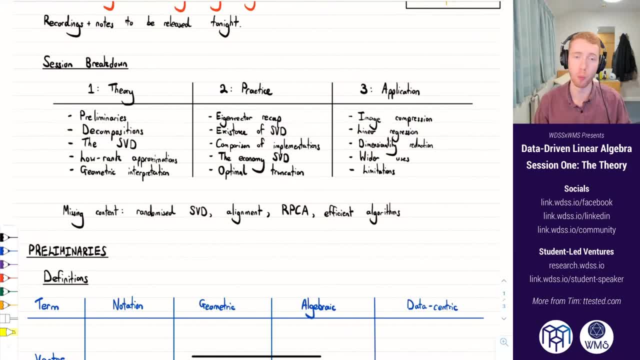 And so the thing about decomposition is becoming more and more important With time. actually, MIT, in their linear algebra course, that introductory one, they recently updated it a year or two ago, to include the singular value decomposition in the beginners course. So it is starting to take hold of the academic scene. 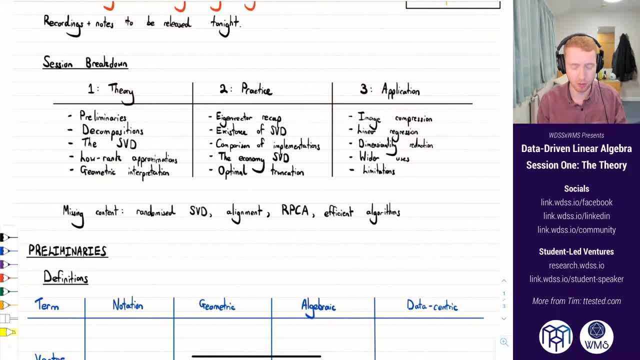 So at a very high level. you know what is the singular value decomposition? we'll define it properly in this session, But just as some kind of motivation before we get there. it's essentially a tool for reducing the dimension of our data. you can imagine we're working with. 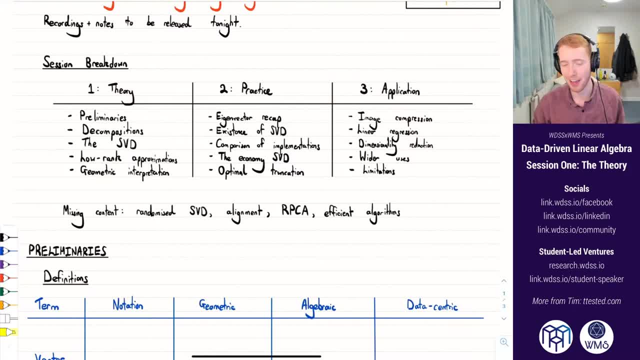 some really complicated data in really high dimensions, and each bit of our data is, you know, a million dimension vector, and that's too much for a human to work with, And so the idea of the singular value decomposition is to reduce that into fewer dimensions, taking the most important features of our data. 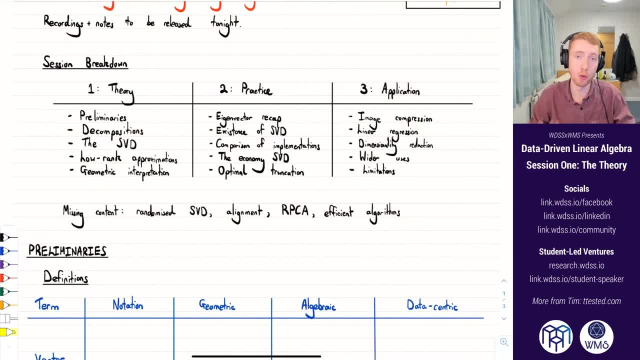 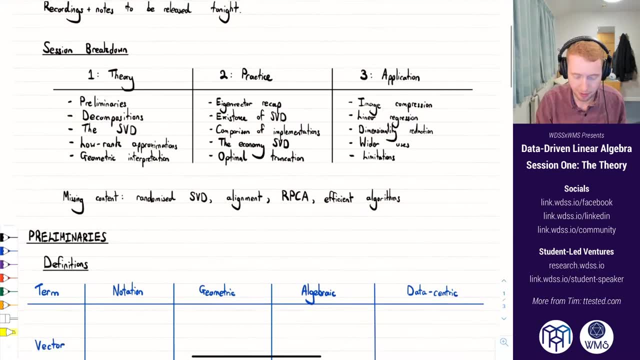 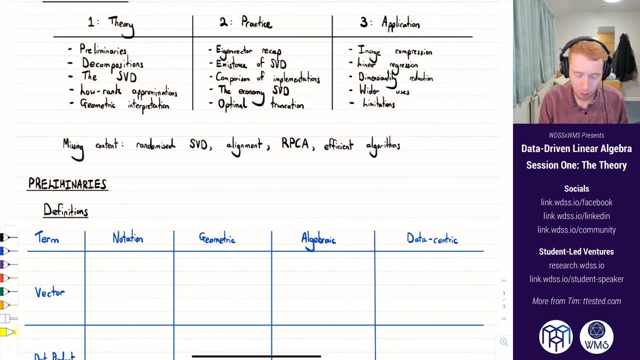 to have this really dense representation that actually has a lot of intuitive understanding and getting rid of the noise and unimportant bits of the data. Okay, so that's all kind of the setup. It's also worth mentioning that there are a few things we're not going to cover, just in the name of time. there's this thing called the randomised SPD. 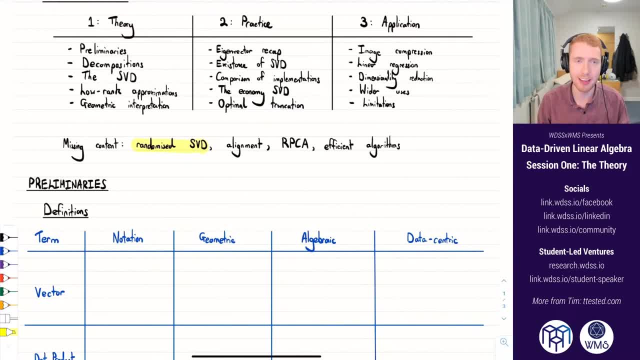 And that is an algorithm kind of based on these ideas of a randomised linear algebra. it's a fairly new field And it's a really clever idea. have a search for it after these three workshops if you're interested. we're not going to deal with issues of alignment again. just Google it if you want to know more. 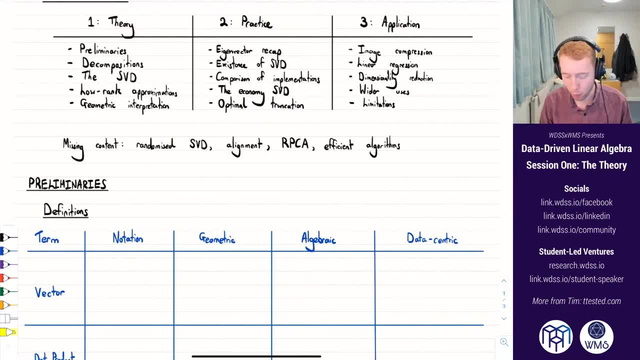 Kind of robust estimates. so the robust principal components analysis. we'll talk about the principal components analysis in session three. there's a robust version which works for missing data. that's kind of the backbone of Netflix's recommendation system. We're not going to explain how that works, But again, you can search up for it. 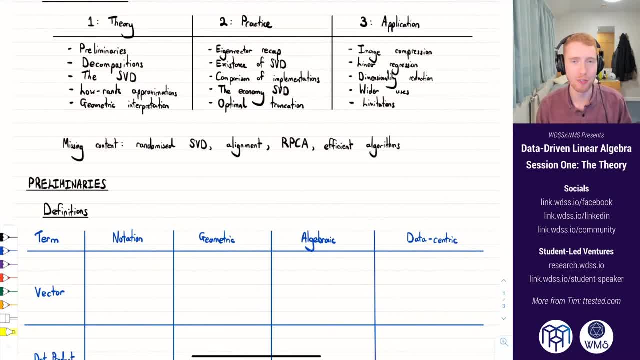 Also, when we actually do the singular value decomposition, we're going to use a very inefficient algorithm. it's a simple algorithm. that's why we're going to teach it, but it's not the most efficient way of doing things, So we're not going to get into the details of efficient ways of computing it. 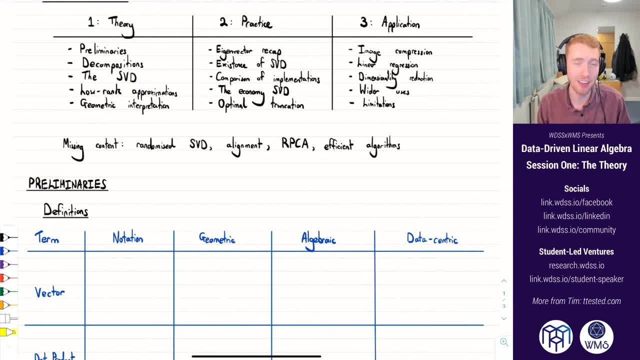 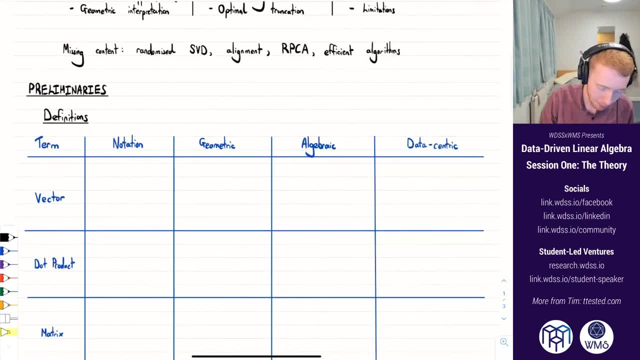 For that. we'll just get Python or MATLAB or whatever to do it. we won't understand the algorithms they're using, but hell don't worry about it, They're fast, so we don't care. Okay, so we're going to start off with some preliminaries and, specifically, some definitions. 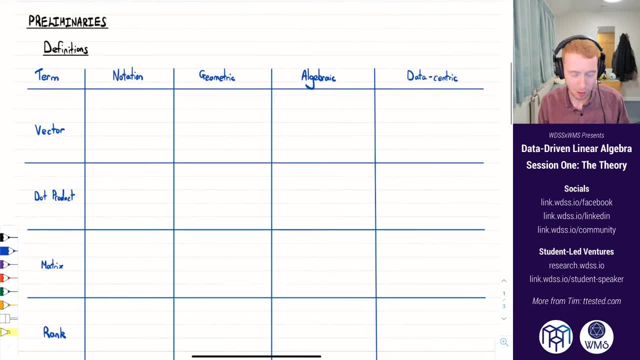 And so if you're, you know, very familiar with an algebra, you might be looking at this and going, okay, this is a waste of time. I know what a vector is, I know what a matrix is, But what I want to try and introduce to you is different ways of thinking about these concepts that you might know already. 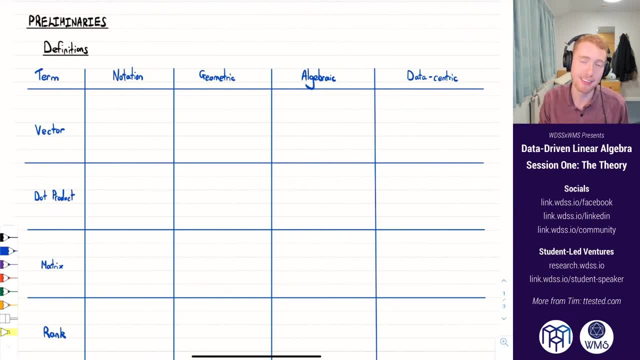 And specifically geometric, algebraic and data centric interpretations of these ideas you might know already. So we're going to start with a vector. so a vector is basically a column or, I guess, a row of numbers, And so we might write it something like this: so we have a vector v, and it contains values v1,, v2, all the way down to vn, and we also might represent this as a row vector, in which case we would use the little t symbol, mean transpose, and that would look something like this: 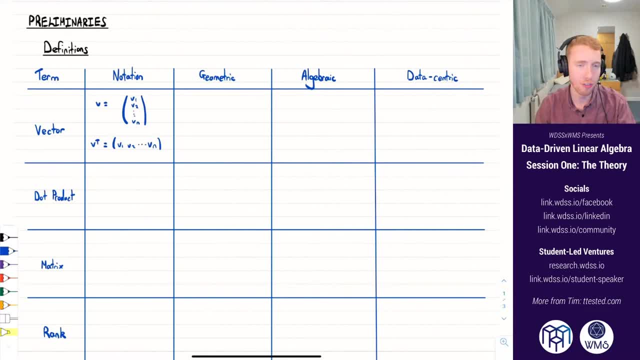 Okay, So if that is our vector, what does that mean? you know what is a vector? Well, let's start with the geometric intuition of a vector, And I'm also going to mention throughout this entire session: we're going to be sticking to real numbers. 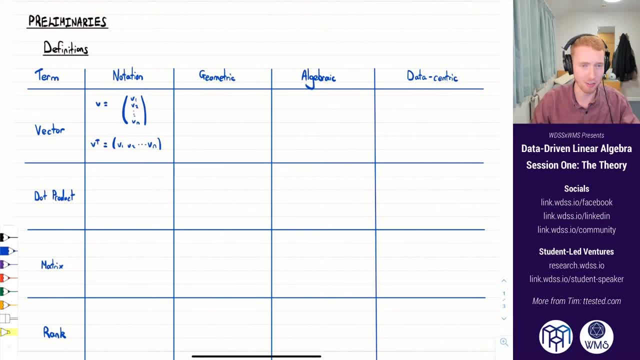 So no complex numbers, no kind of integer fields or anything complicated. we're living in the world of normal decimal numbers. So what a vector is? essentially it is a point in an n-dimensional space. So each of these points here in the vector, those give you one coordinate out of n dimensions. 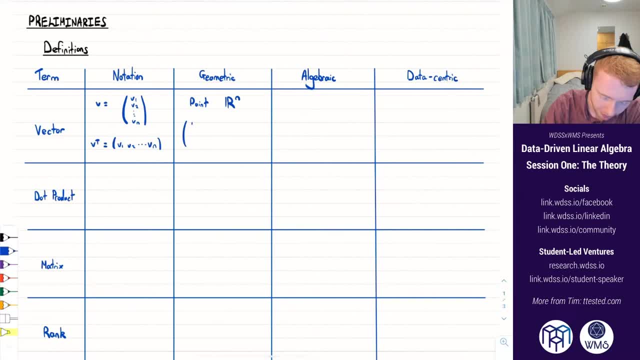 So you can imagine, in the case we had a vector like 1,, 2, and 3, we're in a three-dimensional space. let's have a go at drawing that something like this, with our coordinates x, y and z. 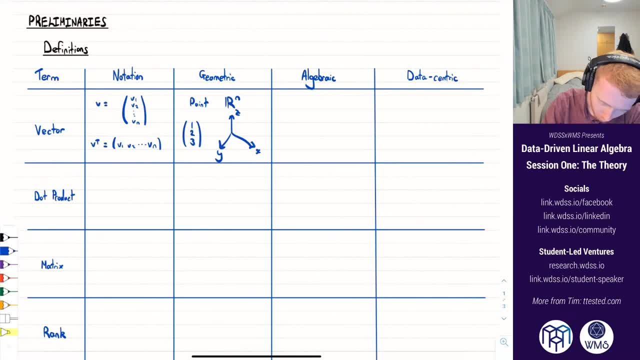 And then this vector has x coordinate 1,, y coordinate 2,, wait, so y coordinate 2, I've done these in the wrong order here. So y coordinate of 2, and then z coordinate of 3.. So at some point up there, 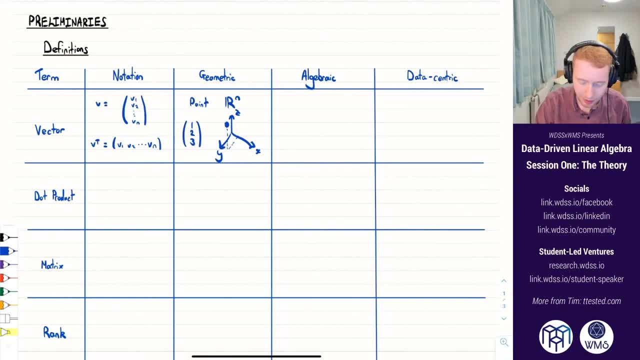 So that's all a vector is. So, algebraically, we would consider a vector to be an element of this thing called a vector space. Now, this is very technical. we're not going to get into exactly what this means, but it just shows that you know there are different ways of thinking about these concepts. 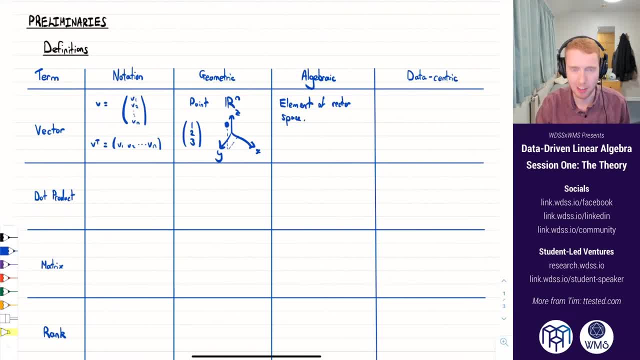 And a vector space. yeah, we're not going to mention what that is. It's basically a thing. There's these eight key elements. There's axioms, or we'd call those rules in quotes there, not a technical name for them. 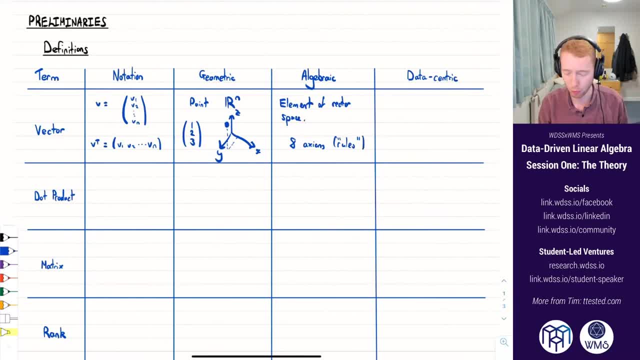 And vectors are things that basically obey these rules. And so, in a data centric view, what is a vector? Well, it is. It is data. Essentially, you can think of a vector as either an observation or a predictor, Or kind of a response. 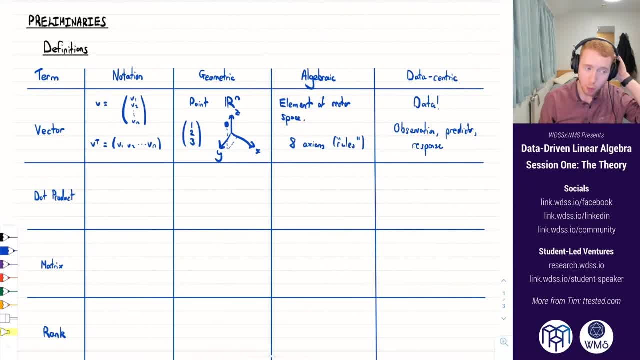 A variable, like something you're measuring. So we could imagine here that this v transpose all this, is it's all the data about a certain person. It's like one row of our data set And each of these v's gives some kind of measurable property about that observation. 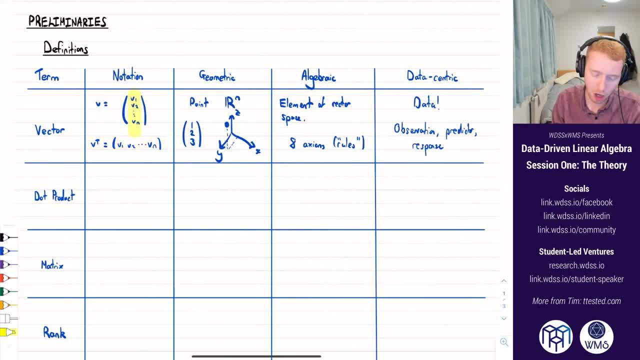 And in a similar way, a column vector like this might represent, for different people, all the values of one measurable property. So that's one way of thinking about a vector. So let's next talk about this thing called a dot product. So we would denote this either with a dot. 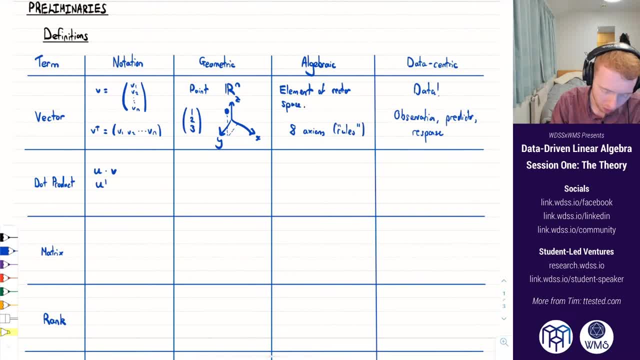 Or sometimes we might write it like u transpose v Or something like this. This is known as the inner product notation, So this is a thing called a dot product. You might have come across it before in A level maths, but we'll define it here. 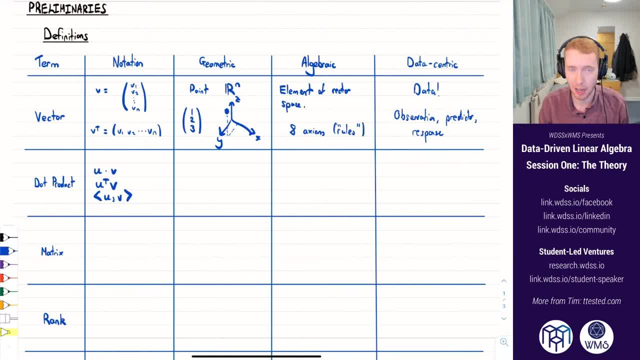 So let's start with the algebraic definition of it, Because this is the actual kind of how we would compute it If we have u dotted with v. All that means is we take each element of this vector u And each element of this vector v. 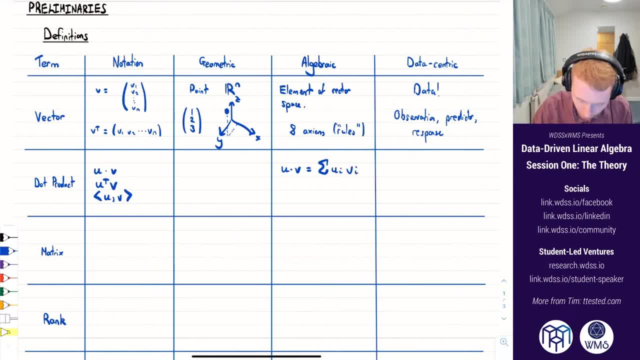 And we multiply those together. And so we do this from i is 1 up to n, So we just kind of take these two vectors side by side and times them across and add up all of those products. And another way to think about this is as when we do u transpose v. 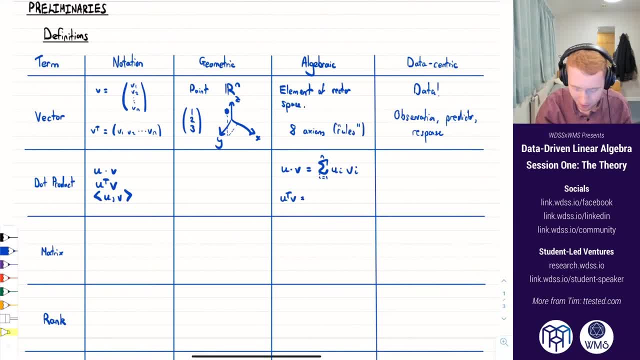 Is thinking of these vectors kind of as matrices. We'll explain what matrix is in a second. But this u transpose is something long and thin like this: And then this v1 is something tall and thin And we can think of this as just like a matrix product, between these different terms here. 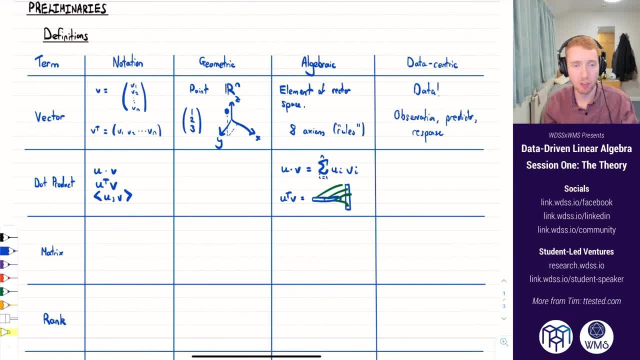 So that's another way of thinking about that. But, geometrically, what is a dot product? Well, one way of thinking about it Is that it's got something to do with the angle between any two points. It's the angle between two vectors, say 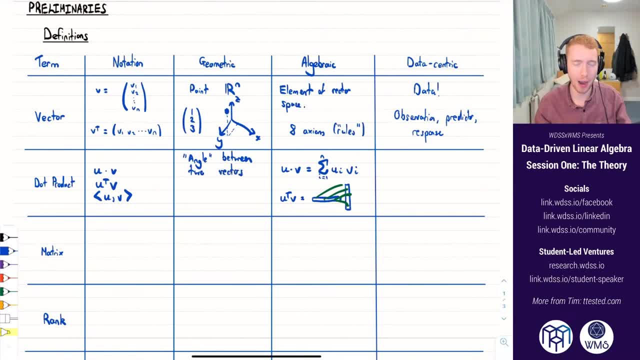 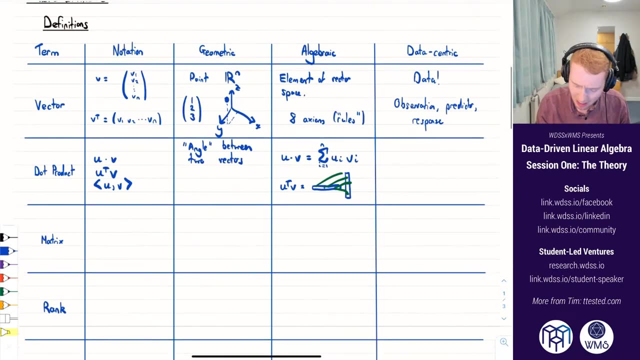 And it's a bit more specific than that. You have to normalise these vectors first, So they have a length of 1.. But essentially a dot product is talking about what is the angle between these two points, Or these two vectors, And there's not really a data centric interpretation of a dot product. 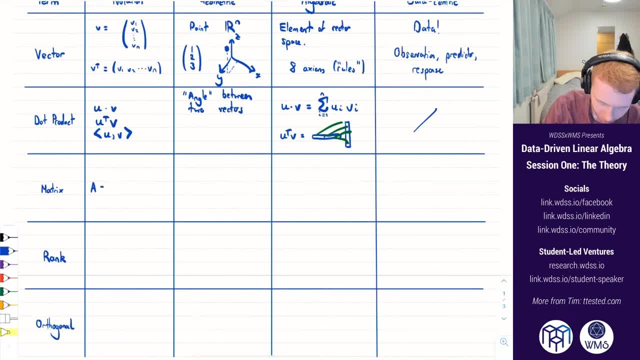 So we next have a matrix. Well, a matrix is just some entries here. Let's call them a1.. And it's going to be an m by n matrix. This is going to go up to a1 n All the way down to am1.. 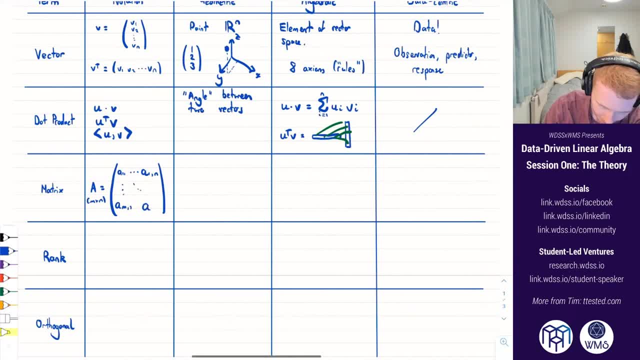 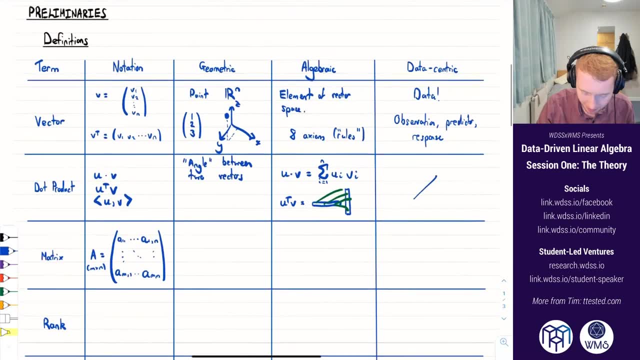 And all the way down here to m and n. So it's basically just a grid of numbers. And how can we think about this geometrically? Well, this is kind of a linear transformation. And so what do we mean by a linear transformation? 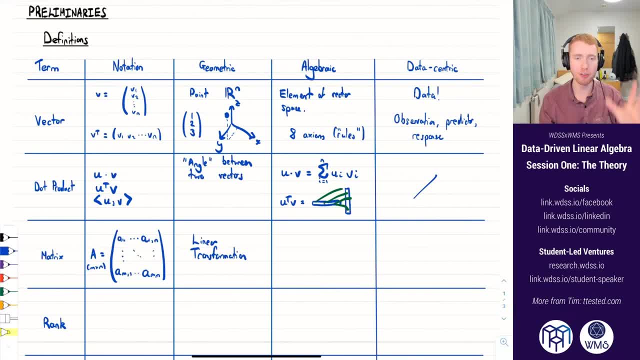 We basically take some sort of space, Say you know three dimensions, And do something to it. And when we say linear, what we mean is: Well, there's two ways of thinking about it. One is that parallel lines stay parallel. Another one is that lines get transformed. 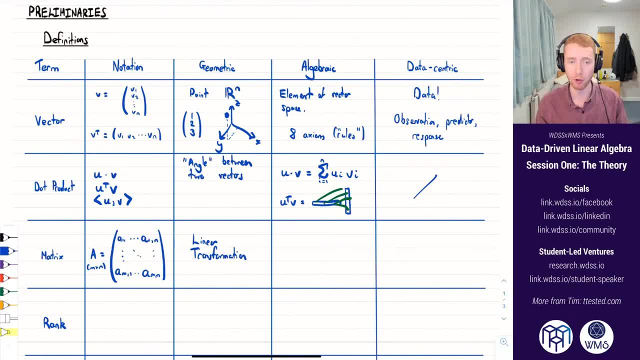 Sorry. lines through the origin get transformed into lines through the origin. So that's one way of thinking about it. You know, rotations, reflections, scaling, stretching, skewing, Those are all linear transformations. Algebraically, we think of this as a linear map. 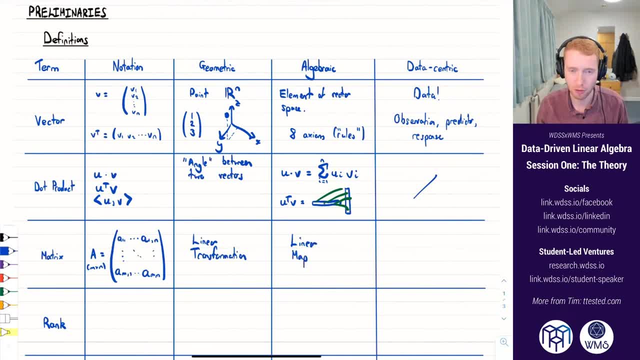 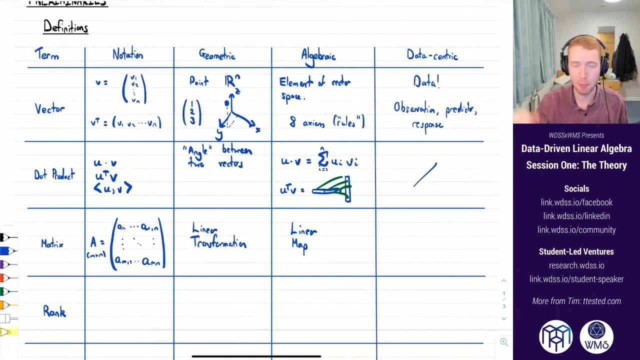 I'm not going to explain exactly what that means. It's not really the focus of this course, But that's one way we can think about it, And in a data centric sense, And this might be a bit of a new idea to people. 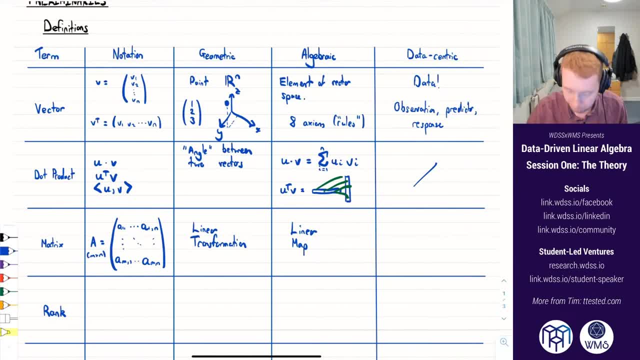 But it's a very nice way of looking at a matrix Is as a data set. If I have a matrix A, I can think of it As either a collection of row vectors Or a collection of column vectors. So, for example, I can think of A. 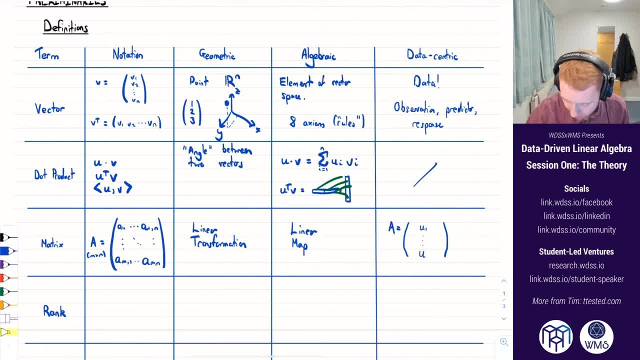 As multiple. So this is an M by N. So it's going to be M of these Multiple row vectors And we're going to transpose those because they're row vectors, Like we saw up there. Okay, So that's one way we can think about a matrix. 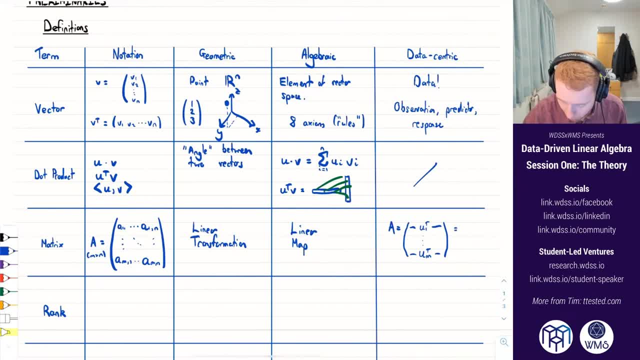 As these row vectors, Or another way. We'll be thinking of things as column vectors, So going up to N now, Because there's N columns, And thinking of them as these different columns here, And so that's a very nice way of thinking about matrices. 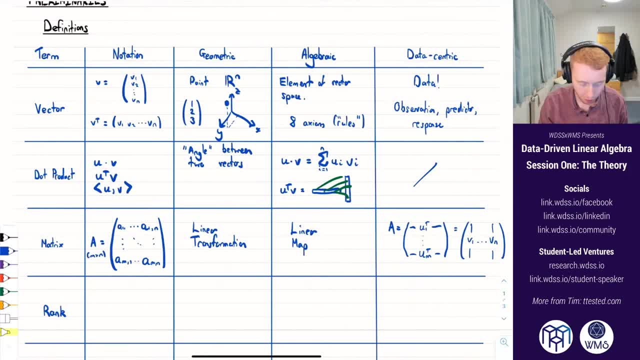 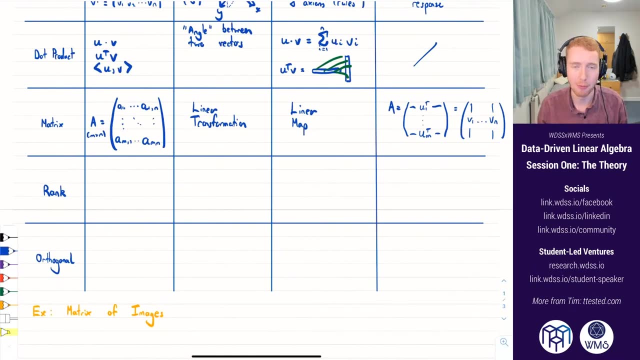 Rather than their actual individual elements. We think of them either as collections of observations- These rows here- Or collections of predictors, Things we can measure. Okay, So two more things we're going to talk about, Then we'll actually get on to talking a bit more about the bulk of this course. 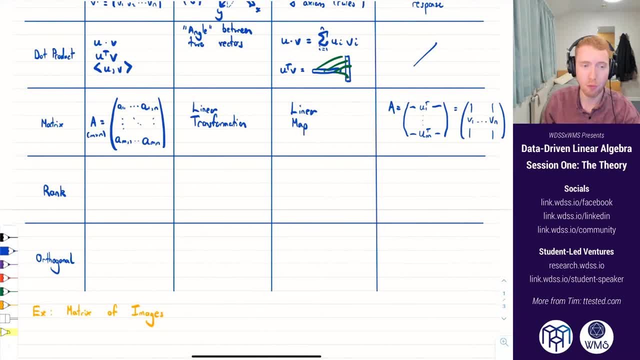 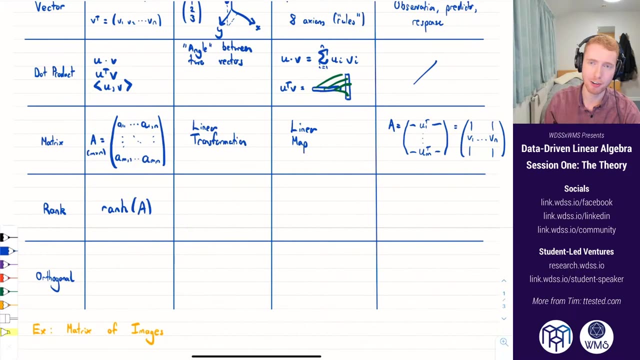 The single value decomposition. What is the rank of a matrix? And we would denote this simply as rank of a matrix A. So let's start with the geometric definition of this. So, geometrically, what the rank of a matrix kind of represents Is, if we took a unit sphere, 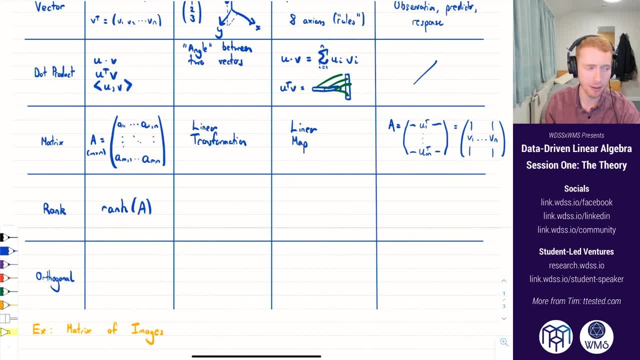 So imagine we're in three dimensions. We'll take the sphere in three dimensions And then we're going to transform that through the matrix And that might get turned into maybe an ellipsoid, Or it might get flattened down into an ellipse, Or maybe even just a line or a point. 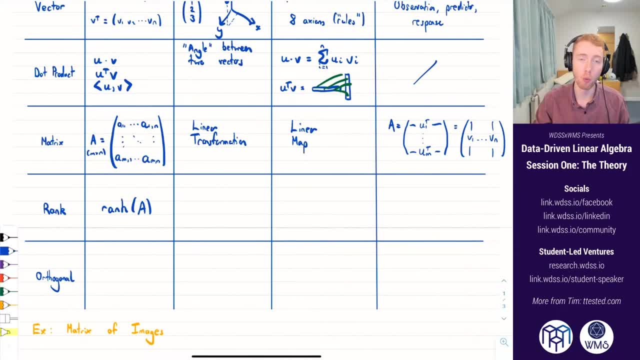 And the rank corresponds to what dimension this resulting sphere is going to be After we transform it. So it's the dimension of a transformed sphere, And we'll come back to this right at the end of this session When we talk about the geometric interpretation of the singular value: decomposition. 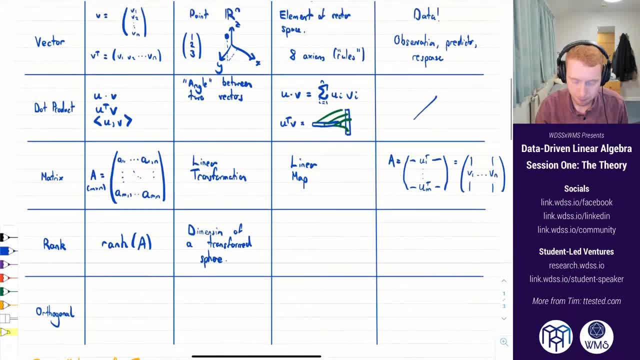 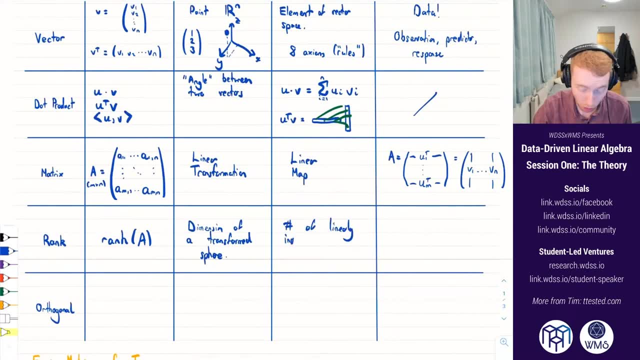 A way we can think about it in terms of algebra Is that it's the number of linearly independent columns Or rows, in fact, Linearly dependent columns Or rows In the matrix. And when we say linearly independent, What we mean by that? 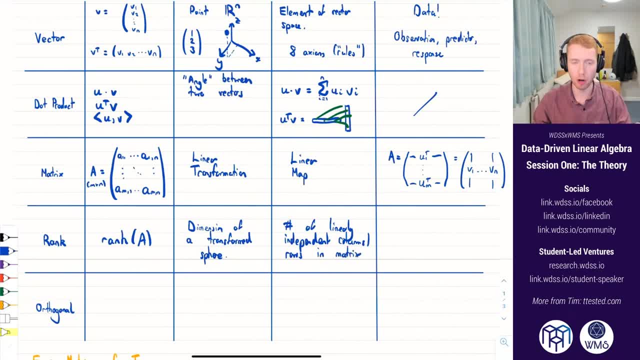 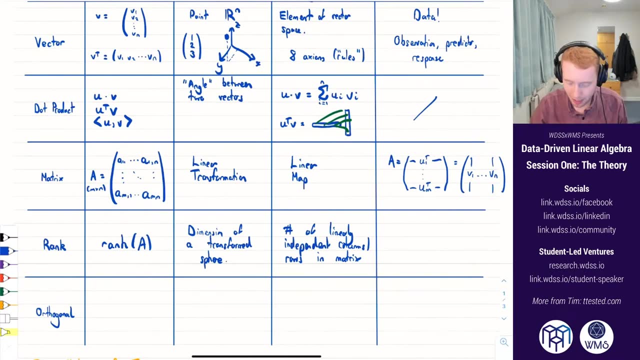 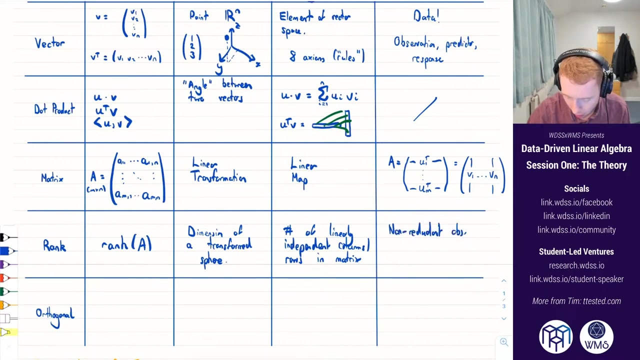 Is that there's no combination of those columns or rows That give us the zero vector. We can't add them up to make zero, But those definitions are quite heavy. The data centric definition is actually quite a nice one, And it comes down to how many non-redundant observations or predictors we have. 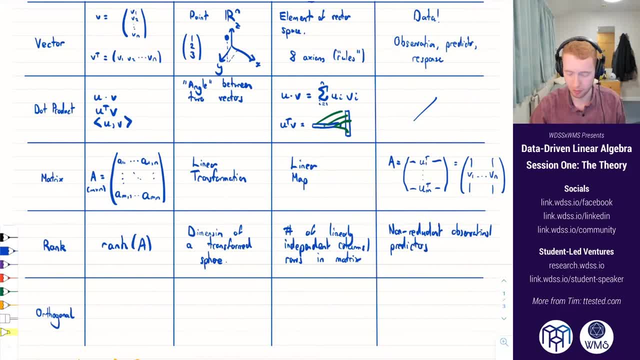 It means the same whether we look at predictors or observations. So, for example, imagine we had a data set like this, Where we had then the values 1 0 0.. 0, 1 0.. And 1 1 0.. 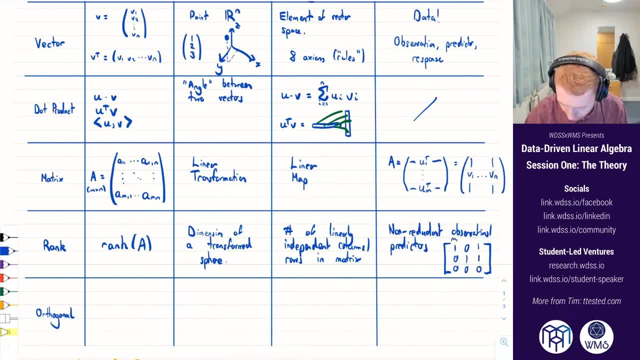 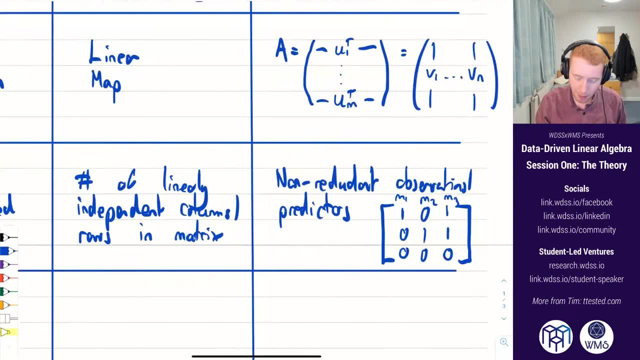 And these are kind of different measurements. So this is measurement 1., Measurement 2. And measurement 3. Well, in this case Measurement 3 is redundant, Because if I know measurement 1 and measurement 2., I can just add those together. 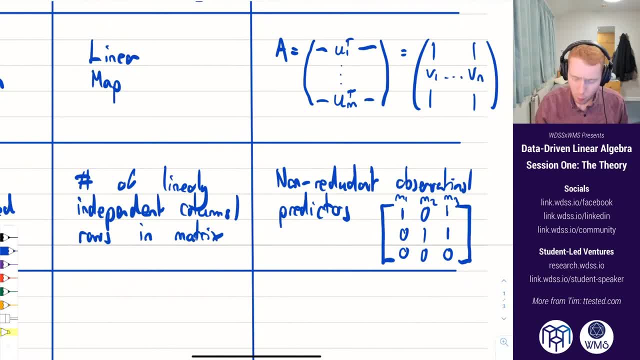 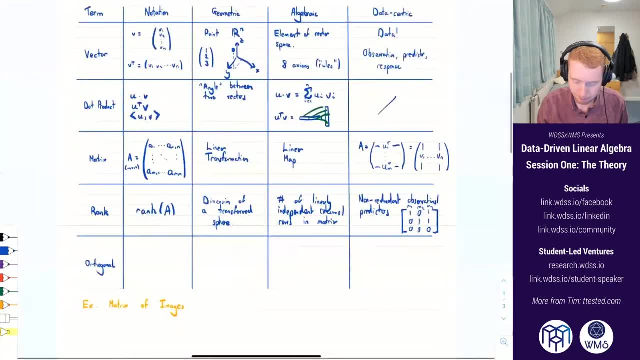 And that gives me measurement 3.. And so in a way, We can think of M3 as being a redundant predictor there, And so the rank of a matrix Is basically how much we can compress this data, Like what is the lowest representation we can have. 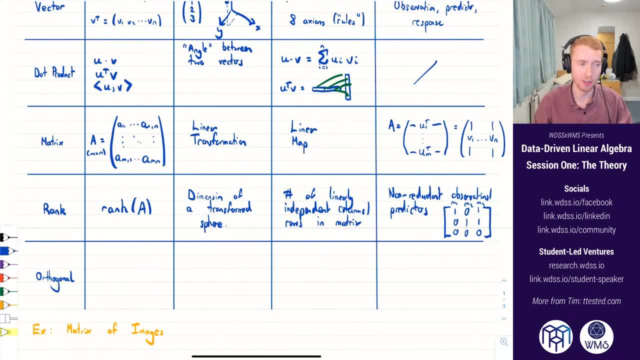 So that none of the predictors or observations Can be given as combinations of the other ones. And then the final thing we're going to look at Is what it means for a matrix to be orthogonal, And there's no real notation for this. 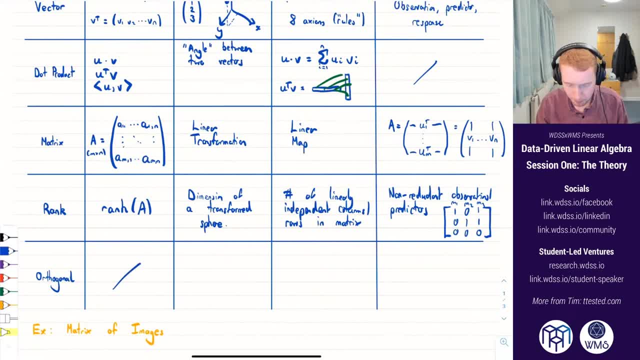 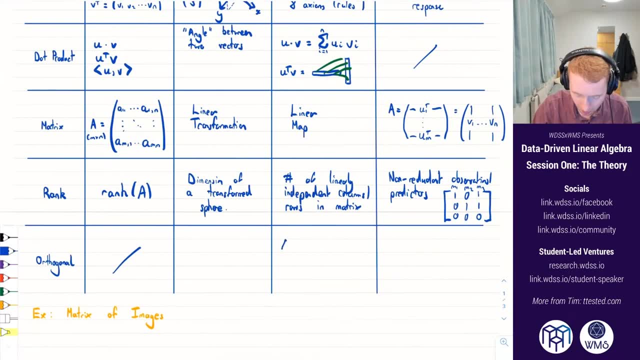 We just write: a matrix is orthogonal, And so let's start with the algebraic definition. So a matrix is orthogonal If, and only if, When we take its transpose times by itself, Or we take itself times by its transpose, We get the identity matrix. 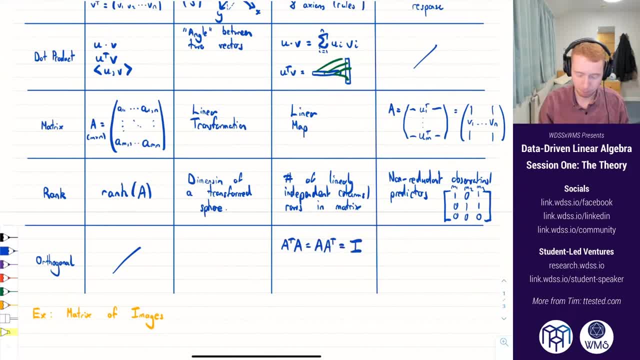 A matrix with just ones down the diagonal Zeros everywhere else. It's worth noting- Let's do this in green- That a must be square for this to happen. It's impossible to have both of these being true If an A is not a square matrix. 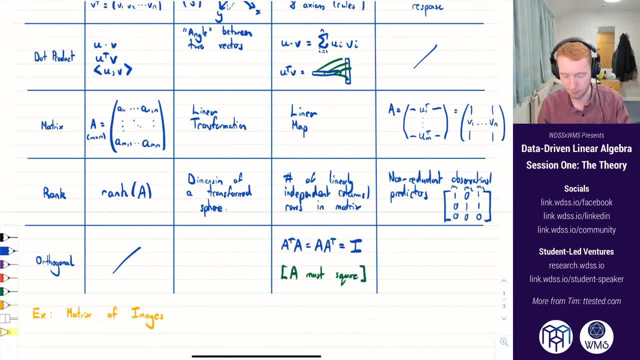 You can have one of them being true, In which case we'd say it's semi or pseudo orthogonal. But that is a heavy definition. It's not intuitive at all. Let's focus on the geometric one, And that is an orthogonal matrix. 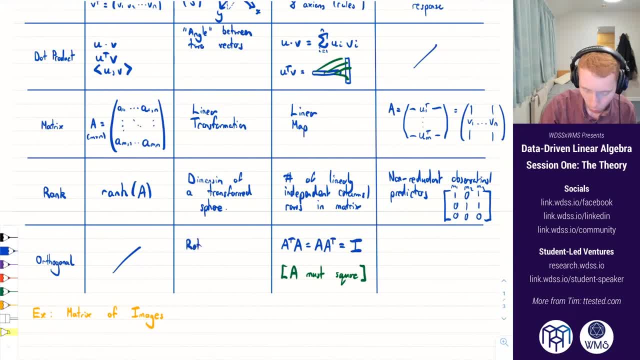 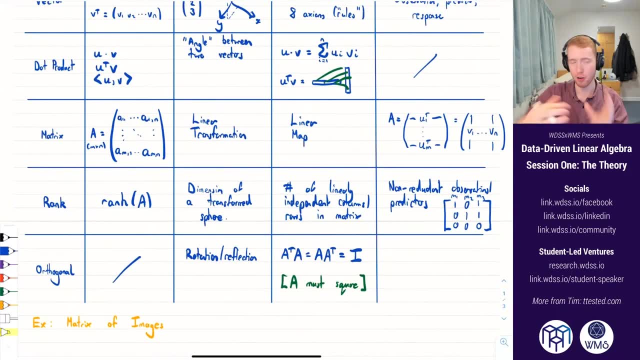 Is either a rotation Or a reflection. So when we talk about these linear transformations, They take our space and transform it in some way. Specifically, the ones that are rotations or reflections, Those are our orthogonal ones, And so, finally, the data centric view of this. 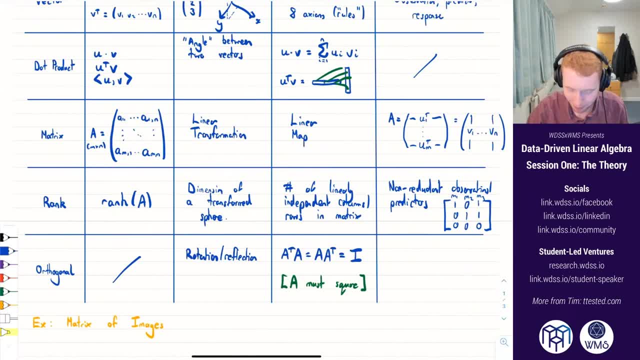 Is that- I'm going to put this in quotes Because it's a bit fluffy- A matrix being orthogonal Or a data set being orthogonal, Because matrices and data sets- We saw that equivalence above- It basically corresponds to There being no correlation. 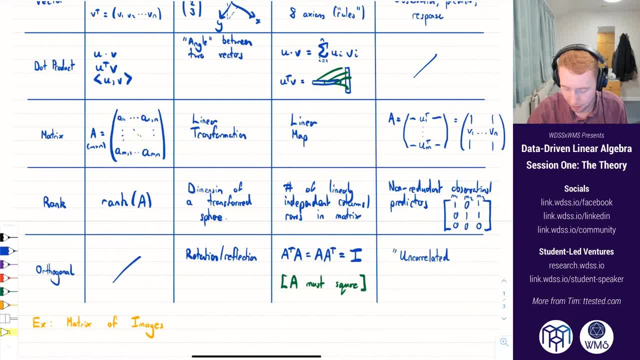 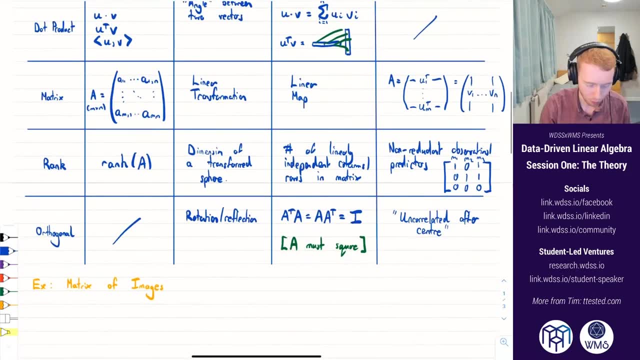 After we center our data. If you're not that familiar with statistics, That's not very helpful, But if you are And want to kind of try to understand What exactly that means, We'll think about the definition of correlation. You'll know that the numerator 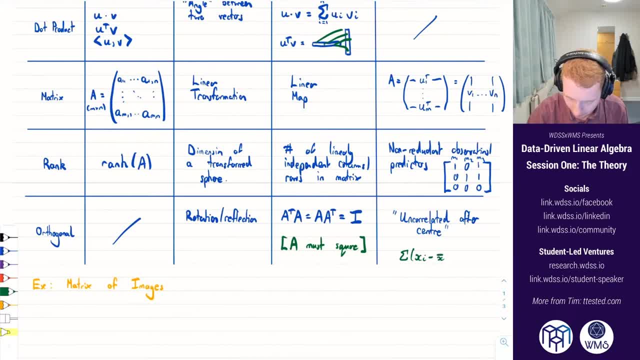 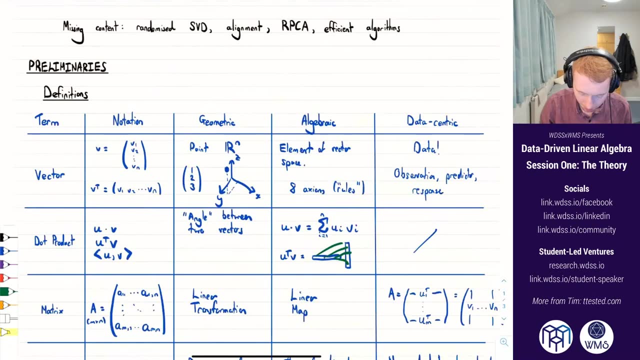 Has this term in it, And if our data is centered, Then these are going to be zero. So then we're left with a sum of x, i, y, i And if you remember Back to above, That corresponded to The dot product here. 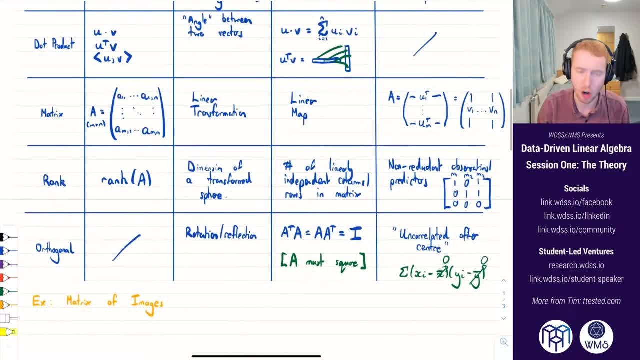 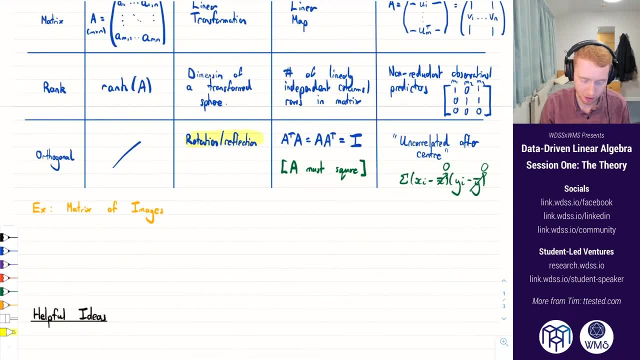 And so if something's orthogonal, Then they're essentially uncorrelated. After we, After we centered them. But this definition here Of reflection and rotation, That makes the most sense. So let's just give an example Of what kind of a data centric view. 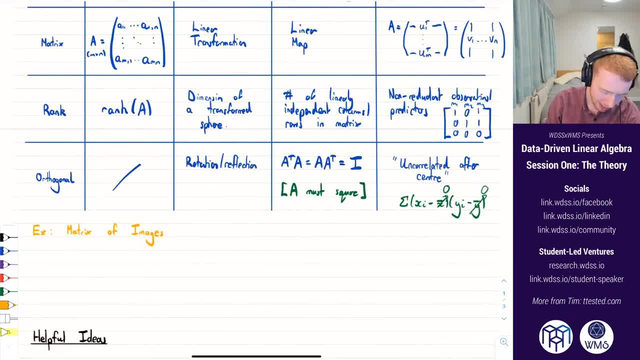 Of a matrix might look like. So let's imagine We have these images here And they're going to be of people's faces. So we have someone smiling here, We have someone Frowning here And someone with a very Long shaped head here. 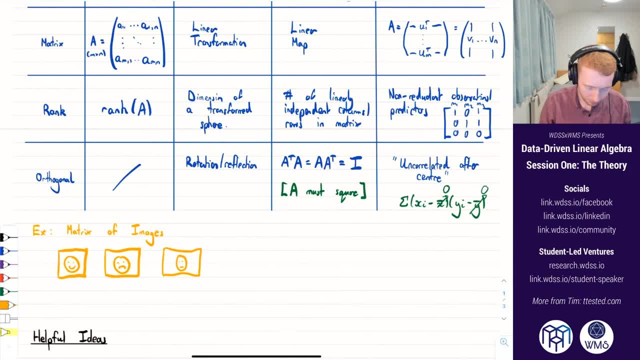 And so we want to represent these As a matrix. Well, the first thing we're going to have to do Is to: Well, actually, yeah, So let's draw our matrix out here, And, if you remember, from This kind of above, 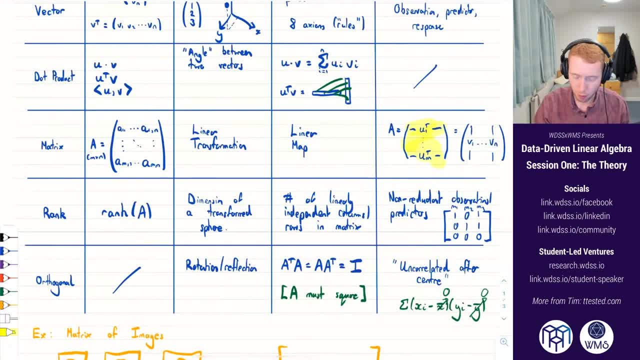 View here That each of these kind of Rows of our matrix Are kind of observations. They are individual Units that we can measure, And so what we're going to want to do, We're going to want to take Our observations here. 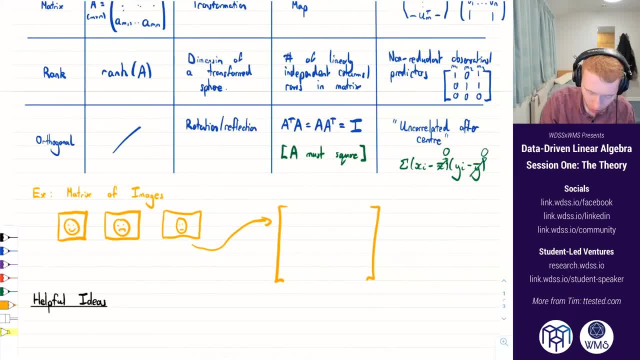 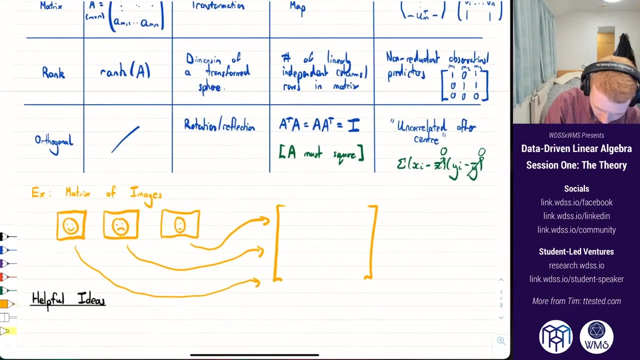 And put those As the rows of our data set. And so to do that, We're going to have to take These images And flatten them down So we can imagine: we turn these, Let's do a proper square here, We turn these. 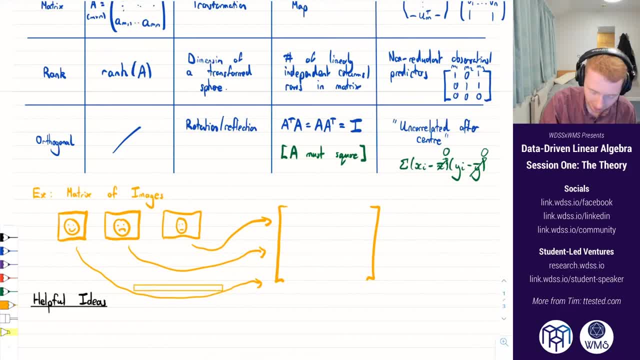 Kind of long images, Sorry, square images here Into these really long and narrow Series of pixels, And those become The columns, sorry, the rows Of our data sets here, And then each of the, Each of the Columns, These correspond to one. 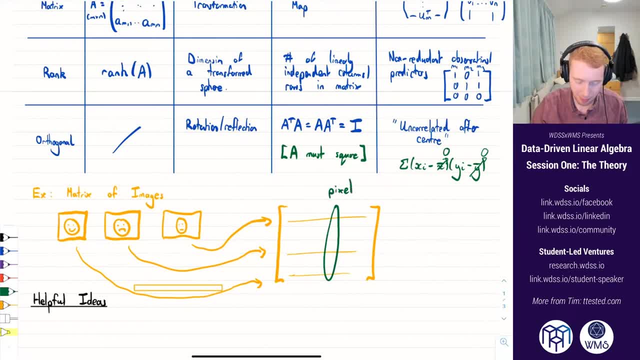 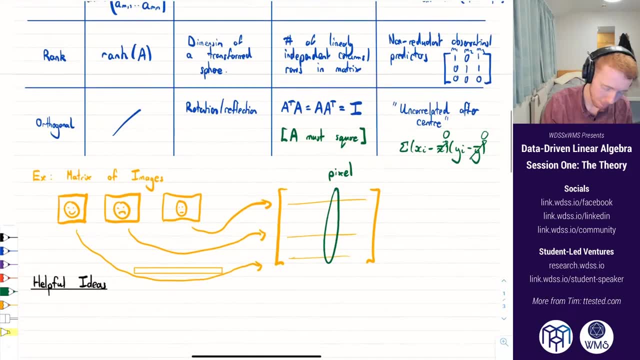 Of the pixels in our image And the value that that pixel takes Over the different images. That's kind of one way of looking at A matrix like that. Okay, so we're now going to have a look at Kind of a helpful idea. 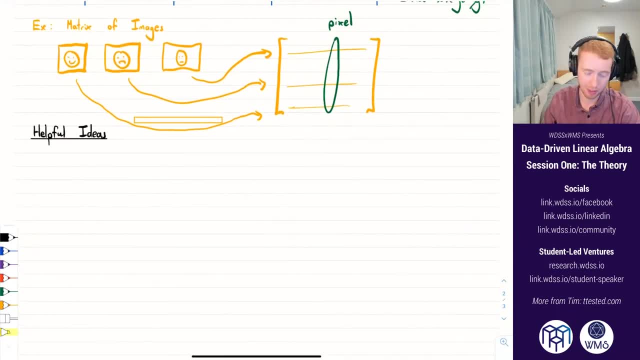 That's going to come in useful When we're thinking about This thing called the singular value decomposition, And it's going to centre around A new way of thinking about matrix multiplication. So you might be familiar with matrix multiplication- Hopefully you are. 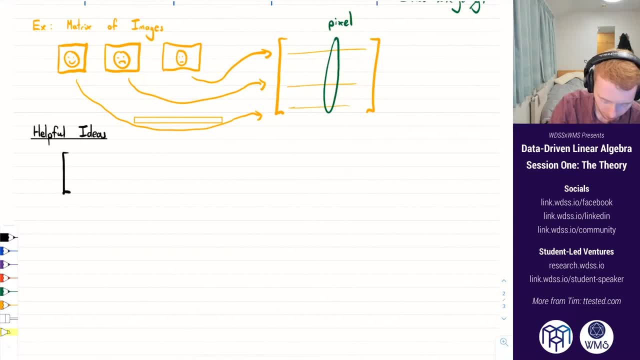 Let's say I have matrices here. We have one, two, Three, four, five, six And matrices one, Two, three, four, And these have dimensions Three by two. These inner dimensions Match. so we're all good, We can take the product. 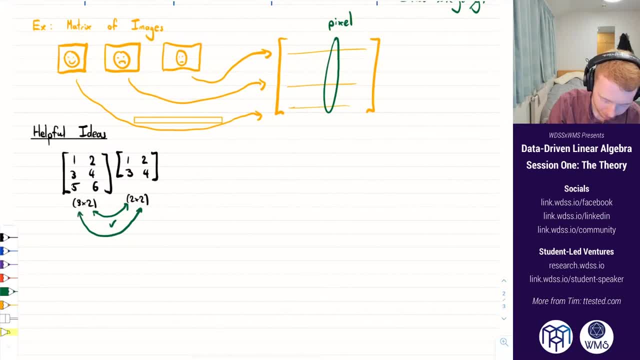 And these outer ones are going to give us The size of the resulting matrix. So here we're going to get a matrix That is three by two, And we do the multiplication By kind of going across The rows and across the columns. 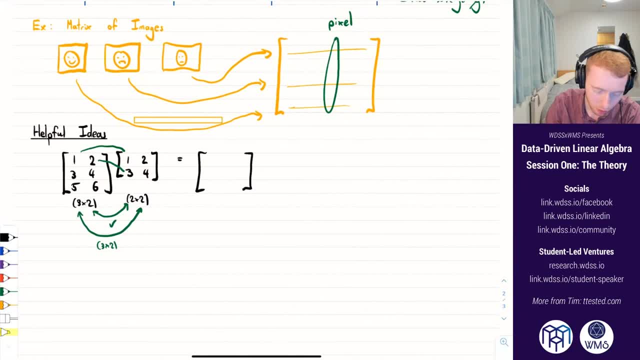 And kind of timesing those together. So one by one is one, And two by three is six, So we get seven there. We have one by two And eight, which is ten, And then we carry on like that We get fifteen. 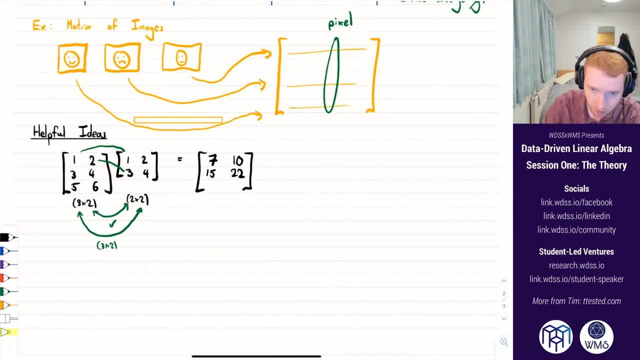 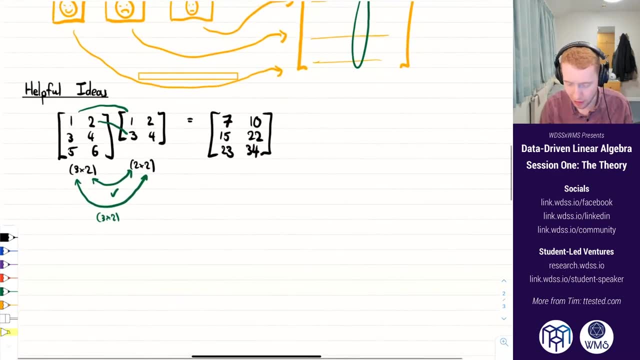 Twenty two, Twenty three And thirty four. So that's how we would do matrix multiplication like that. It's a bit of a faff And there's no real intuition as to what's going on there, So I want to think about a different way of doing. 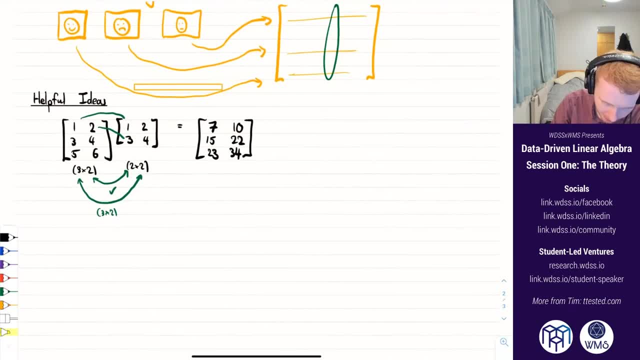 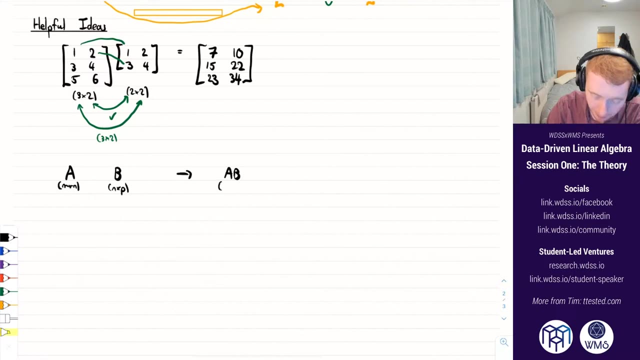 Matrix multiplication. Let's imagine we have matrices A And B And these are M by N And these are M by P matrices, And we want to calculate What the matrix AB, Which is an M by P matrix is, Which is an M by P matrix is. 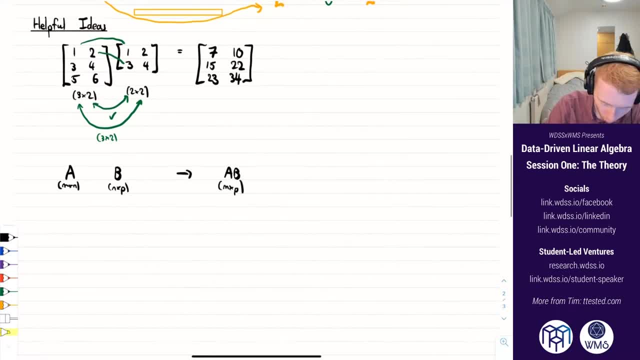 Well, let's think about What the i- jth element, What the i- jth element Of this matrix is going to be. So when we were looking above, We kind of went, you know, If we wanted the i th row And jth column. 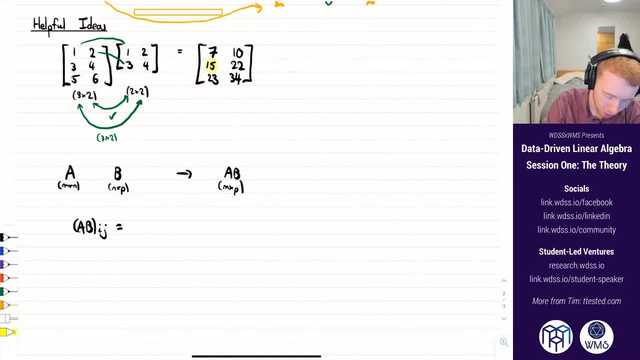 So here it's. i is two and j is one. We went across The i th row And down the jth column in the second one, So, representing this as a sum, We have something like this: So we have the i th column of. 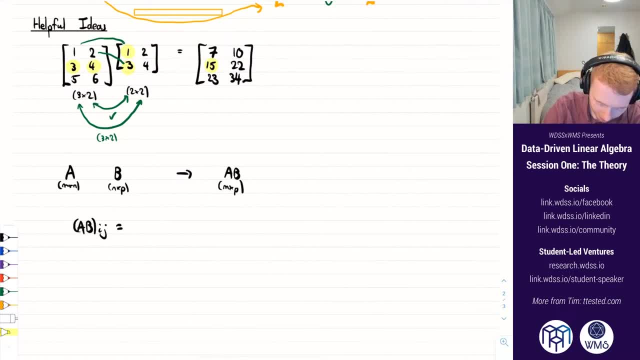 Actually, let's not write it as a sum just yet. So we had something like A, And then we took the i th row, The first column, And the first row in the jth column of B, And we kept adding these together. 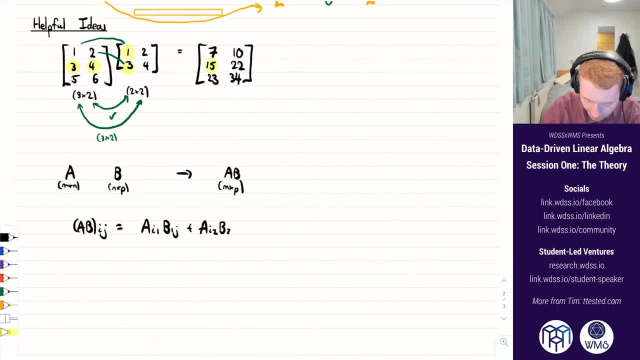 So two, The second one, And we keep carrying that on All over that common axis. So we have n things in it. So then we have n and j Like that, And we can represent this as a sum. So this is the sum of A. 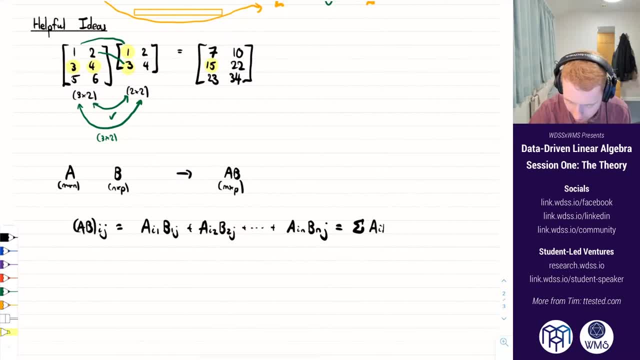 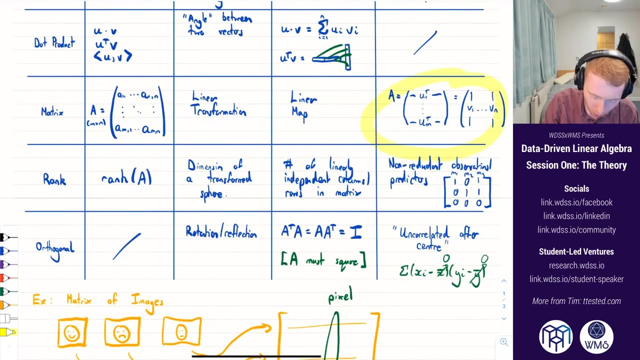 I, k, B, k, j- Going from k is one Up to n, And so now we're going to pause for a second And go back to thinking about matrices Using this sort of Data driven approach, And we're going to write. 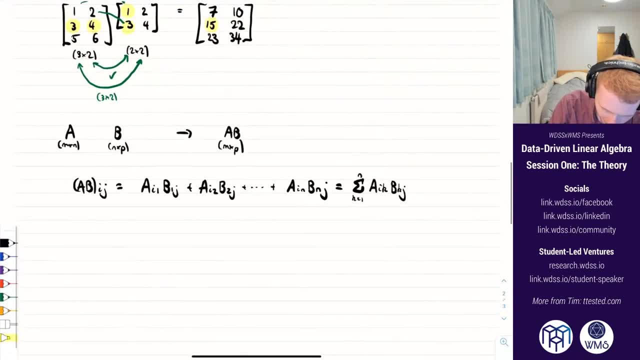 A Like this: We're going to write A As a matrix of rows, So we can have A one transpose, A two transpose All the way down to where there was m rows. So A m transpose, And each of these have n elements in them. 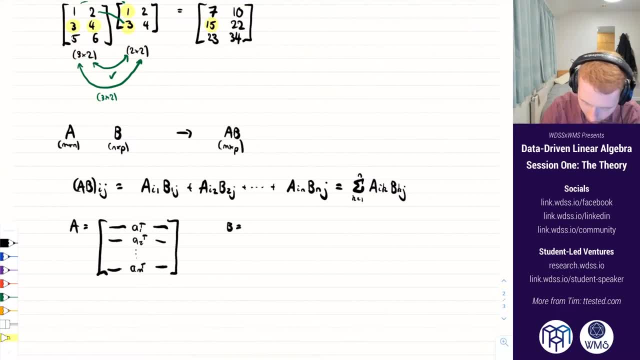 And we're going to write B As a matrix of Of column vectors. So we're going to have B one, B two, All the way up to B p, Because B had P columns. So these are all column vectors here. 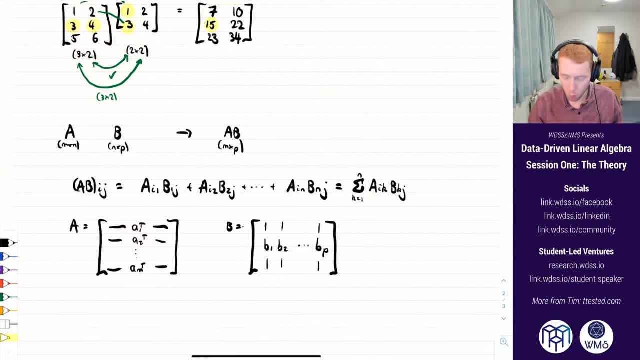 Well, now Let's look at this here We're going through all the elements of A For a fixed i and for a fixed j And all the elements of B And times them all together. Well, that looks an awful lot Like the dot product. 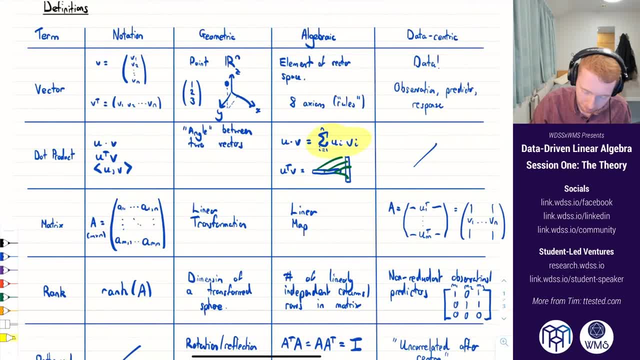 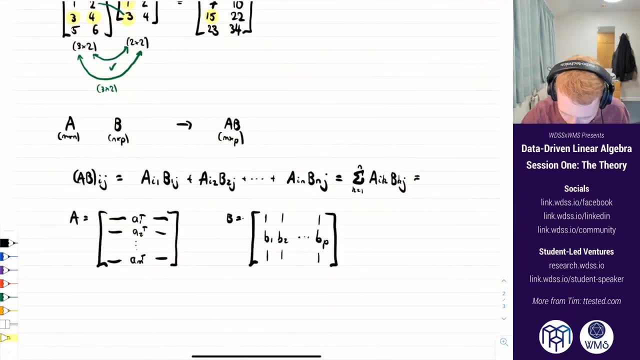 That we had before. In fact it is the dot product that we had earlier, And so we can think of This matrix multiplication As The dot product between A, i And B, j, And so really all the matrix is Sorry, all matrix multiplication is. 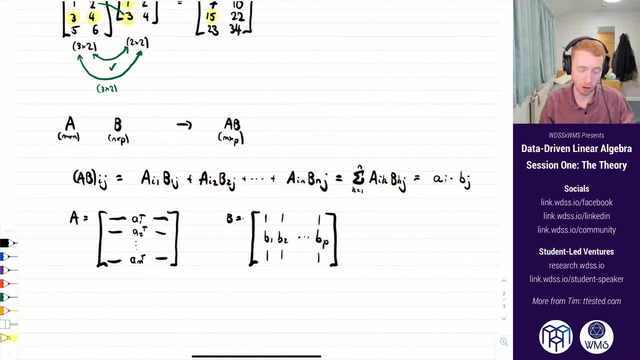 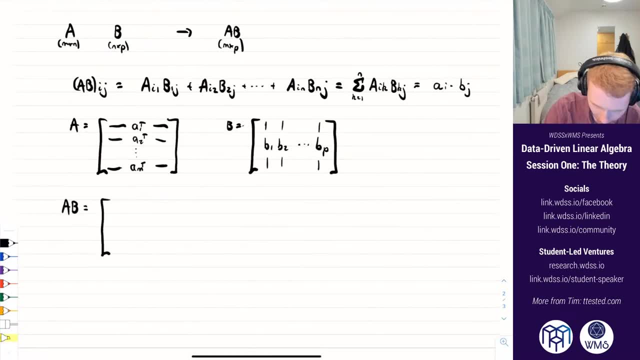 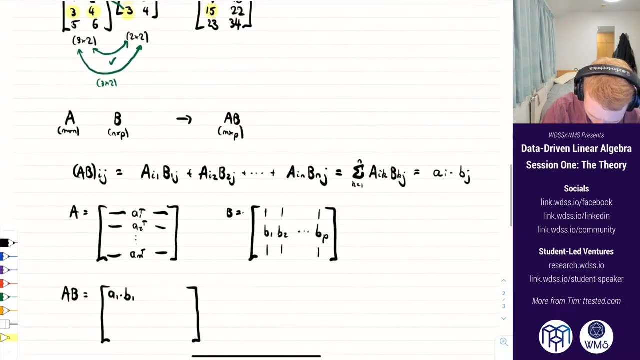 Is giving you a matrix Of dot products, And so we could write A- b As something Like this: So A one B one, Then we're going to have A one B p, Then A m B one. 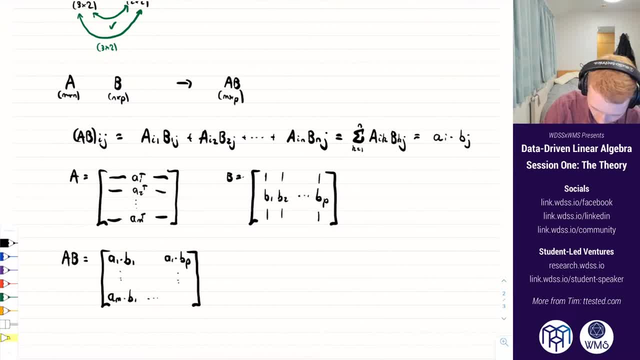 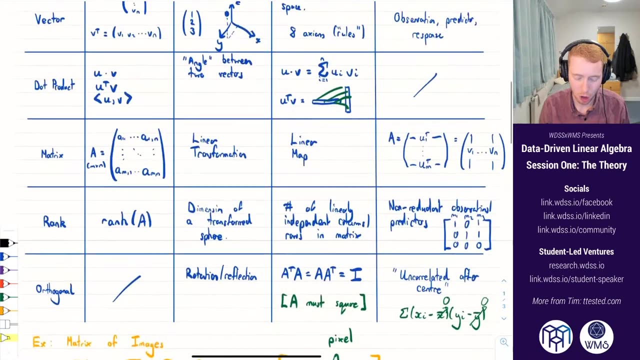 All the way to: To A, m, B, p. So another way of thinking of matrix multiplication Is as building this matrix Of dot products And when we start to think about what a dot product means Geometrically Either as these angles 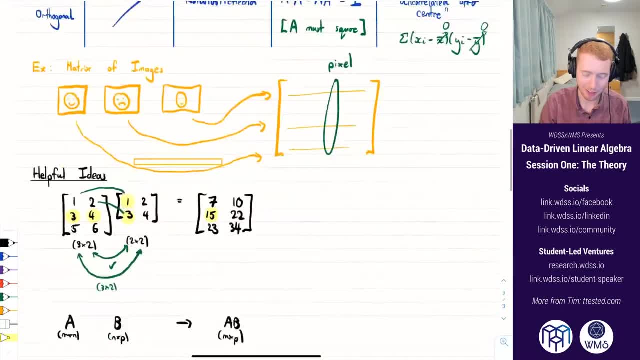 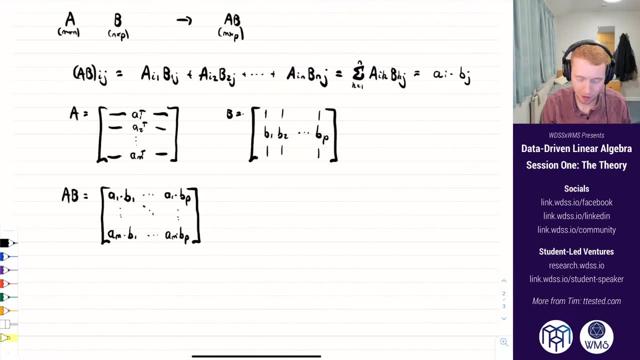 Or as another way of thinking of those is projections. This starts to take on some very interesting meaning As it's the matrix Of the angles Between These observations and these kind of. You can think of these as predictors Or ways of mixing those observations together. 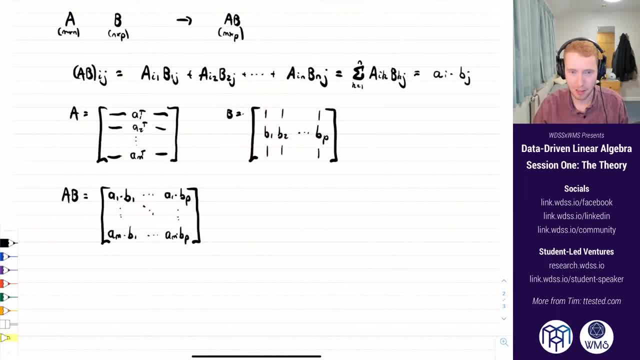 And it starts to take on quite an interesting meaning, And so I'm also going to give another result, And I don't have time to prove it, But if you think about it for a bit, It should Make sense of what's happening. 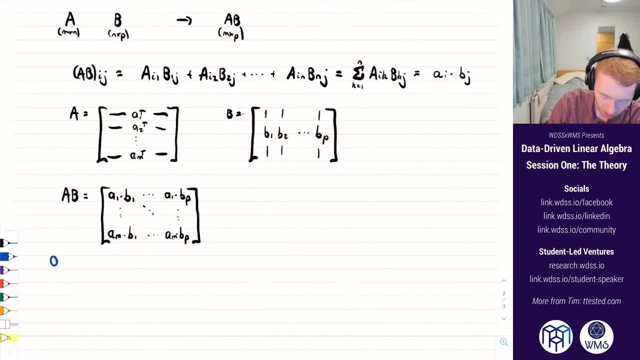 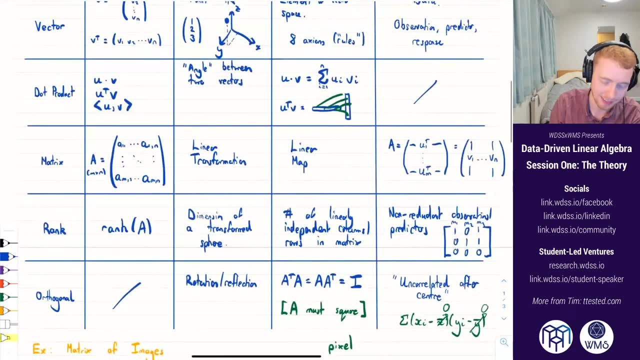 So first we're going to have to define this thing called an out product, And so When we talk about the dot product Here, Another word for a dot product Is an inner product And it's out product is kind of the opposite. 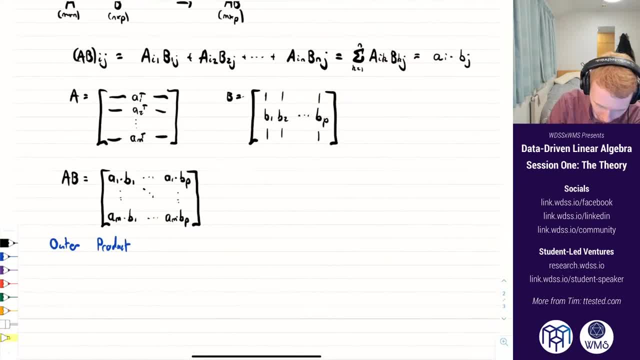 And if we have, If we have vectors U and v, So u is u1. All the way down to un And v Is v1. Down to vn. And what the out product Of these, These two vectors, is. 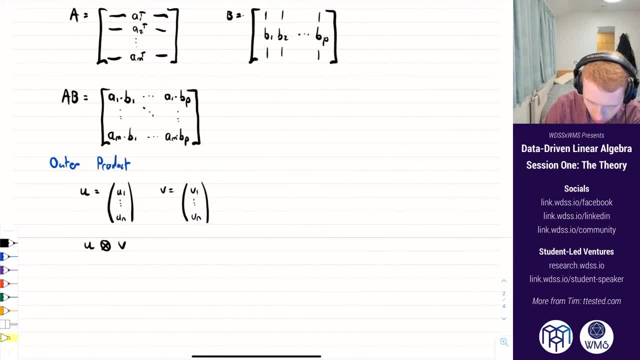 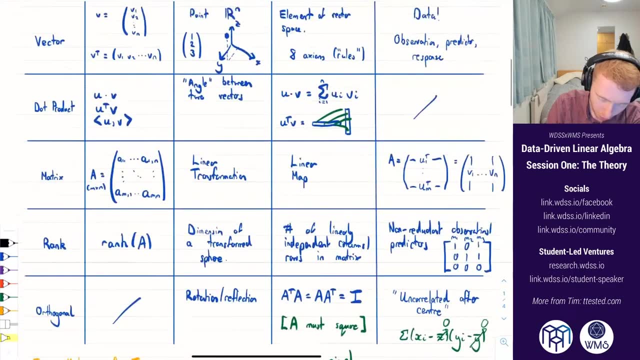 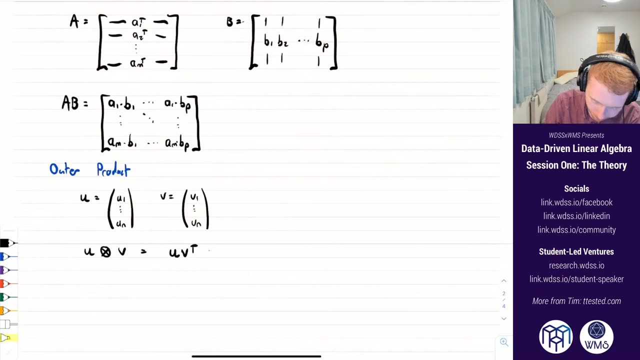 This cross symbol With a circle. We could also write that as u V transpose. Now, don't confuse this with The u transpose v we had before. These are opposite ideas. This is a u v transpose. It's going to be. 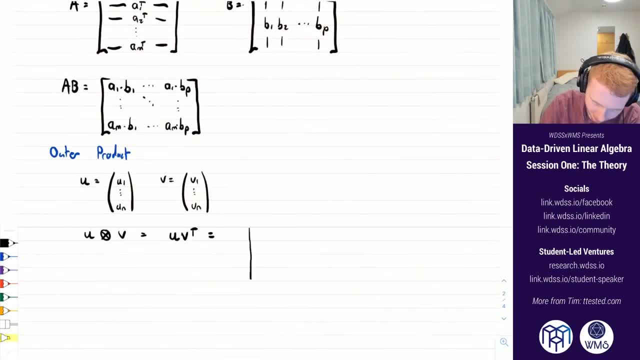 Well, u is this kind of long vector here, And v is this kind of This. Well, v transpose, is this kind of Wide vector going across here, And so this is going to give us A matrix that looks something Like this: 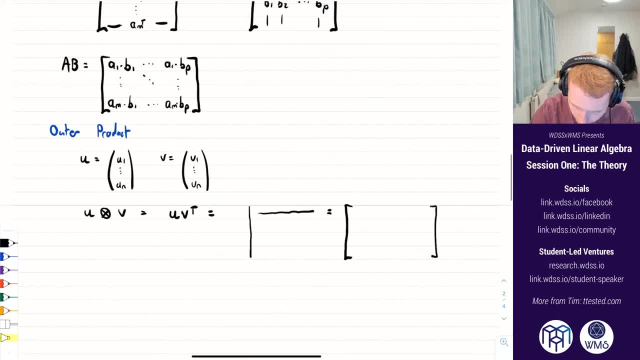 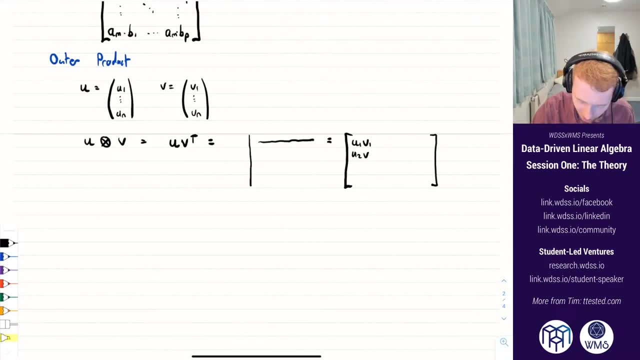 So we're going to have the first term. We're going to take the first element of u, So u1 times by v1.. Then for this one it's going to be U2 times v1 again. It's still in this column here. 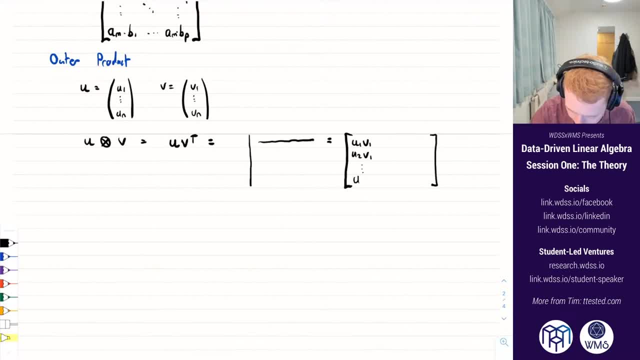 Then we carry that down to Un v1. And then we can go across And we'll end up with Still u1, but now vn, U2, vn, All the way down to vn, vn. So, whereas an inner product 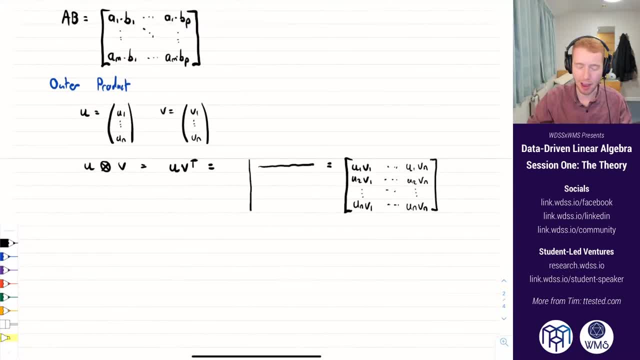 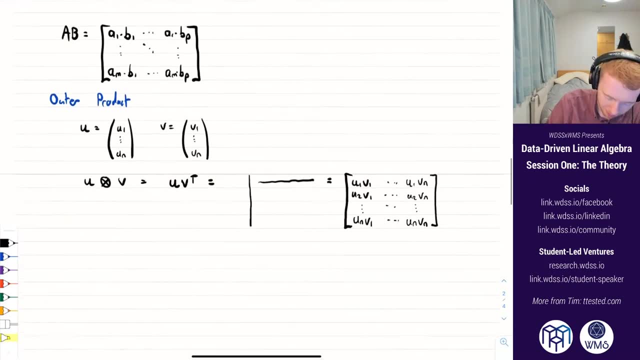 Kind of took us down to a single value. This blows us up into a whole matrix Of every possible combination Of those two elements, And so this leads us to a result Which is another way of thinking about A matrix product, And so 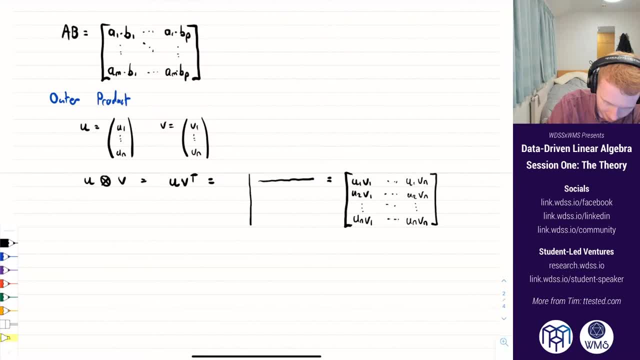 This is actually going to be The representation of b Times a. Actually, no, They don't match up. Let's define two new matrices. So c Is going to actually be Columns now, So c1. C2.. All the way to c. 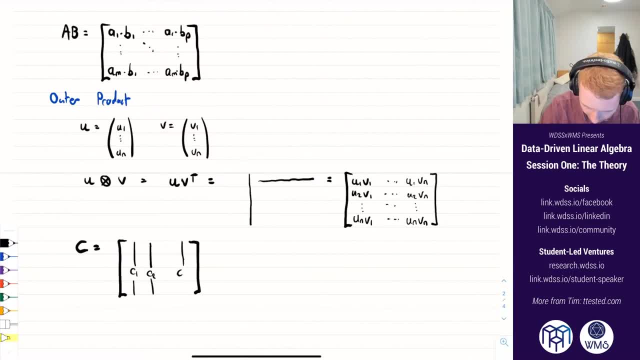 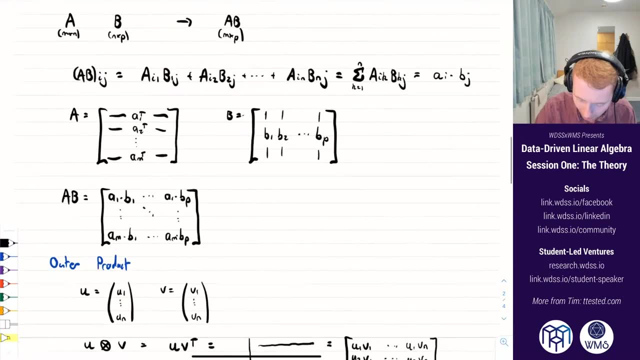 We're going to need to have The same number for these. Let's call it cn, And then d is going to be something like Row vectors now. So before we had columns, then rows, Now we're going to have So columns and then 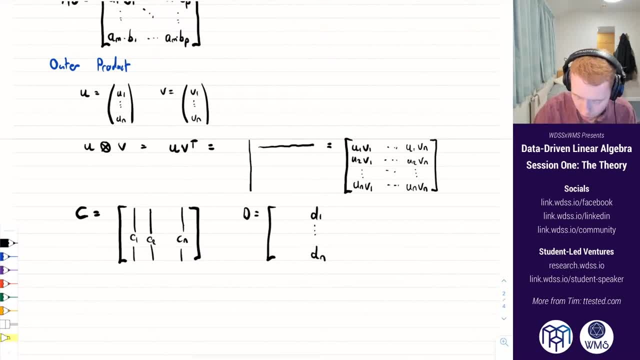 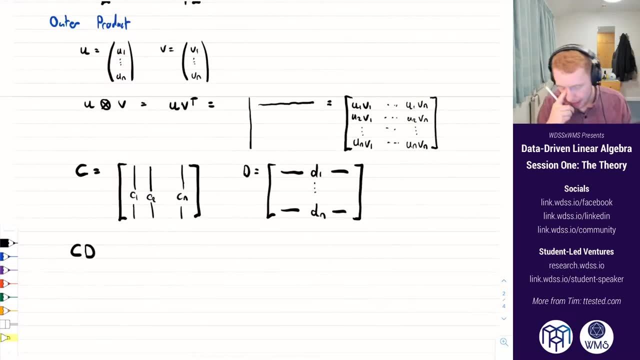 And then rows. So we have something Like this: And then another way of representing Cd Is as a combination Of these outer products, So we can actually write The product cd As the outer product between C1. And. 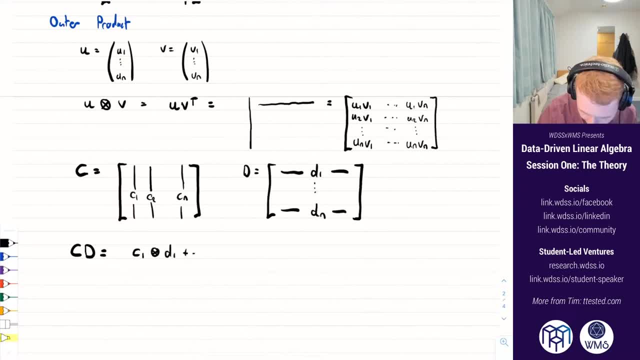 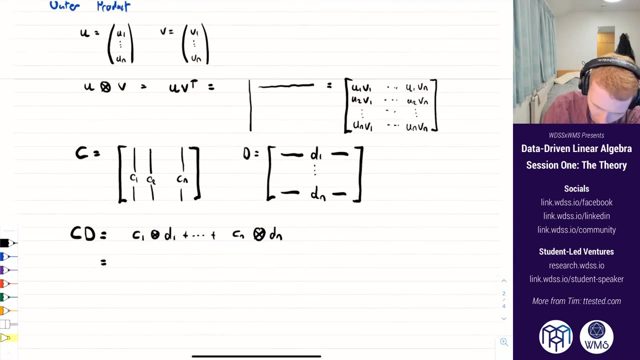 D1.. All the way up to Cn. Sorry, That's the wrong way around Between cn And dn, And so writing that in this kind of, In its vector form, It's c1.. D1 transpose: All the way up to. 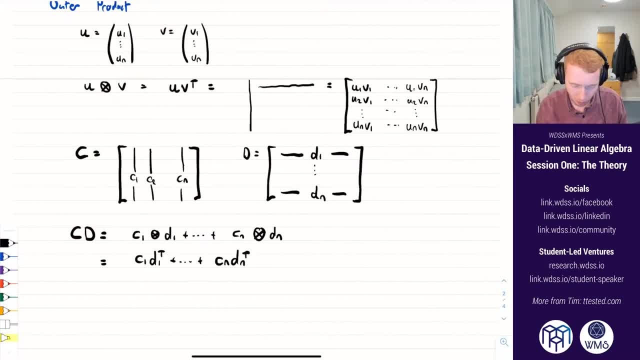 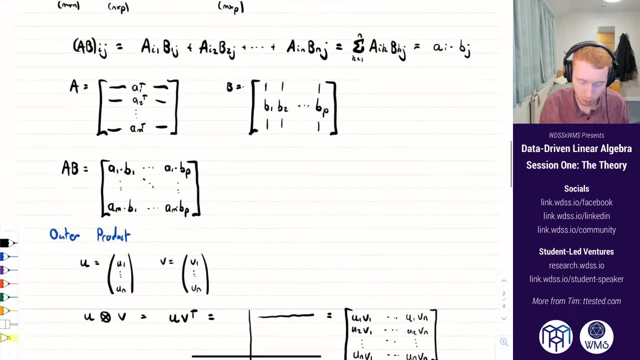 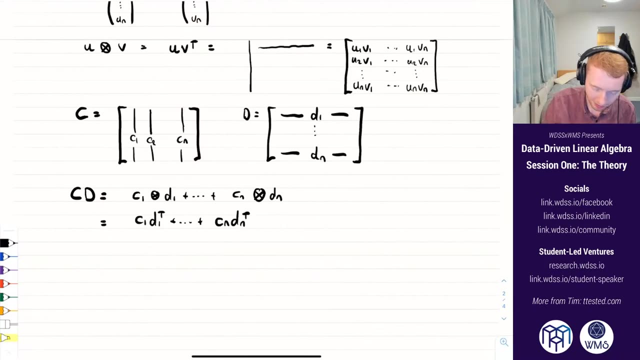 Cn, Dn transpose. So that might seem a bit heavy And I encourage people who are kind of Into their mathematics To kind of sum above But just view in a different axis. Think about why that is true. Essentially what we're saying here. 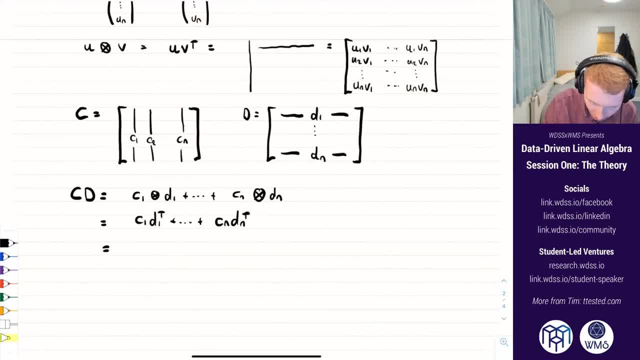 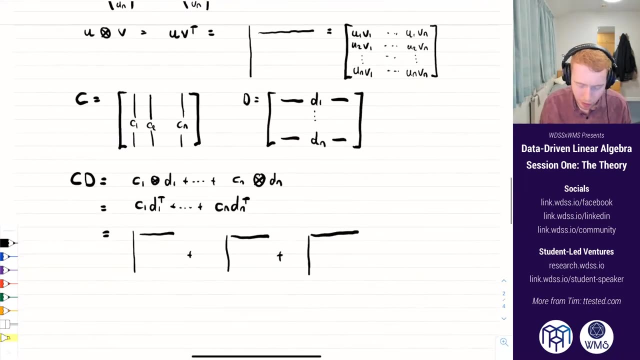 Is that we can write cd As a combination Of these Products Of kind of Single vectors, Single column vectors And single row vectors. It's quite a beautiful idea. And then we can go one step further. And that is what, if we want to compute. 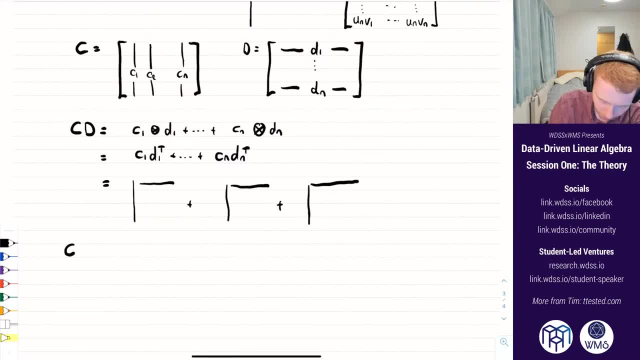 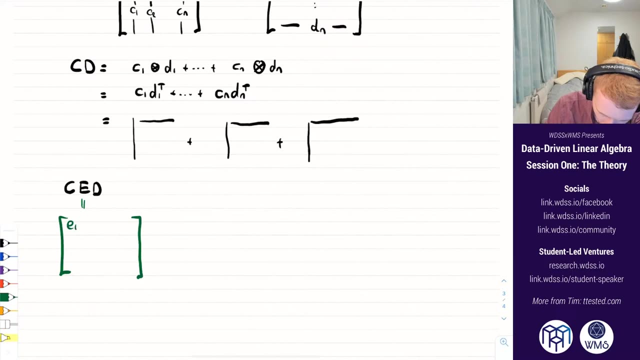 C. And what am I going to call this? I guess let's call it Ed, Where e Is a diagonal matrix, So something like this, And it has elements E1., E2. All the way down to en. 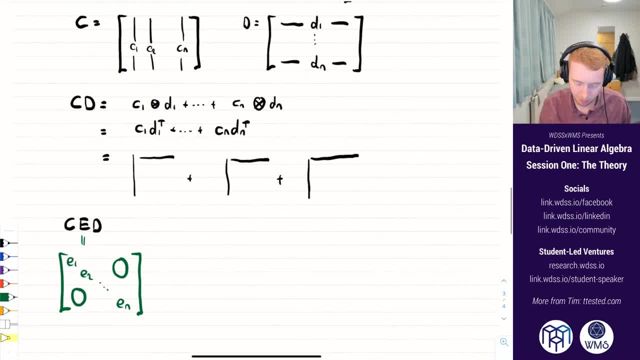 And then everything else is zeros. If we're computing something like that- Actually it has a very similar representation to this One above By those diagonalized elements- Let's do, Let's do this with e3. And then dot, dot, dot. 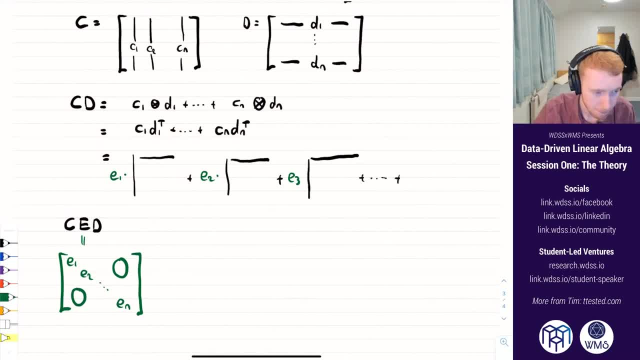 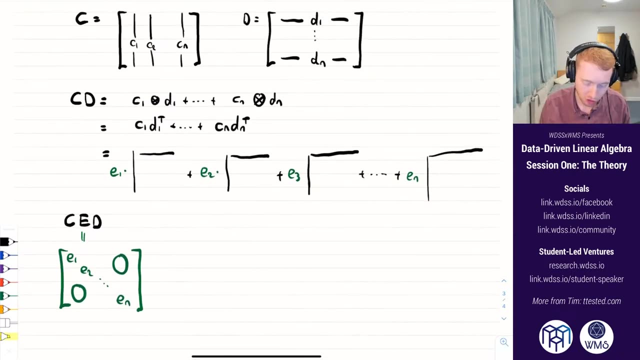 All the way up to En And then this one Here, And so this is going to come really handy When we start talking about the singular value decomposition, Because we can basically Take any matrix multiplication Or kind of a triple matrix multiplication. 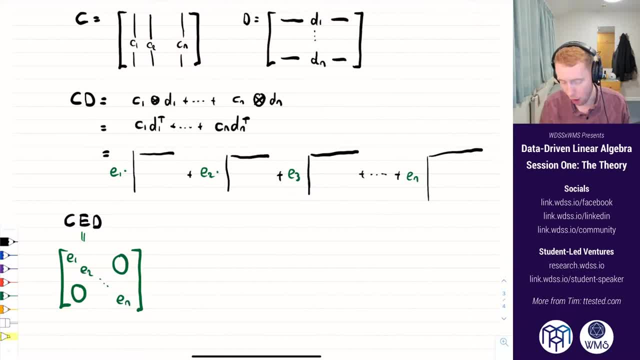 With a diagonal in the middle, And think of it as a sum Of these kind of Low level representations And, more importantly, Each of these matrices, The products we get from here. These are going to have a rank of one, And the reason is that you know, 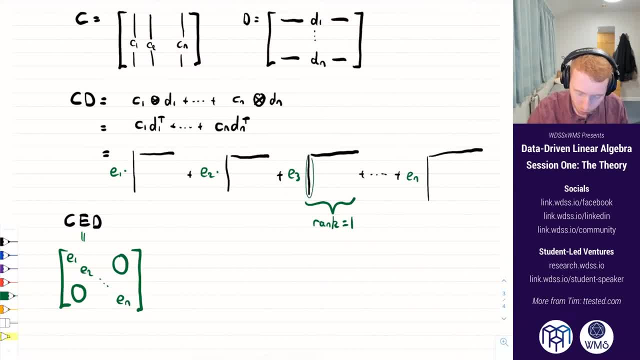 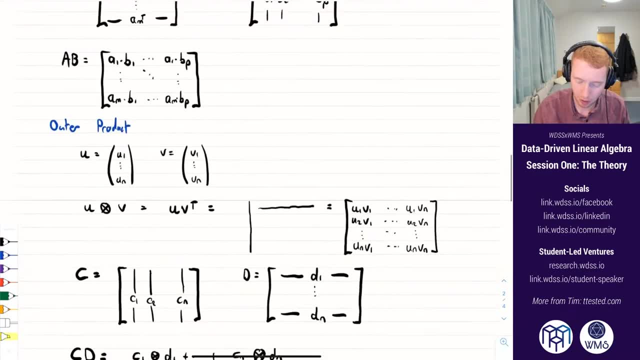 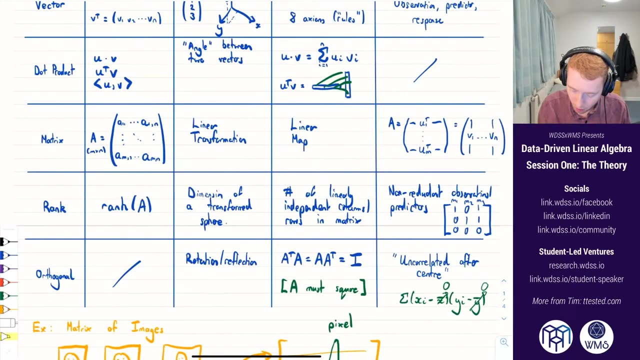 What we're kind of doing here: We're taking a single column And then we're multiplying it by each of these These values here, And so, thinking about the data centric interpretation Of, Of, Of being, Of rank, Let's not delete that. 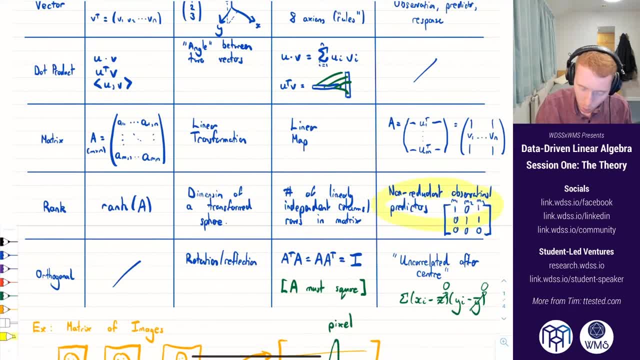 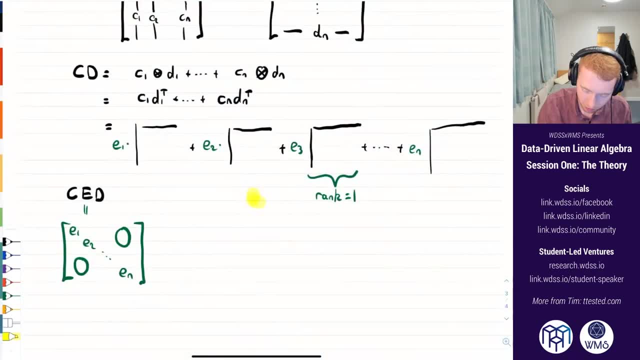 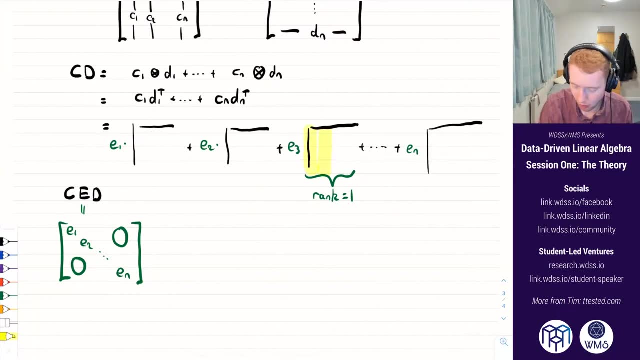 When we're talking about. you know How redundant is our data. We can see here that our data Is just kind of duplications. It's just duplications Of this, Of this same vector Being repeated again and again. So this has it as a rank one. 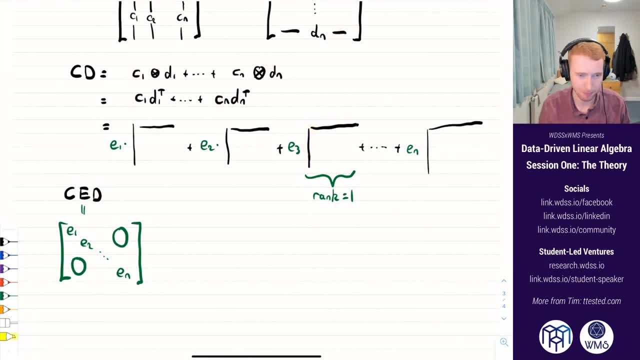 So we can write this matrix as a combination Of rank one matrices. Okay, so Maybe some kind of heavy preliminaries now To kind of bulk of today's session, Which should be a bit lighter than this introduction, But hopefully It was interesting to see these kind of data centric views. 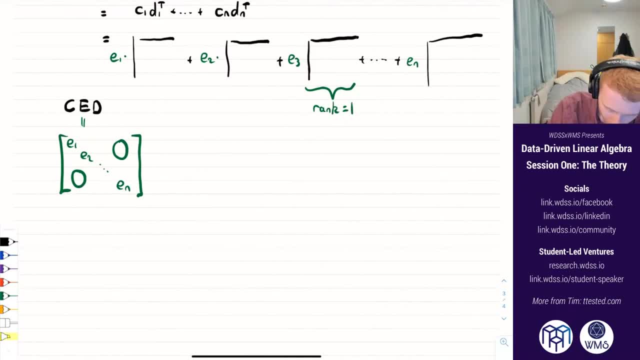 On how we can do linear algebra. So we're now going to talk about These things called decompositions, Decompositions. So what is a matrix decomposition? That's not a straight line. There we go, okay. So a matrix decomposition Is kind of the matrix generalization. 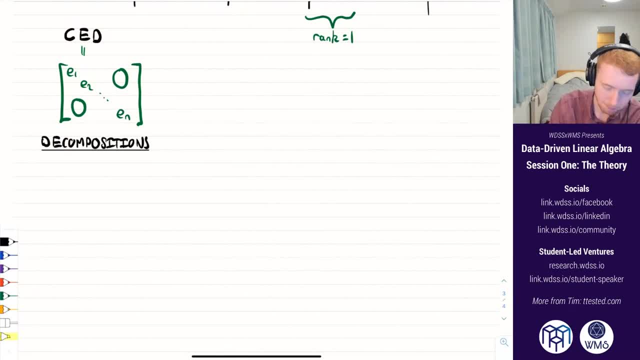 Of factorization. So imagine we had Some polynomial X squared minus x minus six. Well, we can write that As x minus three, And then x plus two, And so this is essentially. They mean the same thing, But this representation on the right. 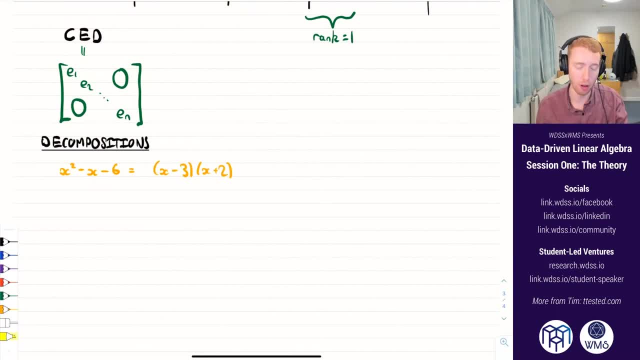 Is much more useful Because it's going to tell us, for example, Where the roots of the polynomial is Zero, when x is three Or when x is minus two. So basically, all a decomposition is- This is a very loose definition, So a decomposition? 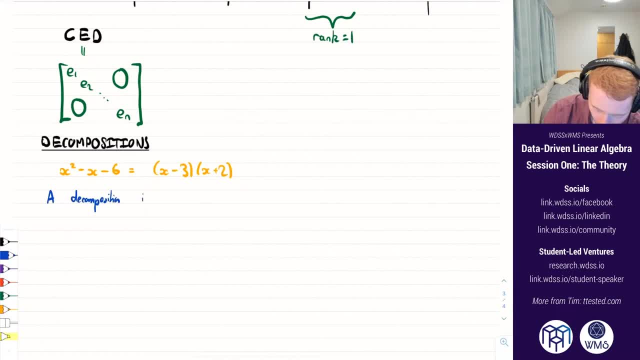 Is A factorization Of a matrix Into products. So basically we take a matrix And we write it as a product Of other matrices And hopefully these products Will come with some interesting properties That will help us do more interesting things. 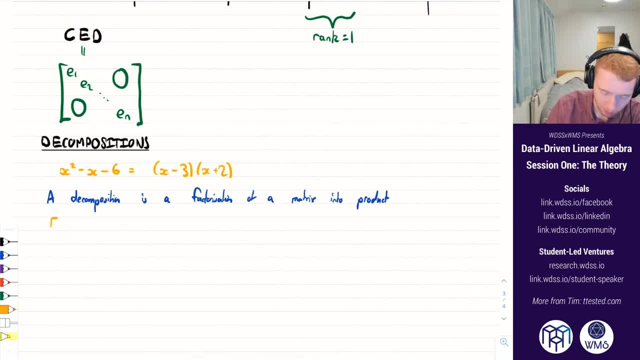 So an example Of a decomposition That you might have seen before Is the eigen decomposition. This is also known As the spectral decomposition, Or simply as diagonalizing a matrix, And so this Comes down to Writing a matrix A. 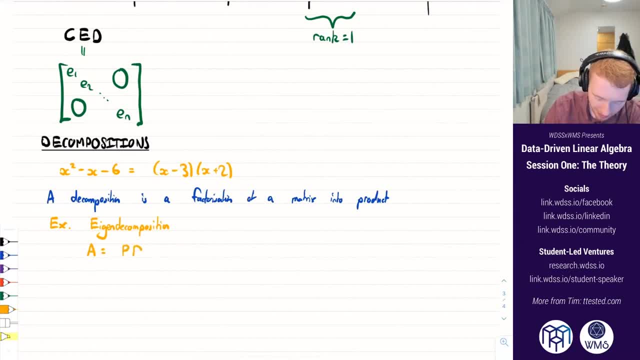 As some matrix P Times, a diagonal matrix, That matrix P. So here this is diagonal And P is invertible, Obviously has to be, Or we couldn't invert it, And so This is a very useful definition. Why is it useful? 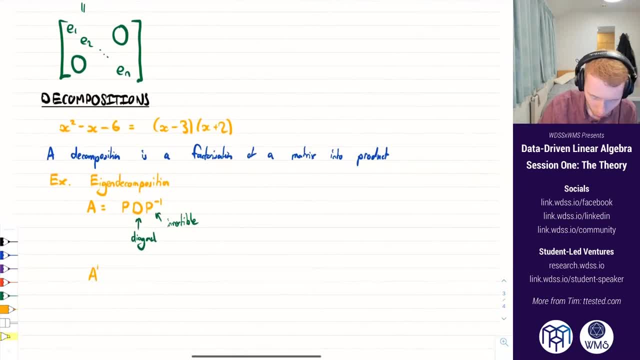 Well, if I want to take A to the power of 100. Well, I can write this as P D P inverse To the power of 100.. Then I can write this out As P D P inverse. P D P inverse. 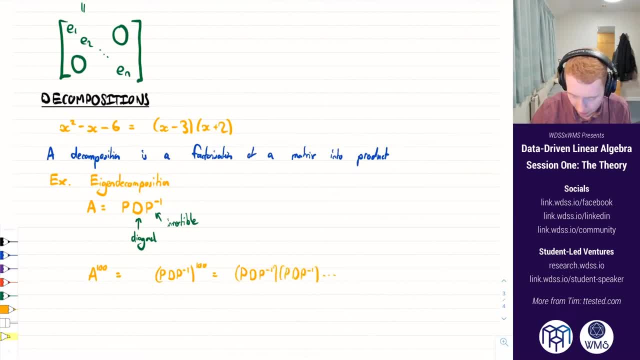 Keep repeating this 100 times P D, P inverse, And then all of these P inverses, P's Will cancel out, Leaving us with just P D to the 100.. P inverse And calculating the power of a diagonal matrix is very easy. 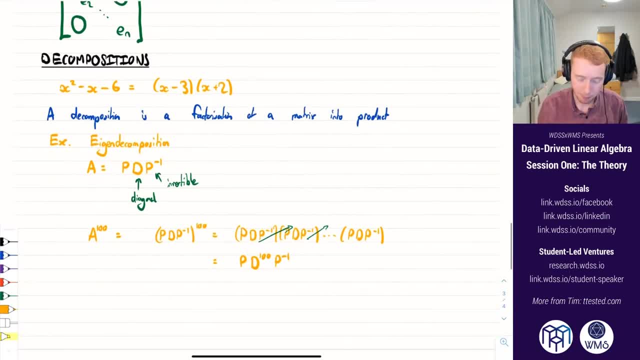 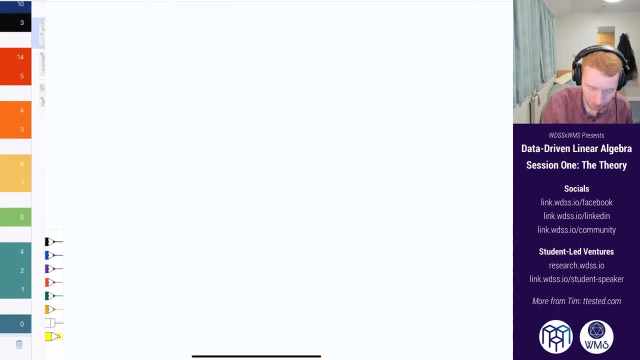 You just take the powers of the diagonal itself. So this is a very useful property That we can get By having our matrix represented In this format. Pressing the wrong button there, Okay, So what are the problems with that, though? 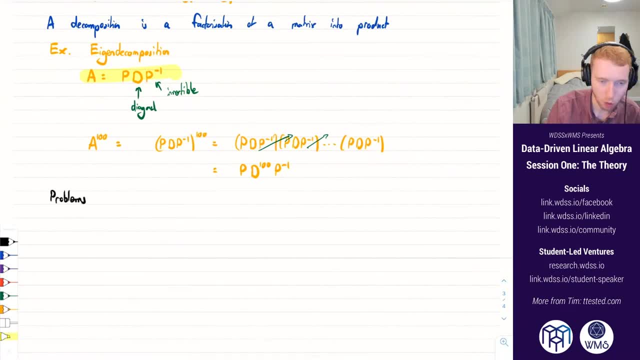 Okay, Well, the biggest problem: It doesn't always exist. So this decomposition here, A into P, D, P, inverse, Doesn't always exist. In fact It only makes sense For square matrices. So these two factors Are very limiting. 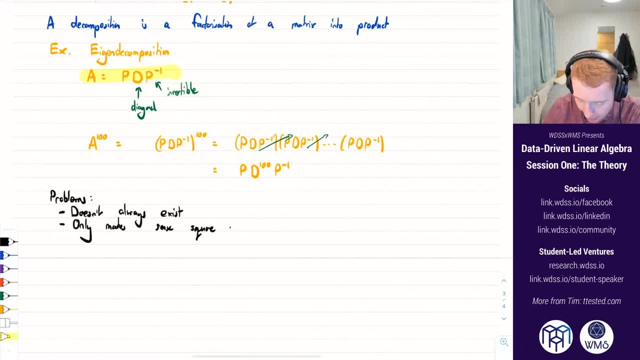 And, even more Annoyingly, The actual check to see Whether it does exist Is just as complicated As actually computing it. And so if we had a really massive matrix And we tried to compute it And then figured out that actually 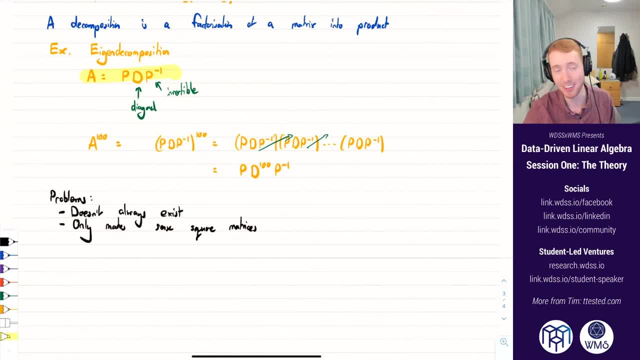 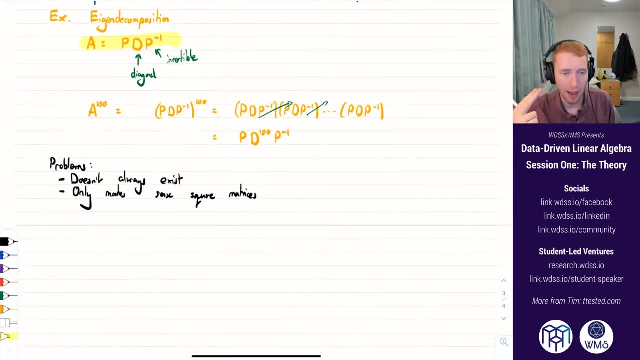 There isn't a solution. It would take us just as long to do that As it would actually compute it in the first place If it did exist. What we would really like Is a more flexible And general decomposition That works for all matrices. 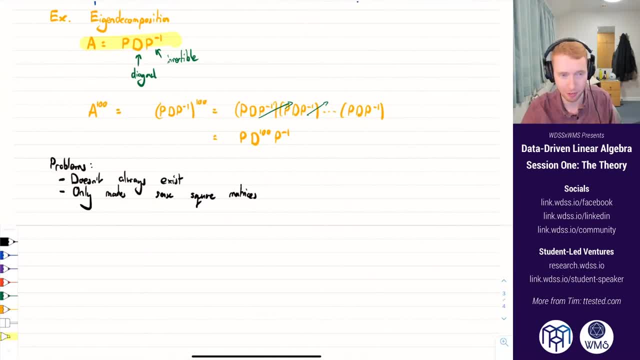 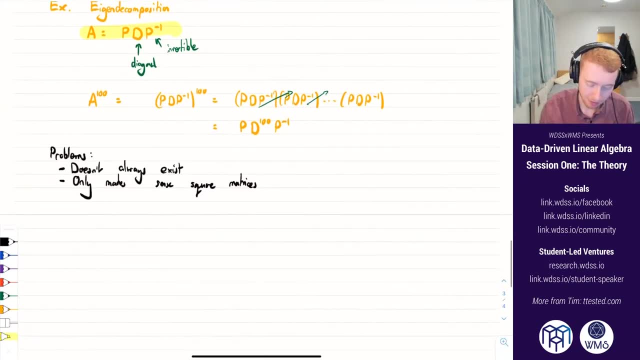 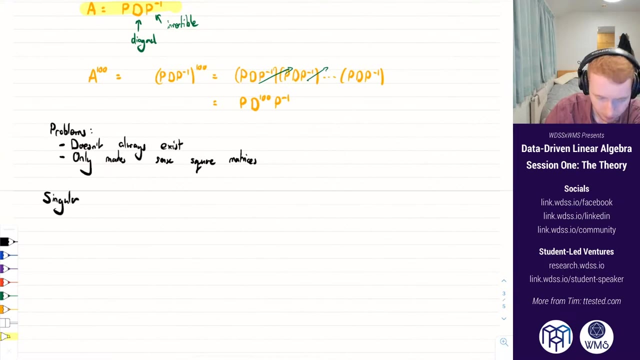 Yeah, Just that We want a decomposition that works for every single matrix, And so we want to step beyond the eigen decomposition That we might have seen before Into this thing called The singular value decomposition, And we, Let's write that in full. 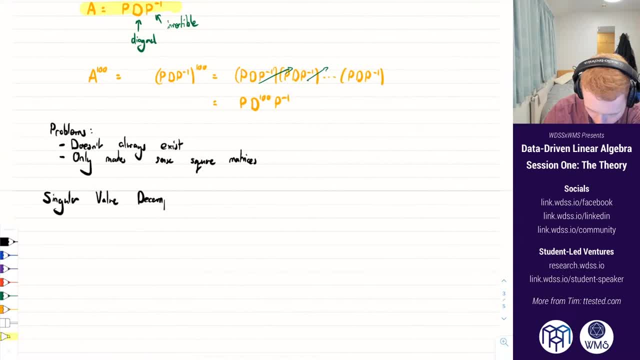 So singular value decomposition, Or the SVD. So I'm noticing, Looking at the time now, That we probably are going to overrun a bit, So apologies for that. We're going to get to the singular value decomposition And then take a short break. 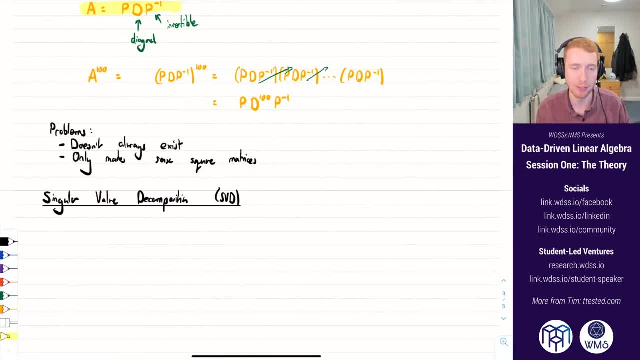 And hopefully we'll only be about maybe 15 minutes overrunning, But obviously the recording will be up later If you want to watch the end of it, If you have to go. So for the singular value decomposition, We're going to have a matrix X. 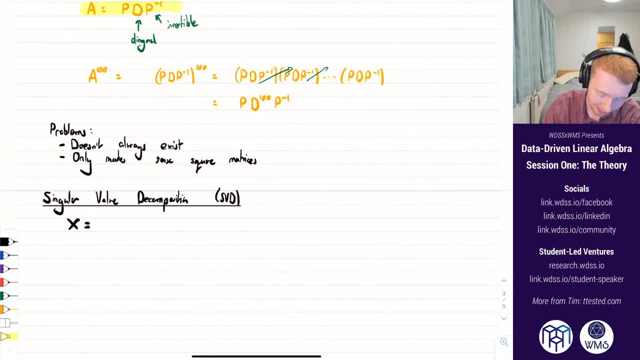 And so We're going to represent X Using Columns Of our observations, So we can write X as X1, X2.. All the way up To Xn, Where we have n observations And each of these are our columns. 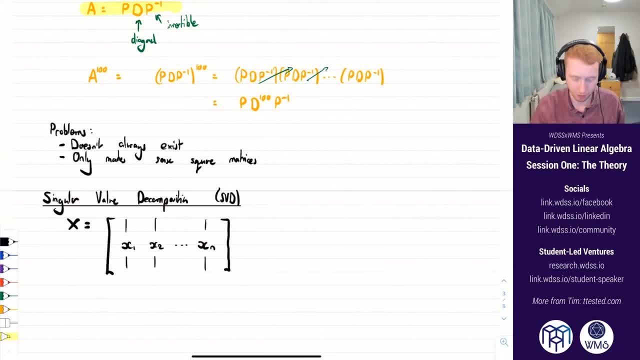 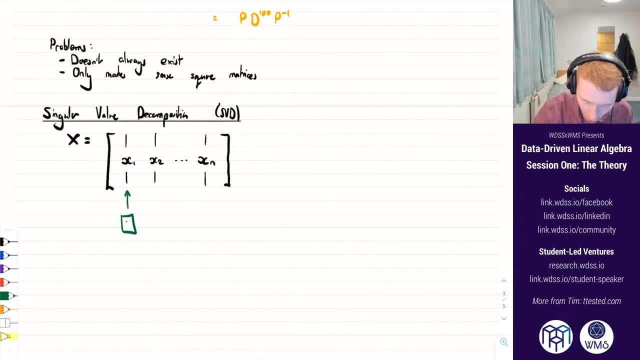 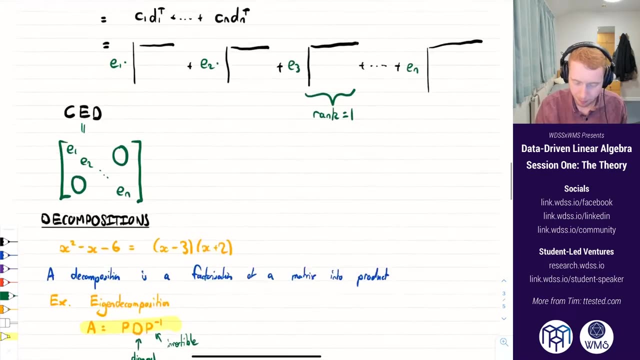 Sorry, Each of these are our observations. So imagine, in the image case we saw before, This is one person's face, This is Another person's face And so This is a bit frustrating. We saw before that actually We would like to represent these. 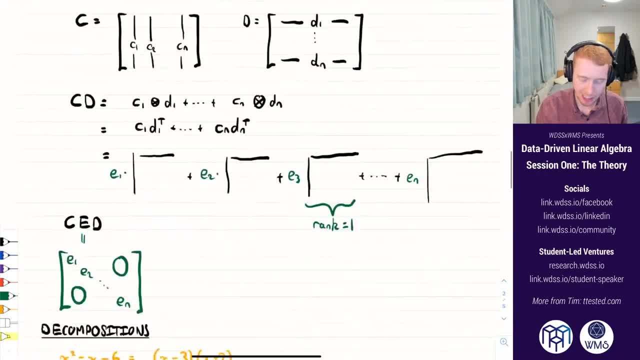 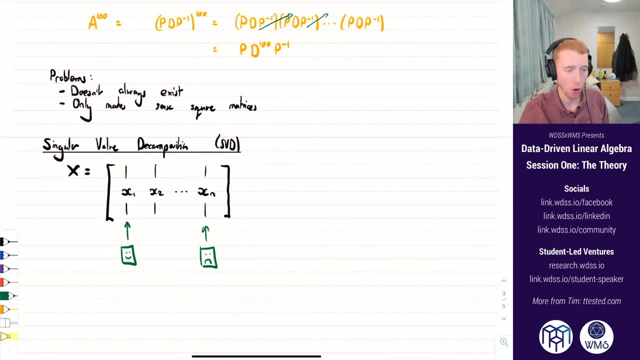 As the rows. But it turns out that all of the theory of the singular value decomposition Works best when our observations Are column wise, And so, to avoid confusing you When you go and look at other resources on the SVD, I've decided to stick with the convention. 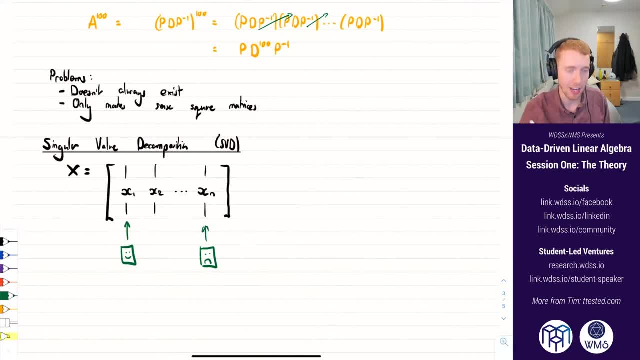 But I do encourage you to have a think about How things would change if we had them row wise, And I'll point out a few things As we go To explain what changes might be made. And this X here It's going to be a p. 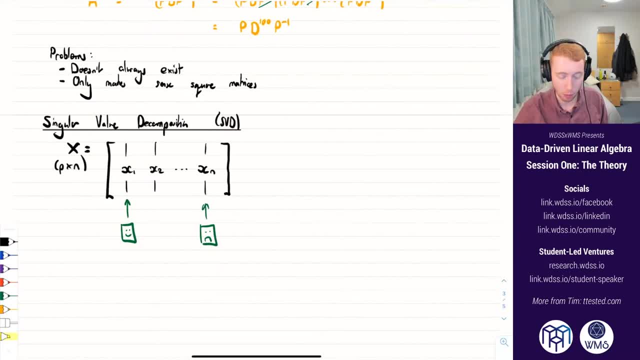 By n matrix, Where p is the number of predictors, So the number of pixels in the image in this case, And n is the number of images that we have available, And so each of these Xi's Is, in the real numbers, A p dimensional space. 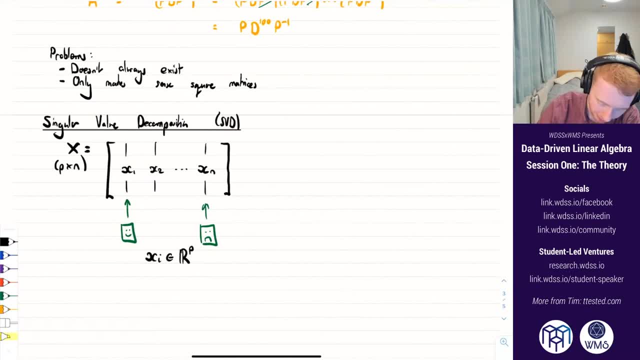 In that- And we're assuming here That p is way bigger than n- We have a lot more kind of pixels Than we do images, Because in most cases That we use the singular value decomposition As a reasonable assumption. Okay. 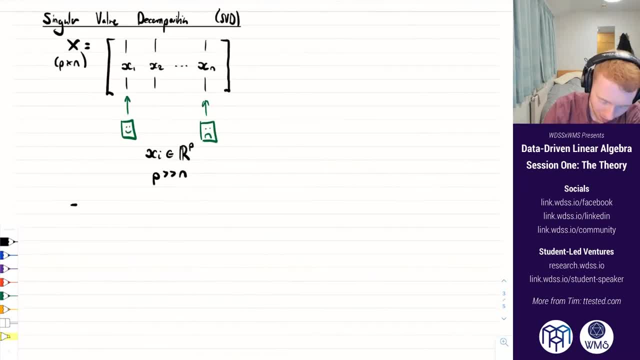 And so the singular value decomposition Says that we can write X in this format. So U Sigma V transpose. And so what do these matrices look like? Well, U Is going to be Okay. so I see my screen is frozen for a second. 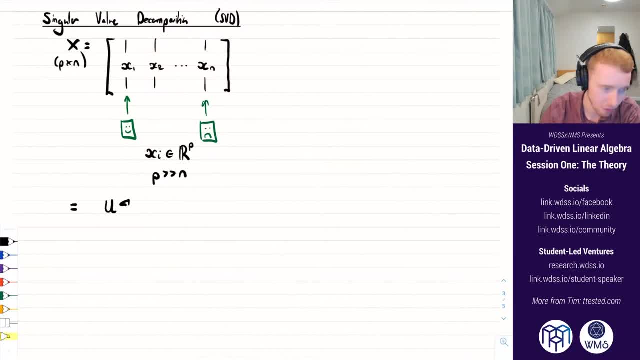 So we'll just give it a second to reconnect Or you won't see what changes I'm making. So we're going to write it as this U, Sigma and V transpose And these are going to have really Kind of tangible real world interpretations. 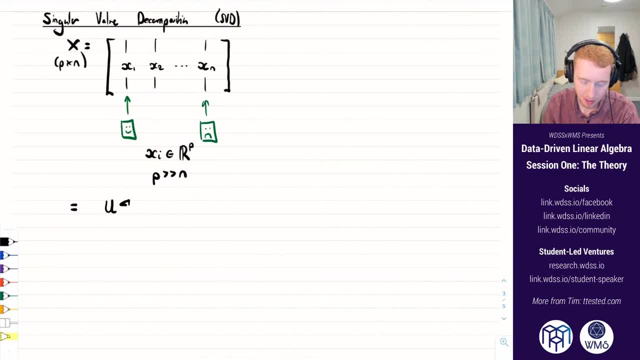 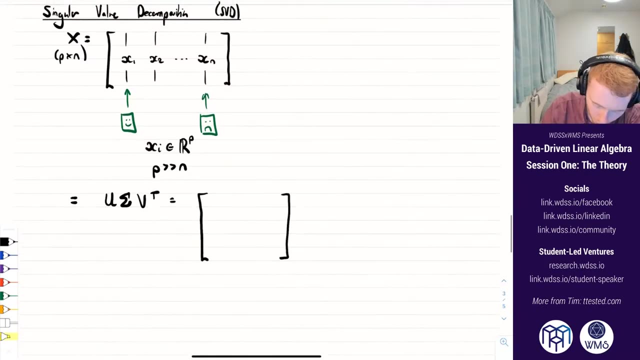 So these are not kind of Generic matrices. These actually represent something about our data And we can use that For understanding more about what our data Is doing. So I think everything is unfrozen now. There we go, So U is going to have these columns here. 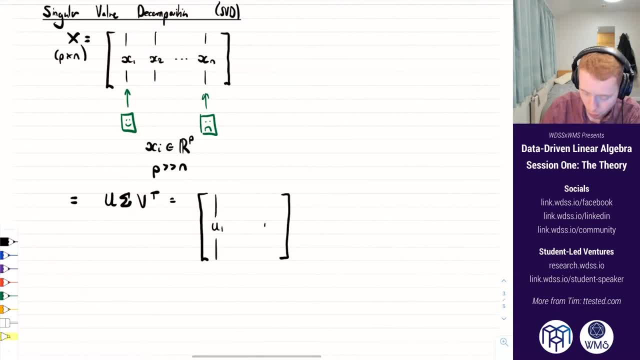 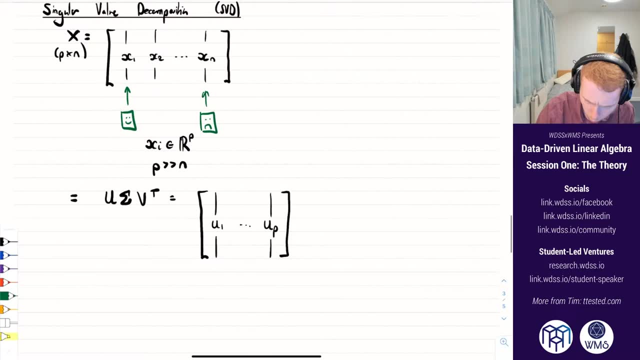 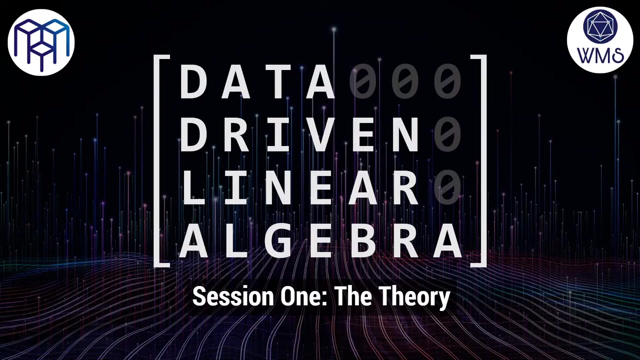 U1. Up to U P, And what each of these represent Is kind of What we'll call an eigen face. Okay, Seem to have lost complete connection To my screen. Let's just try reconnecting that, I hope. 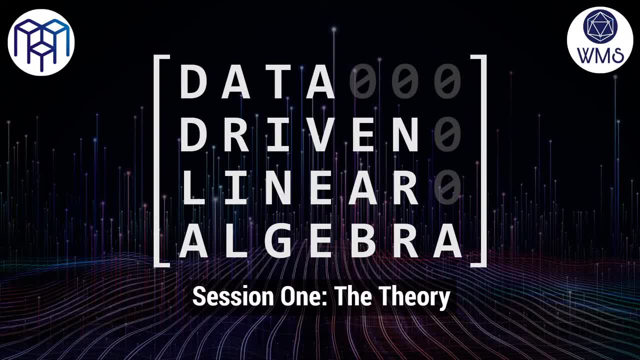 This works. It doesn't work. There we go Something's different. Okay, So we're looking at this randomness And so you can see what happens with this Very An eigen face. So This is what we were looking for. 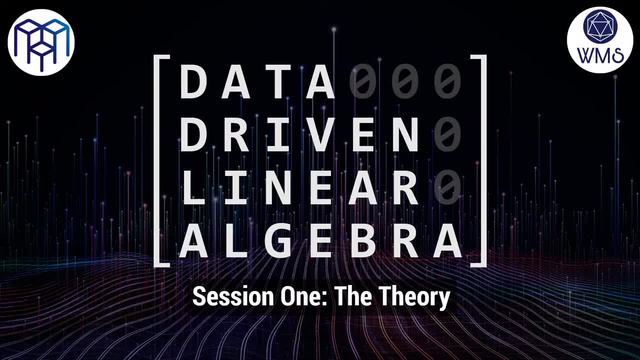 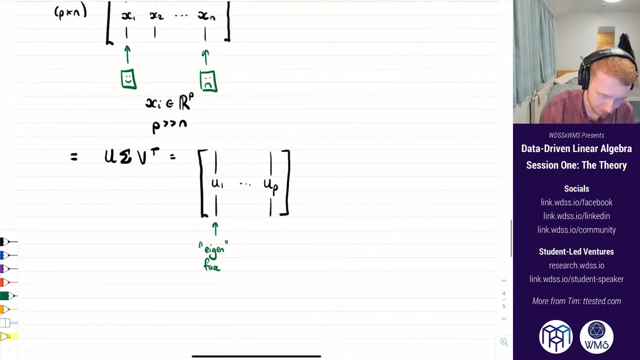 So, okay, we should have the screen back again. um, sorry about that, okay. so so these are our eigenfaces, um, and so these, each of these look like um a face, but they're um. the idea of these is that these each represent um kind of the most important aspects of what makes a face so 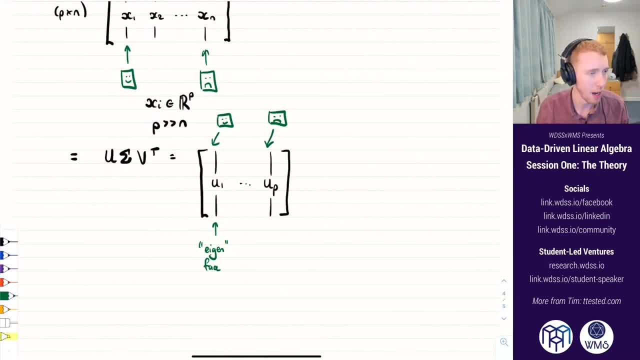 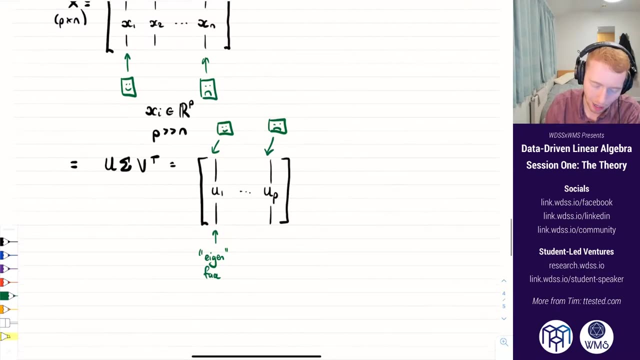 these are arranged, um, hierarchically. um, i assume everything's coming through again. okay, now it would be great if someone could uh let me know in in the chat. um, and so these are kind of arranged hierarchically in order of importance. so, uh, you can think of this as like a new basis for our 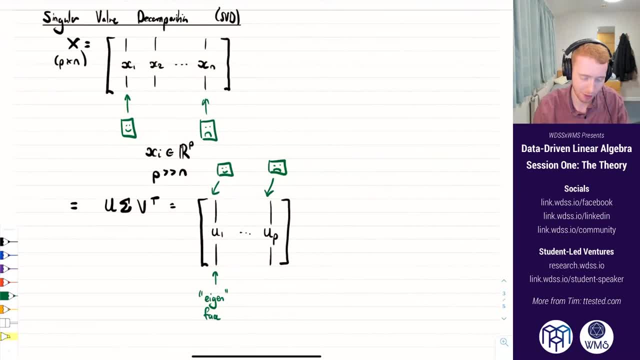 faces, kind of um, a palette that um can be used to compose all of the these faces. and u1 essentially is the most important aspect of what it means to be a face, and then u2 is a bit less important, u3 is a bit less important, and then we can add all these um together um to make up a face. 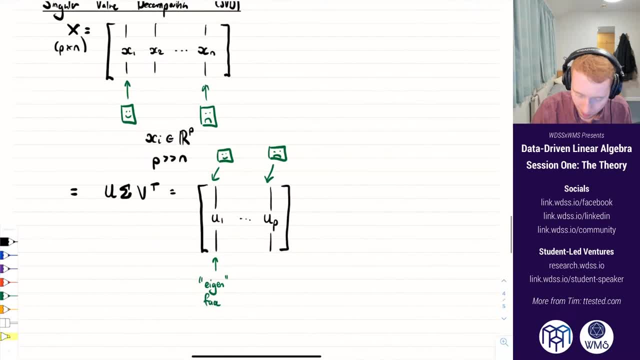 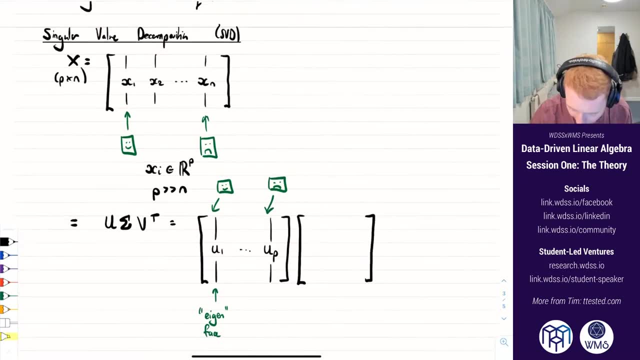 and the important thing, those are ordered and the importance is of these um given values are represented by the values in this sigma matrix, and so sigma is a diagonal matrix looking something like this: uh, going up to p, with then just zeros padding the bottom here and the rest are zeros here. so it's diagonal, but it's a rectangular matrix, just padded. 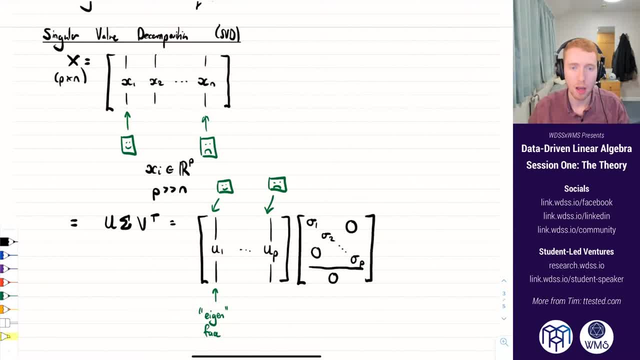 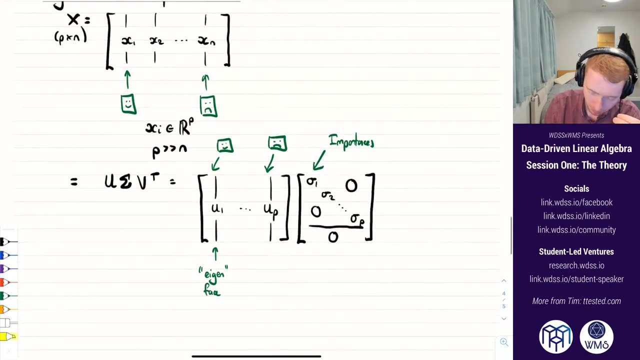 by zeros, um, at the bottom there, okay, and so these different sigmas, these give the importances, um, what the corresponding importance is for these vectors, uh, u1, up to up, okay. and then finally, we have this vector v, transpose, which i'm going to write by transposing the insides rather than the. 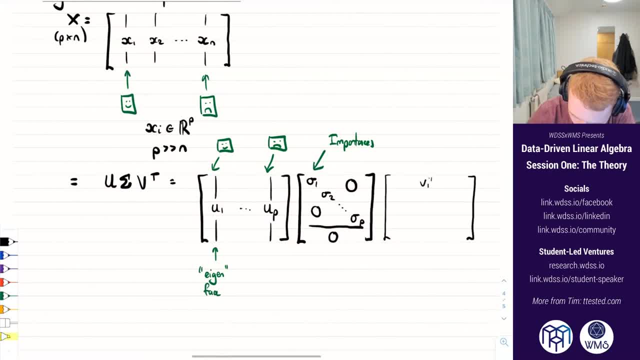 outside, which is going to look something like this. so v1: transpose all the way up to vn: transpose. as i let you point out, this is a p by p matrix, this is p by n and this one is n by n, and this has maybe a bit harder uh of um, of um kind of an interpretation behind it. but what this? 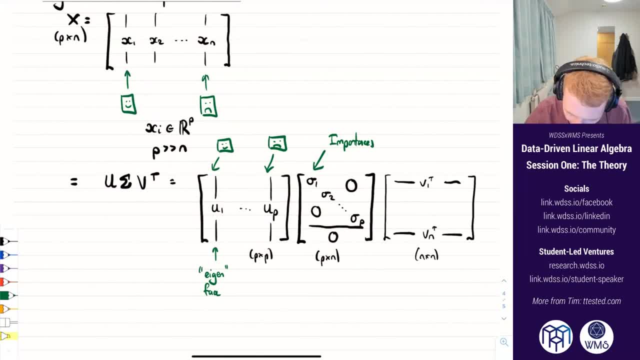 kind of means is that um? each of these columns here, so i'm crossing across the rows. what these represent is the mixtures um of u1 to up, um needed to reconstruct, um, reconstruct x, um. well, in this case it's x1 and the next one would be uh for x2, x3, etc. 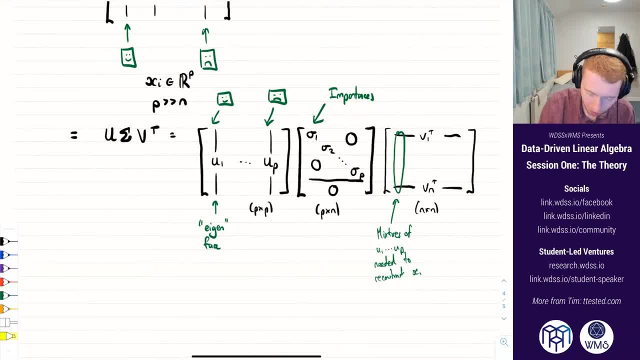 so these is kind of, you know, a palette in order of importance, and these columns here, that kind of cut across these v rows, determine how we combine these, this palette, together to reconstruct our initial thing, um, and then we also have, um, these, uh, these rows across here. 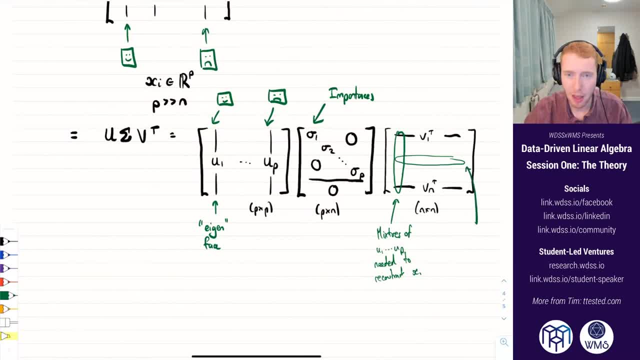 and so what one of these rows represent? um, these are essentially how um kind of the mixtures change, so like i guess, yeah, so they're essentially kind of like a time series. i'm gonna put this thing in quotes again. um, for for how? the contribution, contribution of one eigen face. 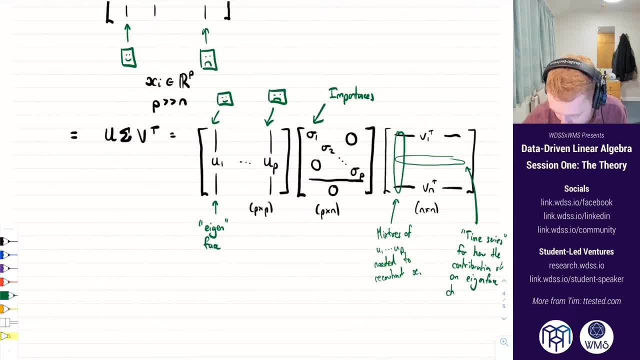 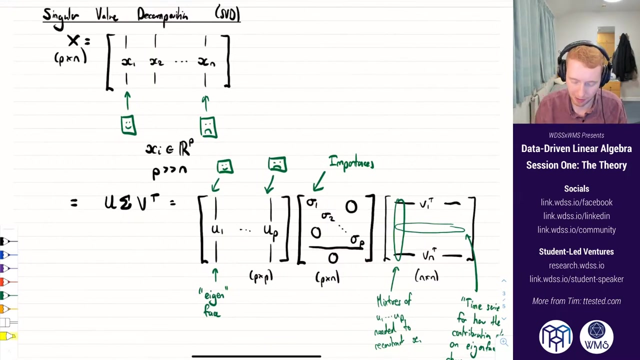 um changes over observations. so this one in the middle here, this corresponds to some eigen face um in the middle of uh, this new matrix here and it shows how for every single matrix or every single face in our original data, how the contribution of that changes as we work through the data set. 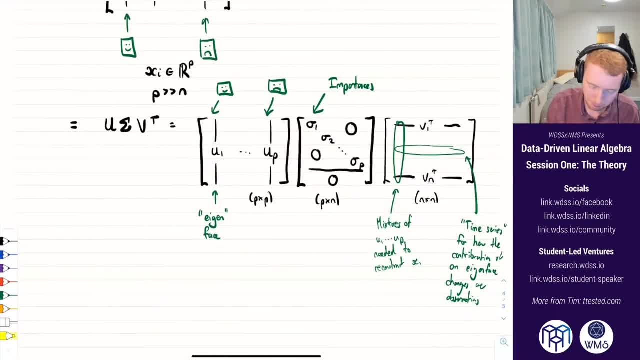 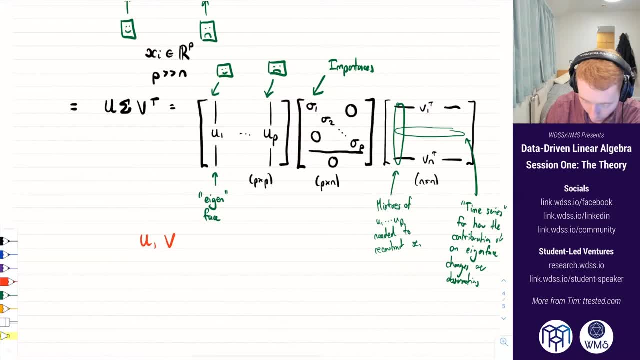 so that's kind of the intuition of what this representation um means, and there's a few conditions that we put on these. so u and v are orthogonal, and so what we mean by that is that you know u transpose u, is u transpose um, is u u transpose? 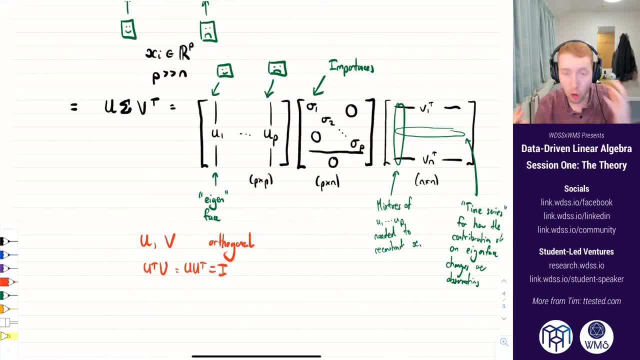 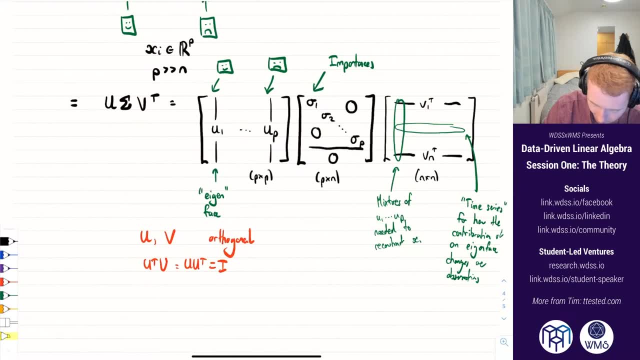 is the identity, and then the same for v, or in other words the geometric interpretation. these are rotations. and then, uh, for sigma. we have the assumptions that these sigmas are decreasing in value. so we're going to be able to do that by taking the eigen faces all the way down to sigma p. 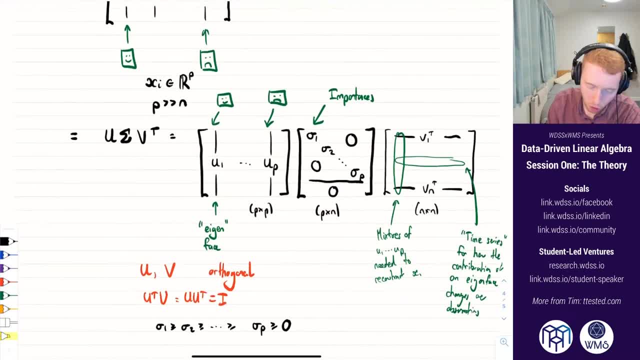 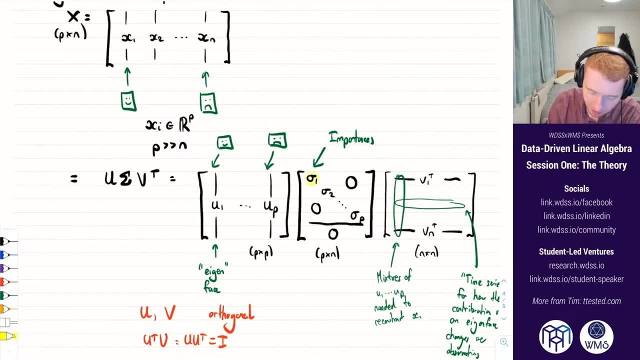 which is greater than or equal to zero. so, summing this all up, the way that we view this thing, the value decomposition is that we break up our image into these different kind of components, ordered by their importance. the importances are given by these sigmas, and then this um, this v matrix tells: 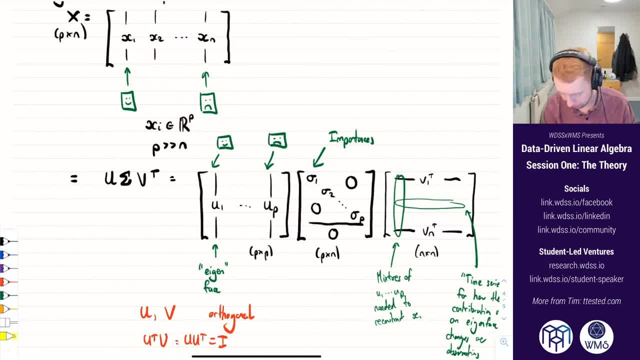 us how to take these eigen faces and combine them together to reconstruct the original. so that's what the singular value decomposition is, and these are known as our singular values. uh, these are known as our left singular vectors and these are known as our right singular vectors. so with that, we're going to pause for a minute or. 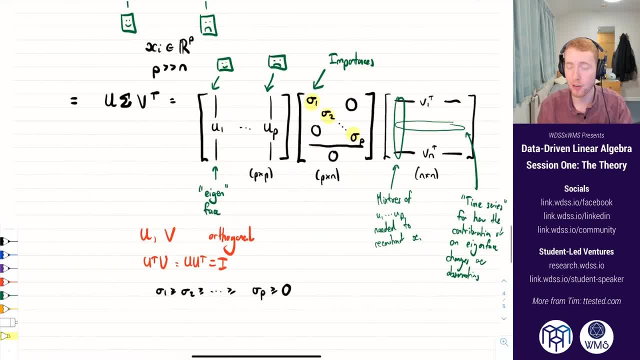 two um just to have a quick break. if you have any questions, pop them in the chat now. um, otherwise after that we'll go on to the properties of the svd, um, how we can represent this as the sum of low rank matrices, and then the geometric interpretation of the svd. so join back again. 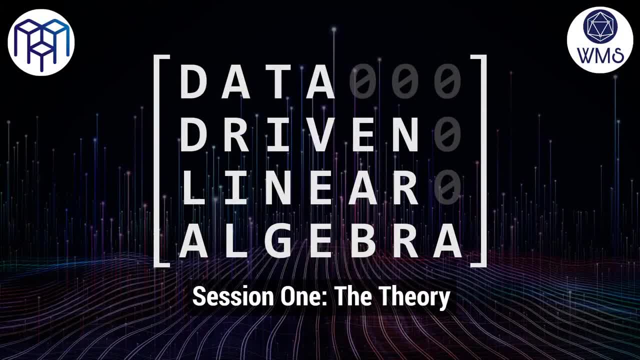 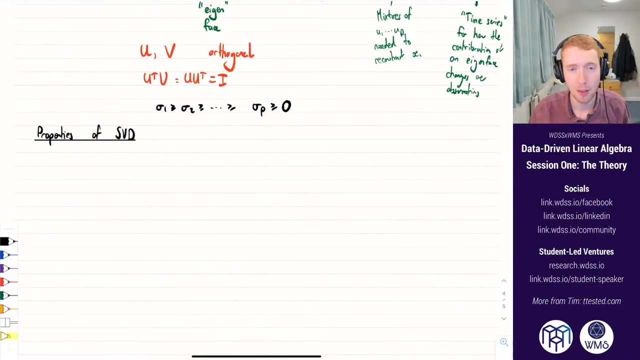 in a minute or two. so Okay, welcome back. So we're now going to have a look at the properties of the SVD, just a few high-level properties. So the first one is that the SVD. well, actually, let's start with the most important one: it exists. 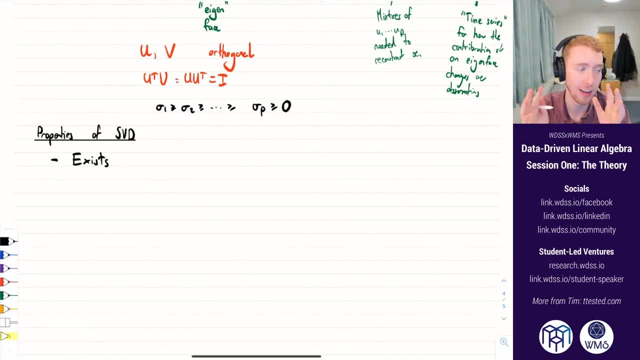 So for any single matrix the SVD exists And this is a really powerful property that we didn't have with the eigen decomposition And actually many decompositions do not have guarantees of existence. We'll show that it exists by actually deriving the SVD and computing it. 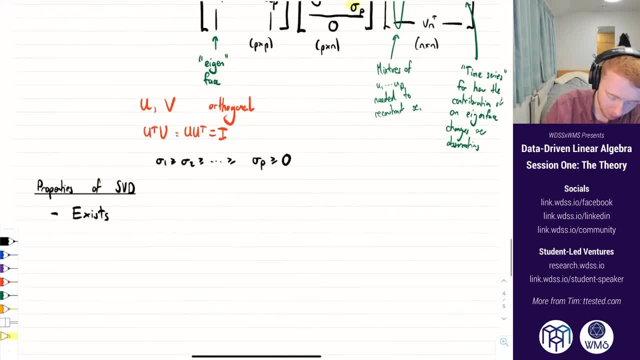 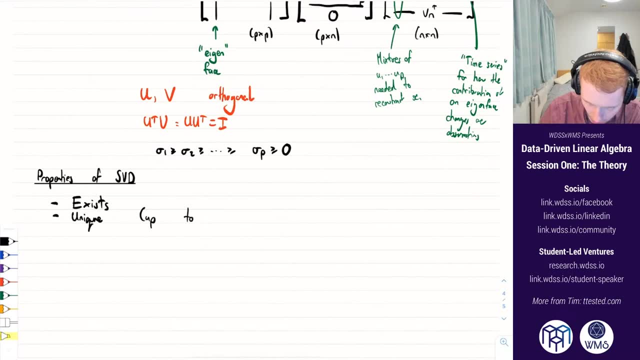 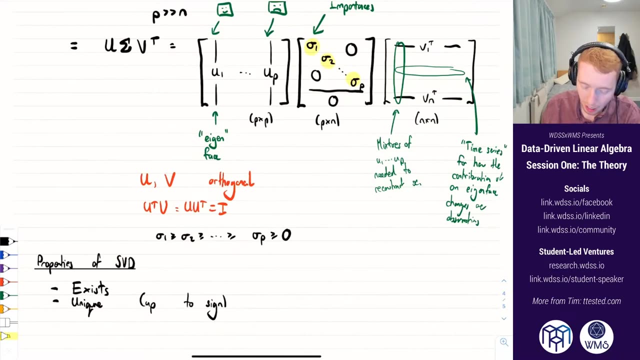 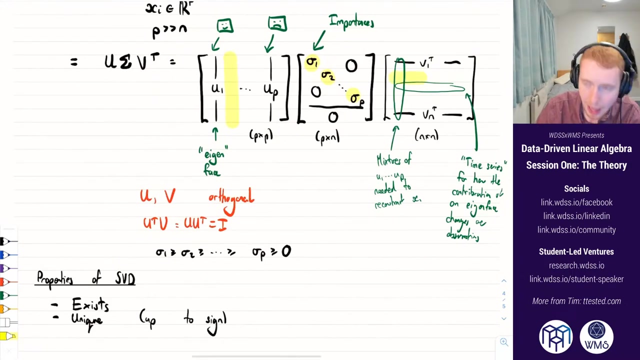 In the second session. So that's nice. And secondly, it is unique Up to sine. So, given these conditions, that u and v are orthogonal and that these sigmas are decreasing, the matrix is unique, Apart from, let's say, if we took u2 and v2 and negated both of those. 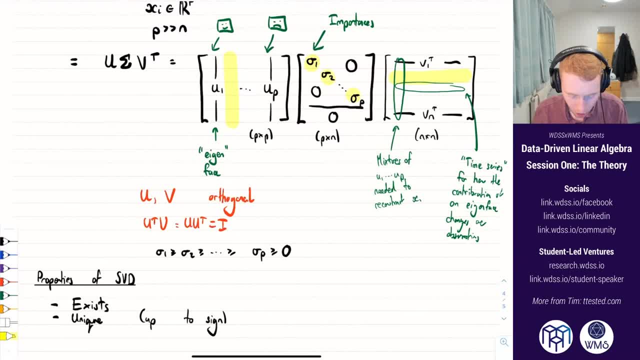 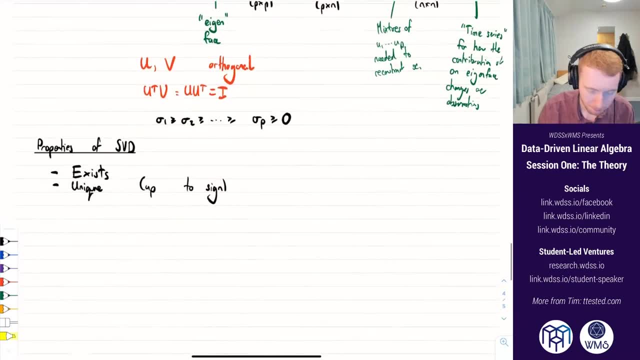 then we'd also get another SVD That was e2.. So, apart from changing the signs of those, we have a unique decomposition, So that's a very useful property. What else do we have? So if the matrix x is real, then u and v will also be real as well. 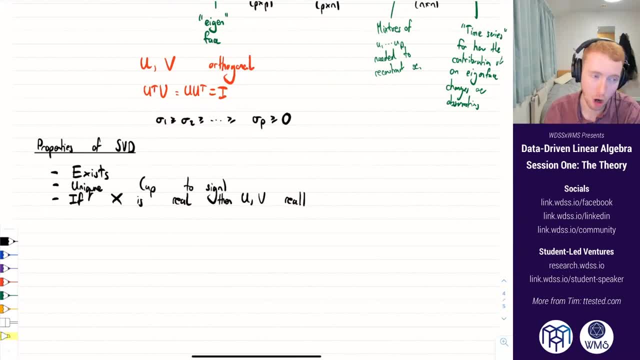 So again, that's nice, We can stick in the world of real numbers. But if x is a complex matrix, then no guarantees on u and v. Okay, What else do we have? I guess we can have. so yeah, So these sigmas are allowed to be 0. 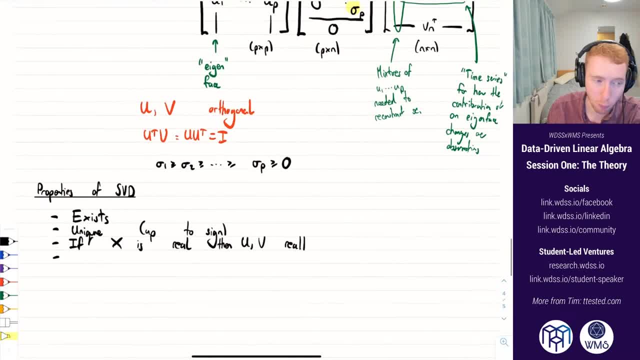 And they can become 0 at any point. Say, maybe, from sigma 4 onwards, they're all 0. Well then, so the number of sigmas that are not 0, that is the same thing as the rank of the matrix x. 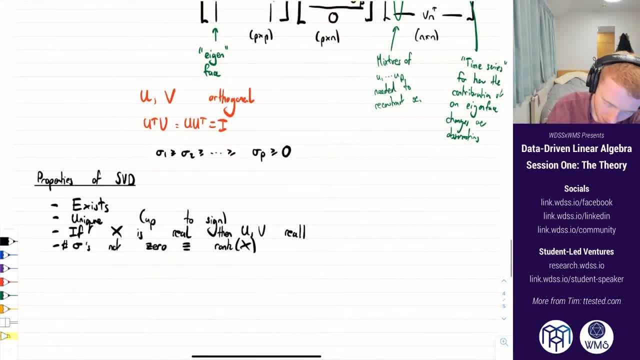 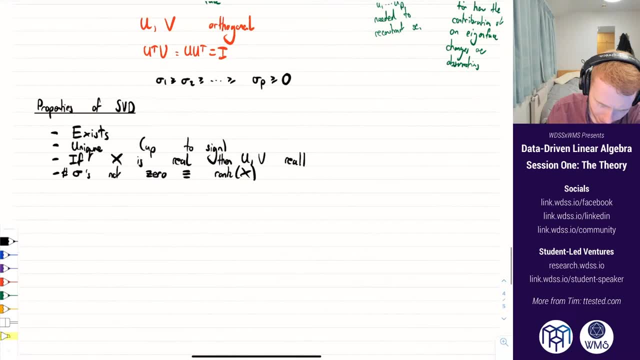 And we'll actually see why this is in a moment. So that's a nice, nice property, Okay. yeah, there's one more property that I won't mention here. I might get time at the end just to add it, Okay. 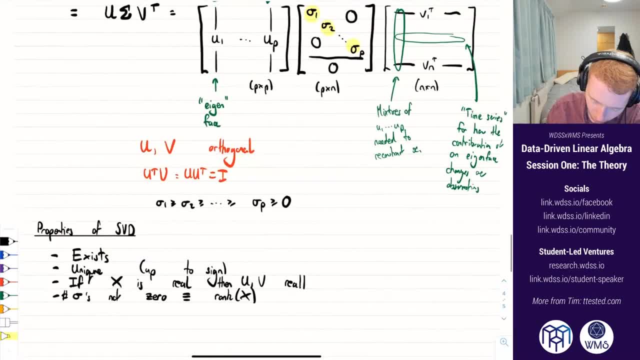 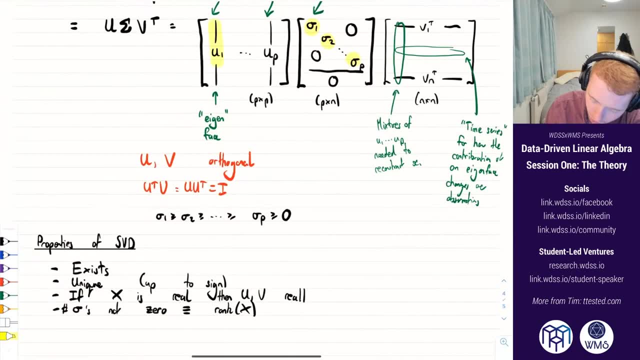 So now, the most kind of important thing is that. so we look at this matrix here. We have a matrix of columns, We have a matrix of rows here and a diagonal matrix in the middle. So this brings us back to this result that we showed before. 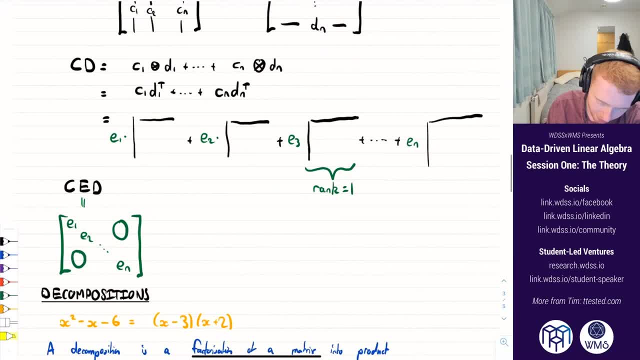 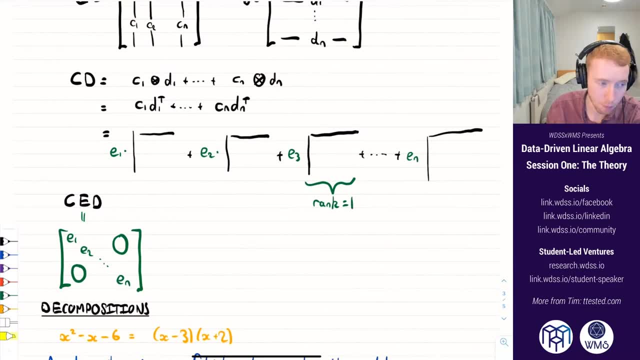 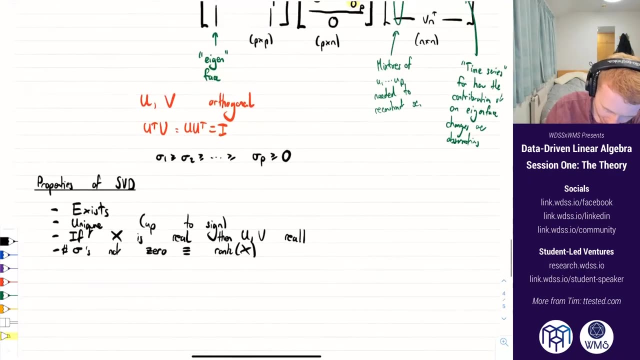 You can reference it. You can represent a matrix with a diagonal in the middle when we have them as columns and rows, as this sum here of these rank 1 matrices, these rank 1 outer products, And so what this actually shows is that we can take the matrix x. 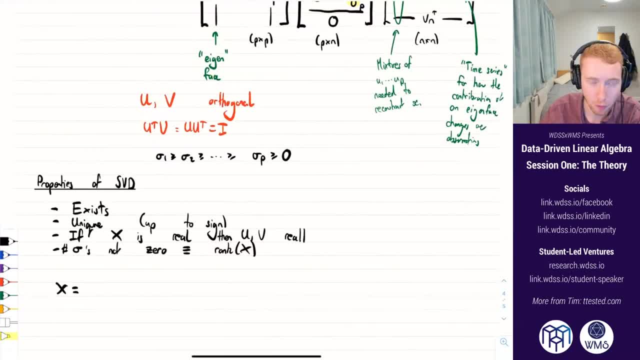 and write it in the following format: So x is sigma 1.. It's going to be u1, v1, transpose plus sigma 2, u1.. Sorry, u2, v2, transpose all the way up to sigma p of that doesn't seem right. 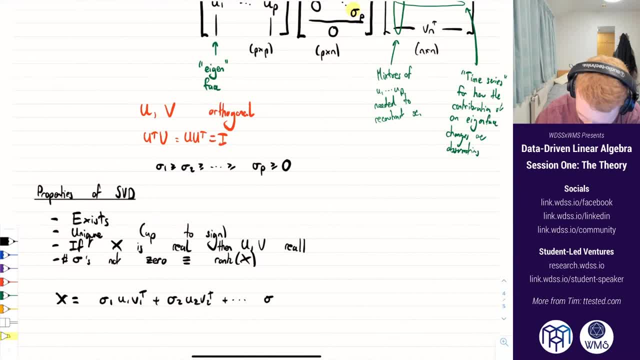 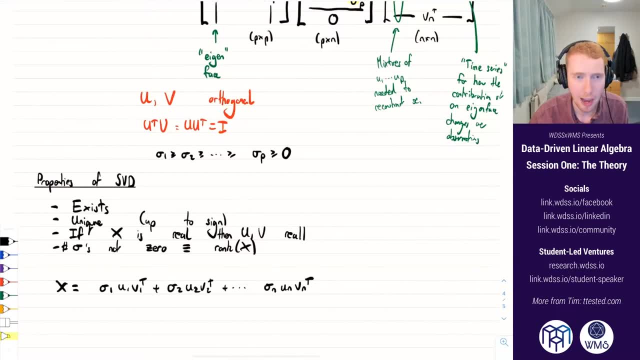 No, it's going to be up to sigma n, because we'll reach the zeros first. Sigma n of un vn transpose And I think that makes me realize. I think that there's a mistake in my matrix. Yeah, this should be an n here. 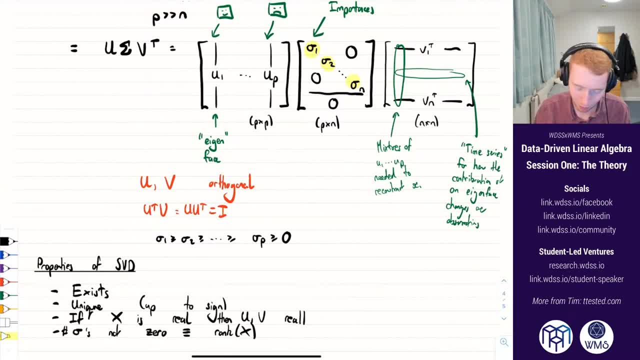 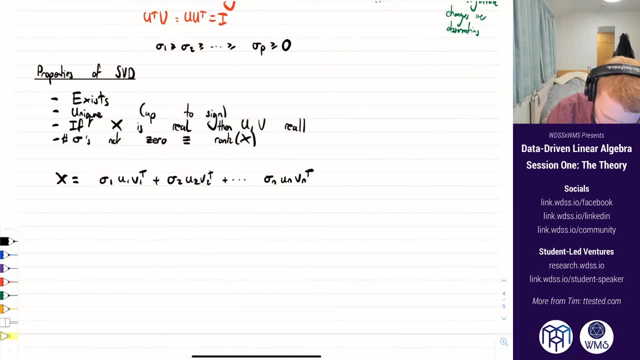 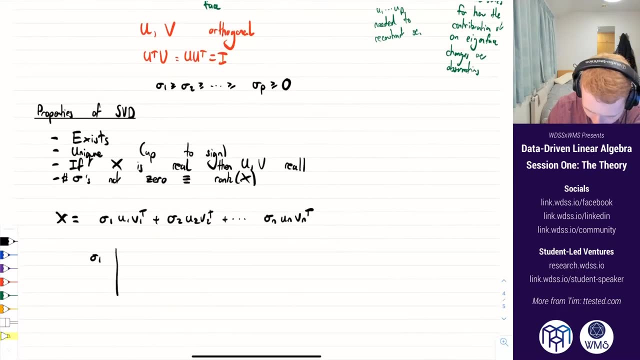 Because it's a p by n matrix, So there can only be n diagonals going across And p is much bigger, which is why we had the zeros at the bottom there. So we can write x like this, And just a reminder, you know u1 is a column and v1- transpose- is a row here. 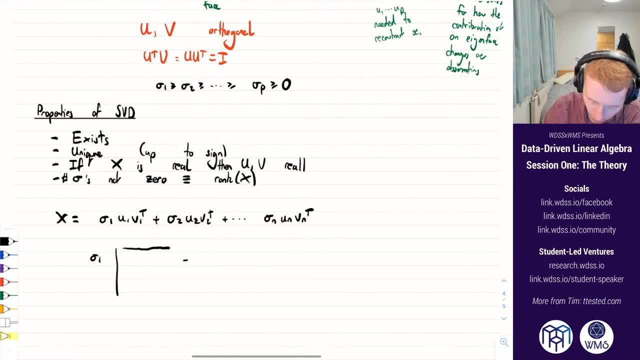 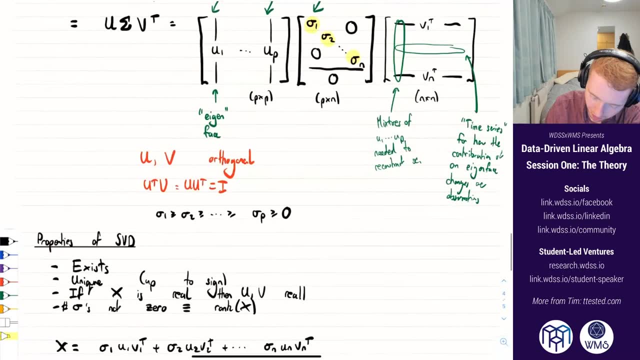 And that's going to give us a matrix here which has a rank of 1.. So basically, it's just going to be yes, yeah, this is the point I was making earlier- that these ones across here, these v's, are the combinations of: 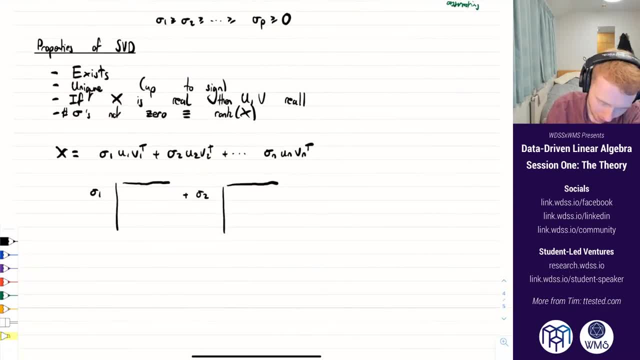 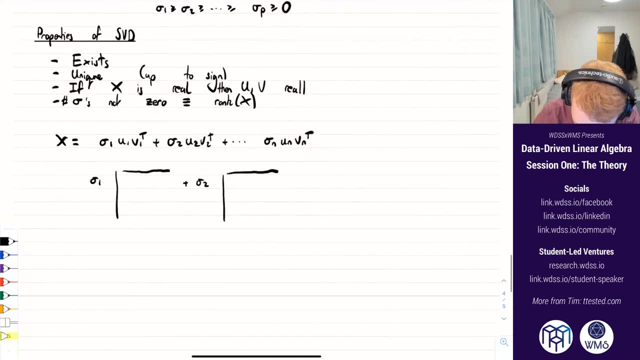 each u1 of each of these components over time or over each observation. So we're just taking different amounts of these over time, different amounts of our palette over time. That goes all the way on to sigma n: un vn transpose Okay. so why do we care? 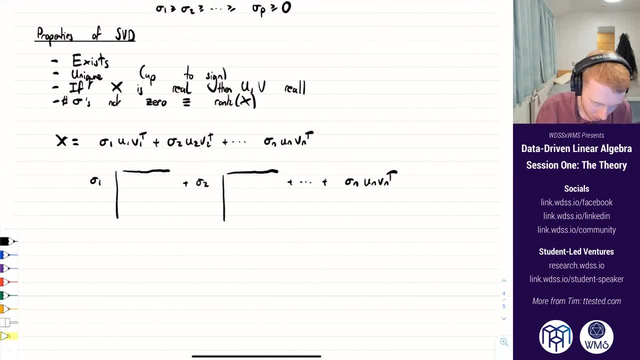 Like: what's the important part of this? Well, the important part is that these sigmas are decreasing, And so you can think of this. as you know, we decompose this into these rank 1 matrices, But the contribution of each of these matrices gets less and less as we go through. 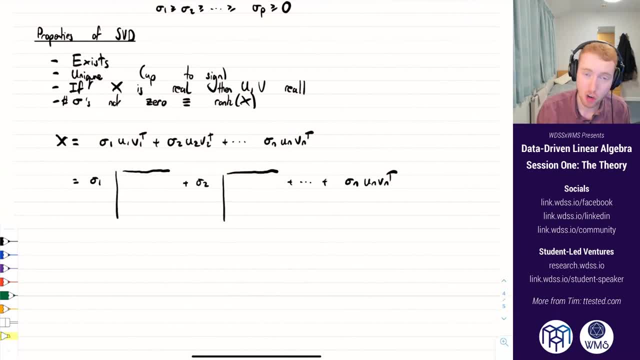 So this sigma 1 is probably pretty big, showing that this first combination contributes a lot to the matrix. This next sigma 2 is probably still pretty big By the time we're at sigma n. this is adding nothing. This is a really tiny contribution to a matrix. 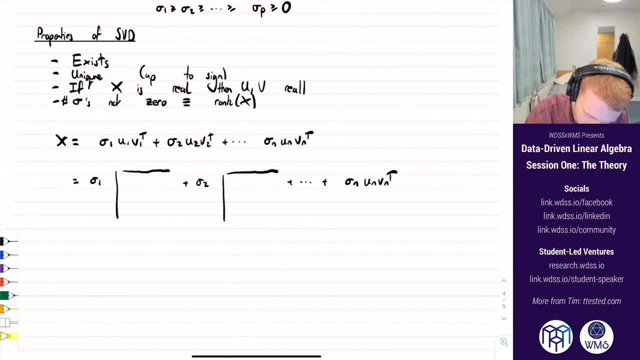 It might even be zero, And so the idea is, at a certain point we're going to call this r, we're going to cut things off and just stop it, We're going to truncate it, And that's going to leave us with an approximation of x. 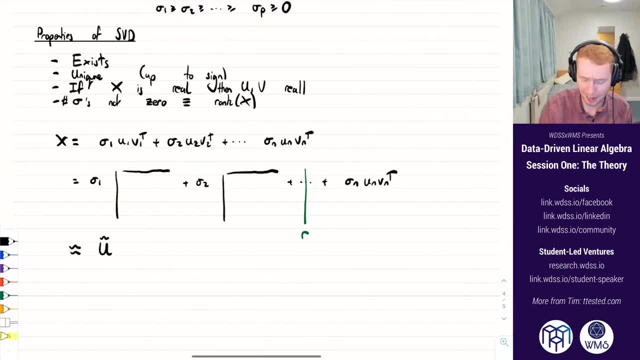 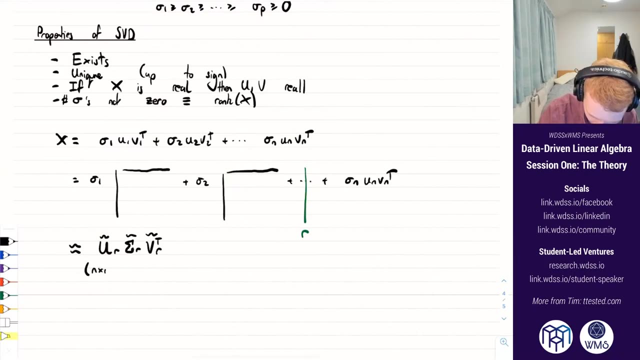 which is going to be u. We're going to put a hat on it, Sorry, not a hat- a tilde for approximation of rank r, Sigma approximated rank r, And then v transpose approximated with a rank r, And so these matrices are going to have sizes n by r, r by r and r by p. 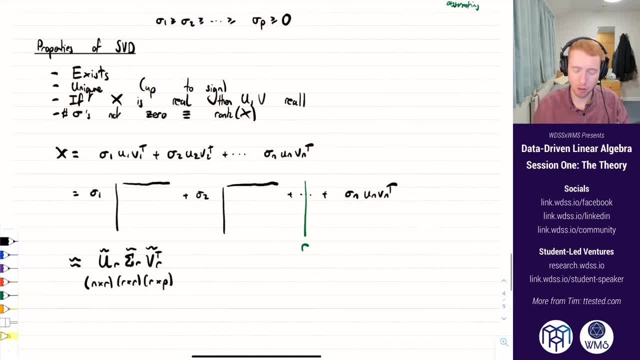 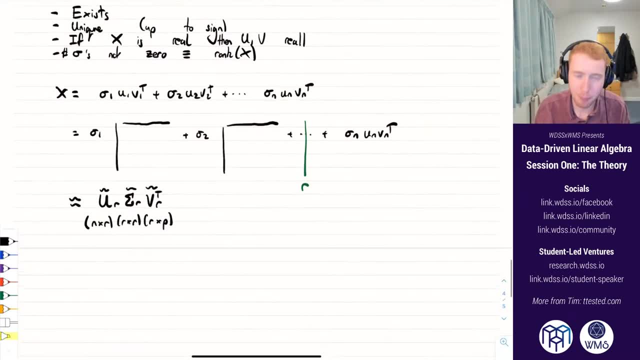 Let's be taking this massive matrix x, and we've collected, We've collapsed it down into only a few underlying out-of-products that represent the whole matrix, And so that's kind of a really important idea And actually this has a sense of optimality as well. 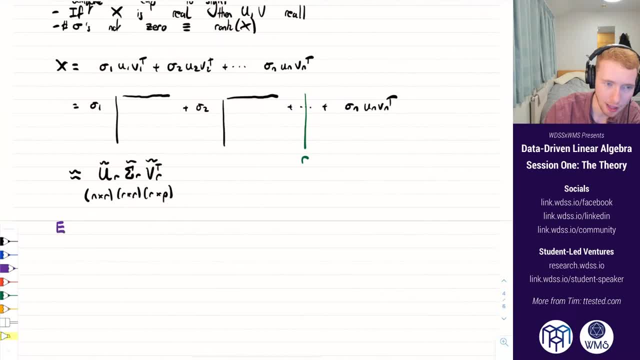 So there's this thing known as the Eckert-Young theorem. I believe there was a third person involved, but I forgot the name of that, so apologies to that person. And that was proved in 1936. So still fairly recent maths. 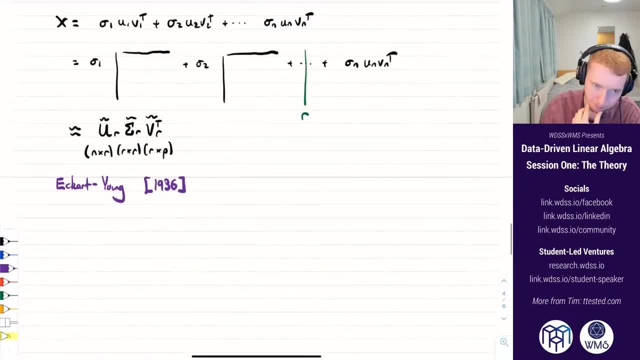 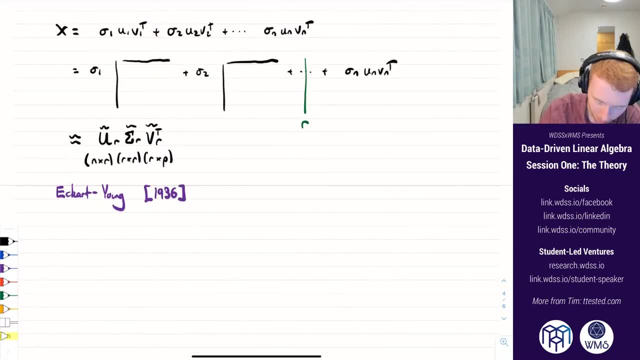 And that says that this approximation, Yeah. so what the Eckert-Young theorem says is that let's consider all possible approximations of the matrix x, So all kind of possible matrices in the space of p by m matrices, And consider all of those that have a rank. 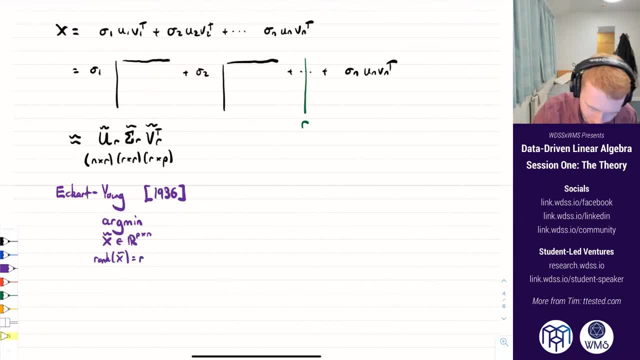 of rank r. Well then, which of these minimise the difference between the actual matrix x and this low rank, this rank r approximation in the Fabinus norm? I'll define the Fabinus norm in a second, So kind of what minimises the distance between these two matrices? 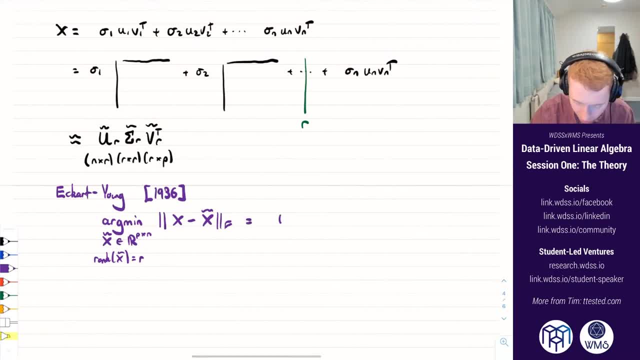 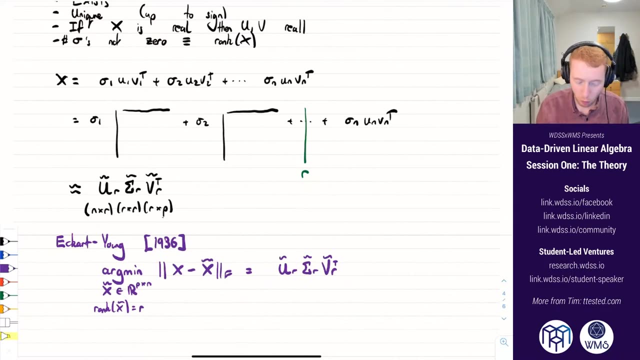 It turns out that this minimising matrix is this matrix here, And so, in other words, when we take this and truncate an r, that is the best possible truncation. we could do So if we wanted to represent our matrix using only kind of a certain amount of compression. 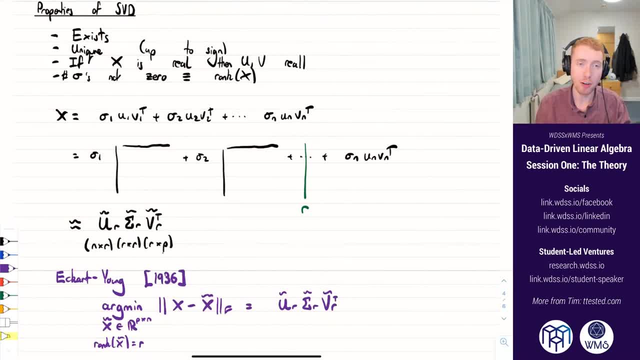 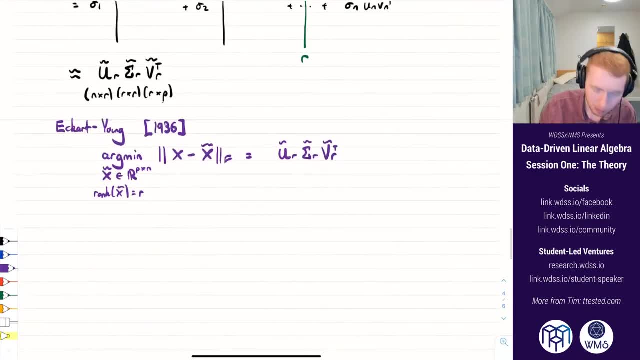 a certain amount of low-level representation. seeing the value decomposition will give us the best possible way of doing that. There was an efficient way of doing that, And that's in the Fabinus norm. Let's just define what the Fabinus norm is. 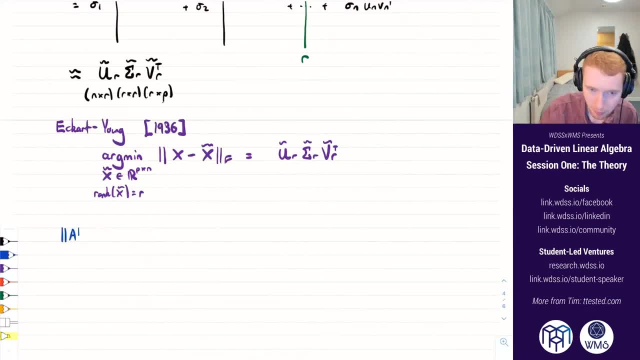 Let's say we have a matrix A And then the Fabinus norm is a matrix A. The Fabinus norm is the square root of each of the entries of this matrix squared. And so another way to think about that is: take the matrix, flatten it out into a single vector. 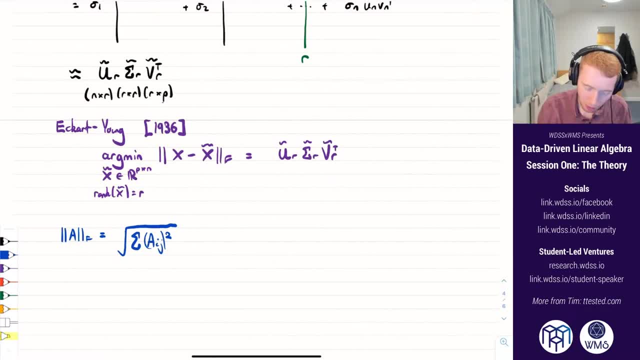 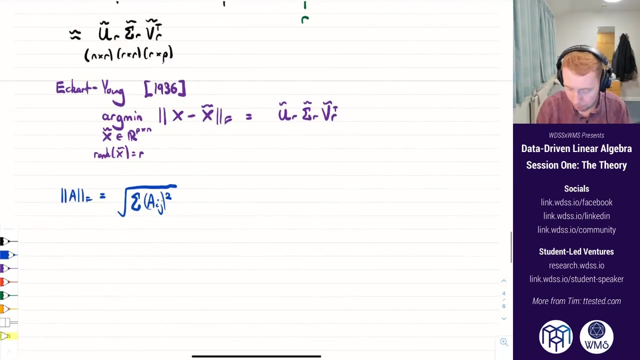 and then consider the length of that vector, And so this x minus x x tilde in the Fabinus norm is essentially: you flatten both those matrices out into vectors. What is the normal Euclidean distance between those? Well, the normal Euclidean distance between those two vectors is the length of the matrix. 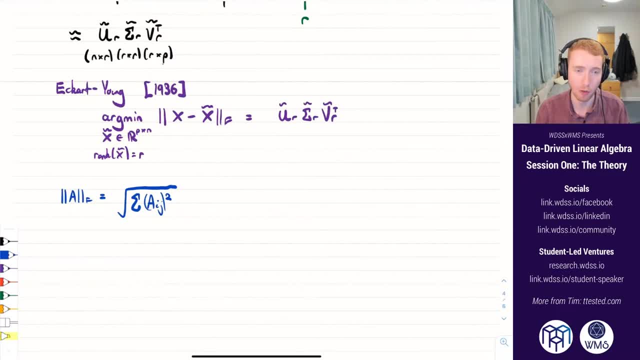 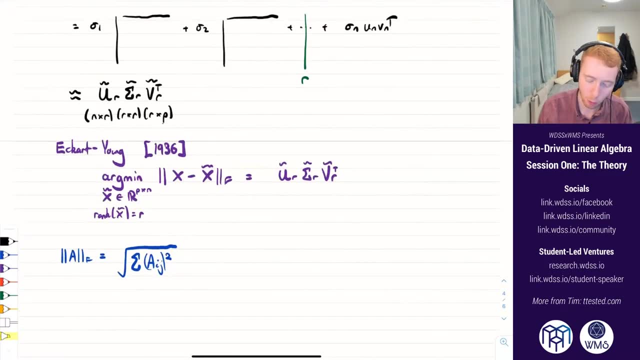 And so that's the Ecclid-Young theorem, And that kind of is what gives the singular value decomposition all of its power. OK, so now let's consider well, when should we truncate this R? When's the correct point to cut that off? 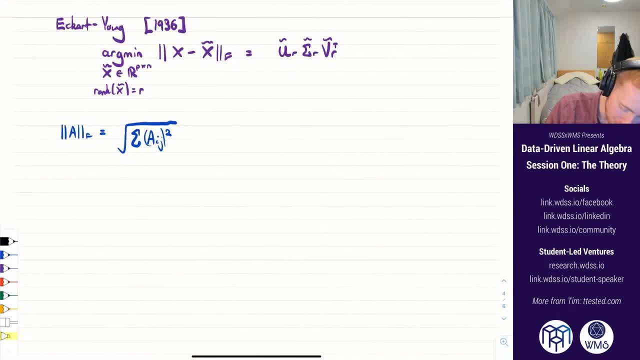 And so to do or to answer this question? what we can do is we can draw a graph, And usually we would do this using a computer, But for now, we're just going to imagine we've done this already And we're going to put this in a graph. 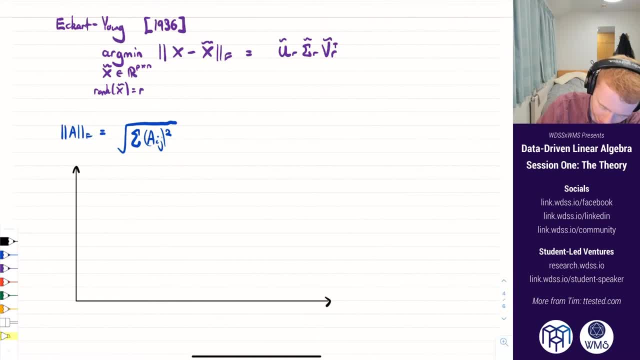 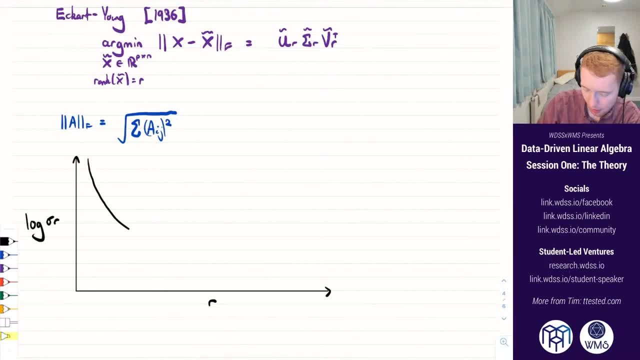 And what we hope to obtain is something that looks a bit like this: say OK, so we know that these are decreasing And we want to pick a certain R at which to truncate, And we can do that by looking for what we call an elbow. 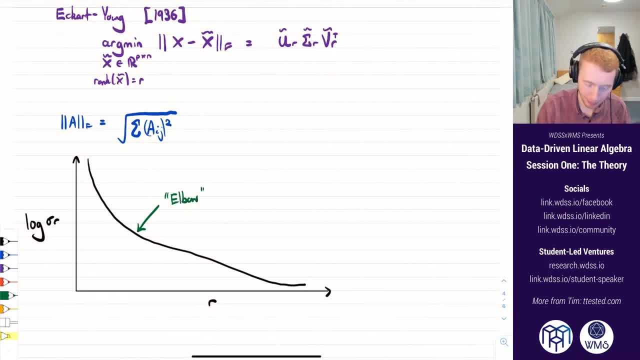 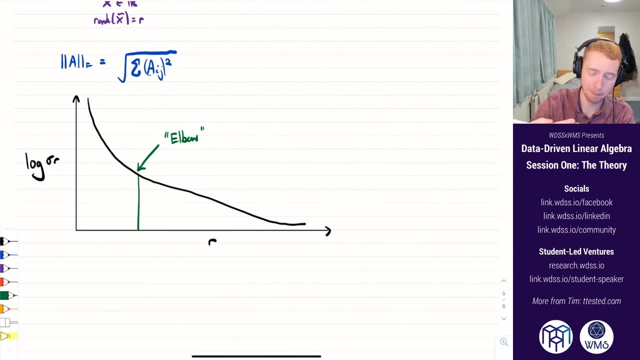 And this is kind of a place in the curve where it starts to flatten out a bit. So this would be a good place to truncate, Because after this point, every added bit of data, every added kind of a bit of rank to the data, the amount of complexity to the data, it doesn't add as much explanation to. 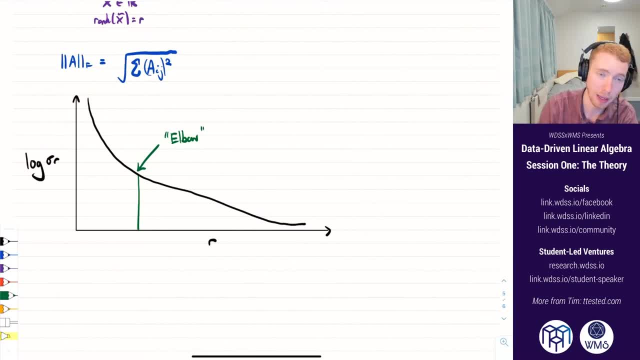 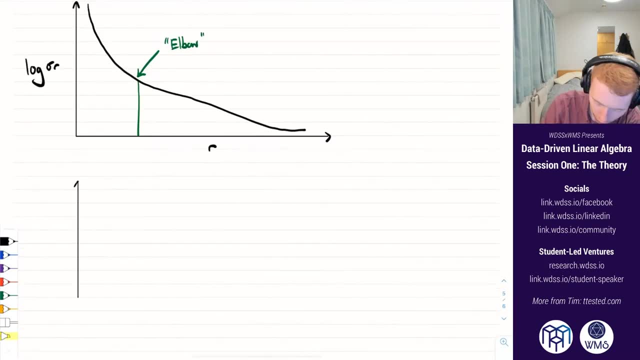 the actual matrix. So basically we can get a pretty good approximation by stopping here. Another way of looking at this would be to draw this other graph here. So again, we're going to go along R And then we're going to do this. 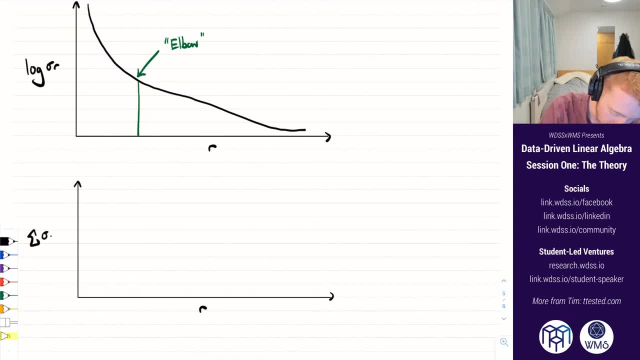 And then we're now going to look at the sum of all sigma- i's going up to R And this will look something like this: a tailing out. And then what we can do. we can pick a certain point here, say, 99% of all the sigmas cut. 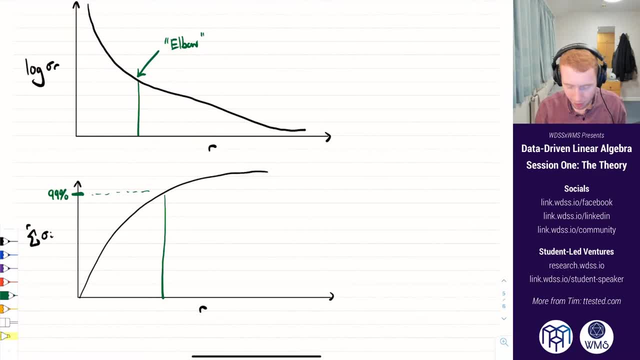 across And that's going to give us the R, And so this way, we can represent 99% of the information in the matrix using only a certain number, And so we can then take the data from the R and we can then use it to make a new representation. 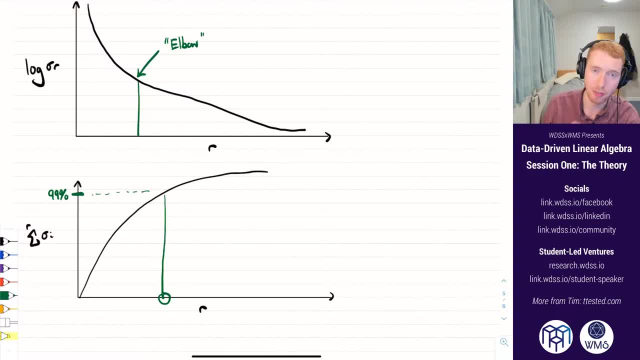 of these low rank matrices, or with a matrix with this low rank R here, And we'll actually look in the second session of a formalisation of this called the Gavish-Donico method, which was derived in 2014,, which actually gives us an algorithm which has proved to. 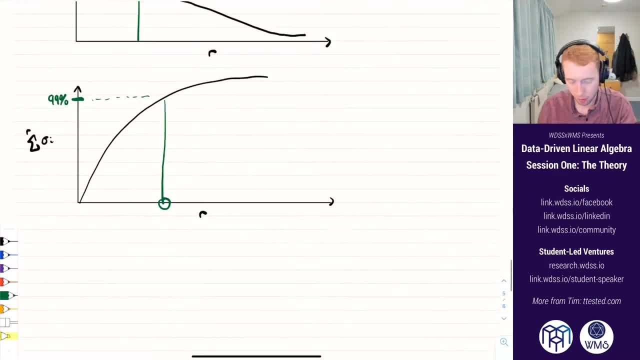 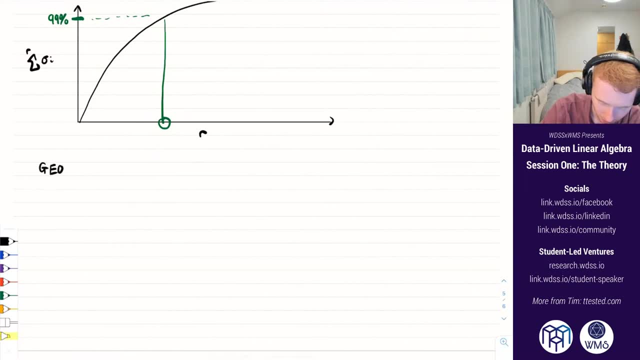 be optimal, under certain conditions, for where to find this R cutoff. But for now we can plot something like that. minutes. i'm going to talk about the geometric interpretation of the singular value decomposition. so the geometric interpretation, you know, what does this singular value decomposition? 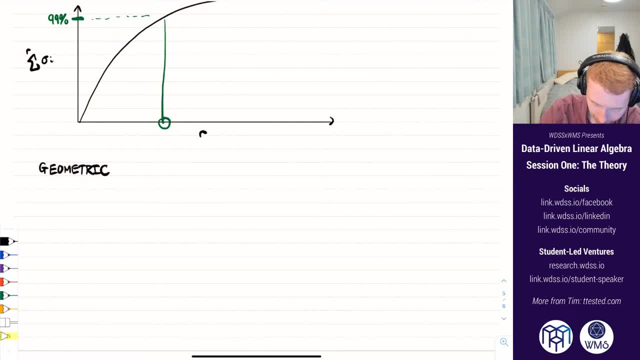 actually tell us geometrically about our matrix. okay, so we have um our matrix x and it looks something like this: so this was um, a p by n matrix, if you remember, where each um, each column is an observation and each row is one of our predictors. so we can multiply this in two ways. we could take a, um an n by one vector, let's call this v. 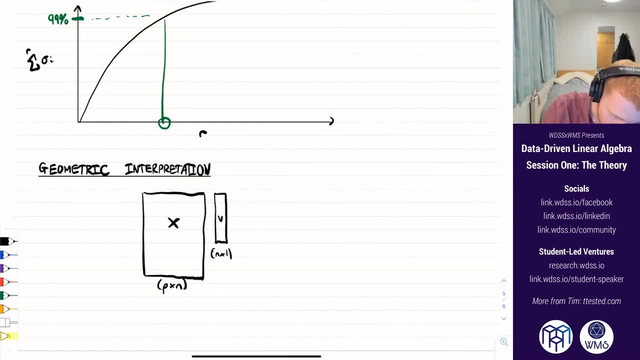 and take this vector and these are our values. times that on the right. or we could take kind of a row vector a, 1 by p vector, we'll call this u, and times that on the left. And so the singular value decomposition tells us something about. 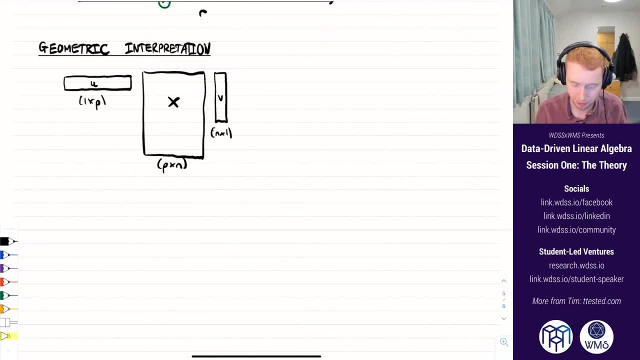 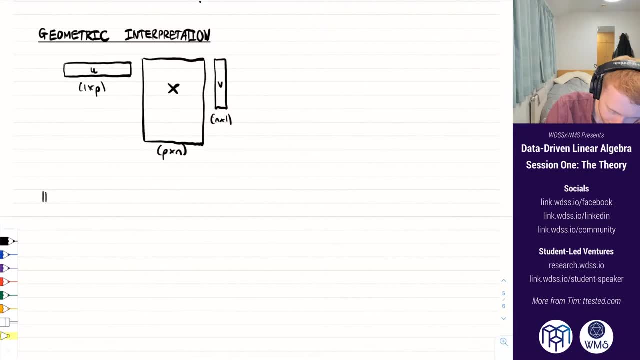 geometrically how these operations take place. So let's start with this right multiplication here. So imagine we have a vector v in an Rn And specifically we're going to take v to be somewhere on the unit sphere in the space of Rn. So imagine we have- okay, I'm going to try and draw. 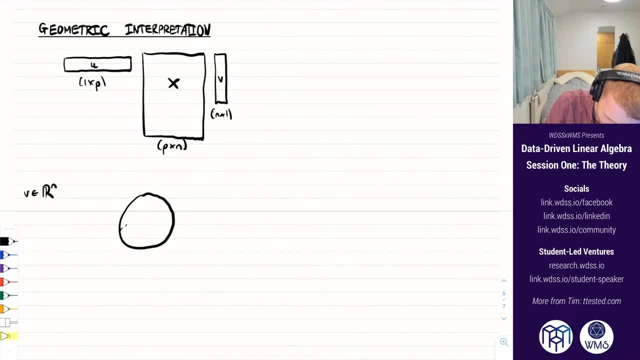 a sphere. It could look something like this: That's not terrible. There's the origin, And then v is some vector on that unit sphere, And then we're going to take that and by multiplying it by x, we're going to transform it into a new space. And this is now going to be. xv is going to be. 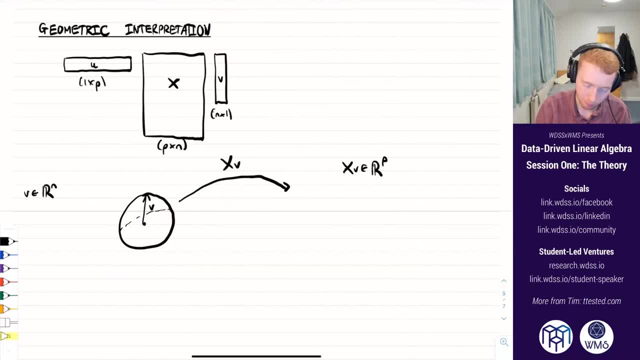 in the space R to the p, because you know n by n, and then we have p by 1, because it's a p by 1 vector, And then so we take this unit sphere here, and when we transform it with x, we're 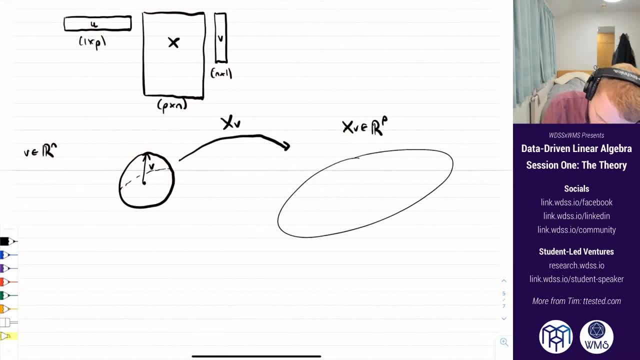 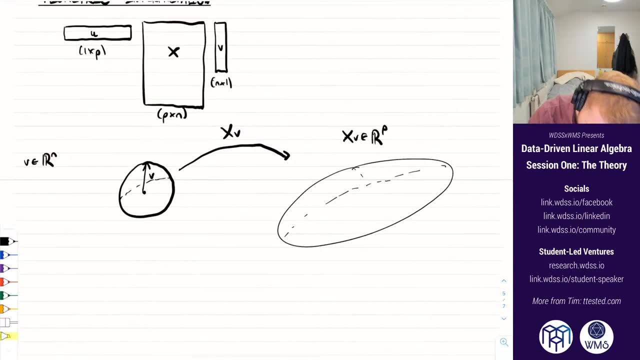 going to end up with an ellipsoid. So this is my attempt at drawing an ellipsoid. And then singular value decomposition tells us something about, geometrically, how these operations take place. So this is the ellipsoid composition. I guess I'll put one across there as well. It gives us information about what this ellipsoid looks like. 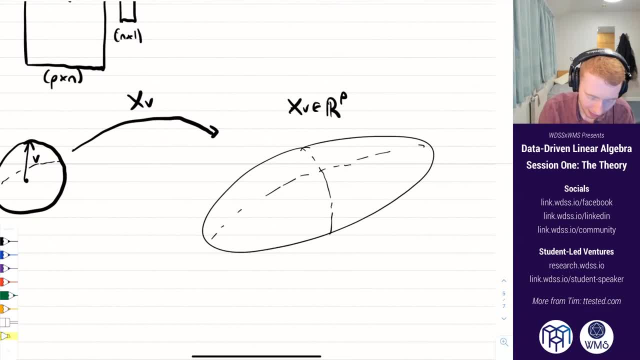 And so an ellipsoid is defined by its principal axes. So it's one axis here, So the next one's probably somewhere here and one going up here, And the lengths of these axes are given by our singular values in decreasing order Three, and then it would carry on like that. So here we're in three dimensions, but p would probably be a million dimensions. 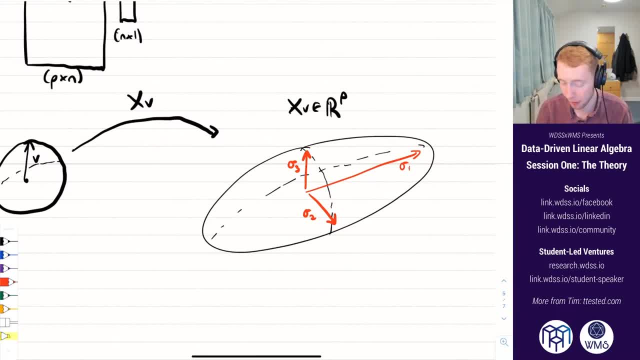 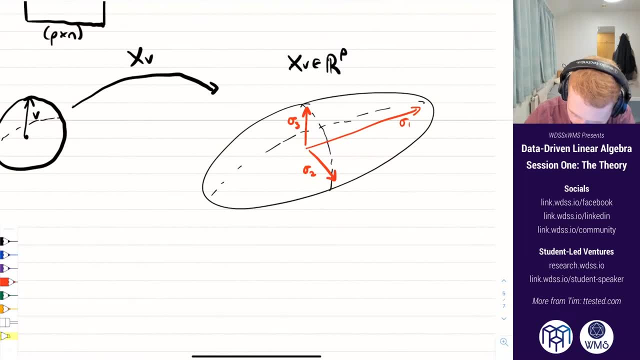 And we have some million dimensional hypersphere, And so that's what the singular values could give us. And then these directions. here, these are the vectors u1, u2, and u3.. So, essentially, u and sigma tell us how this unit sphere gets mapped by x into this new space. 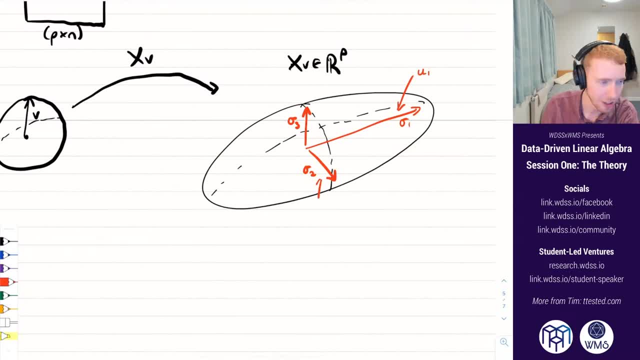 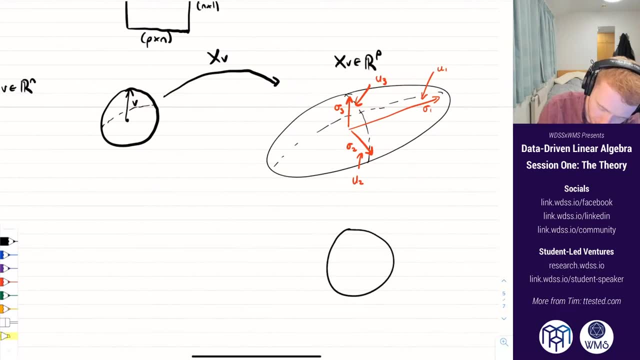 And so I think my screen has frozen again, So we'll just give it a bit of time to catch up. There we go, Okay, And then what the matrix v is going to tell us is what happens when we do the reverse. Let's take u in the space, rp. 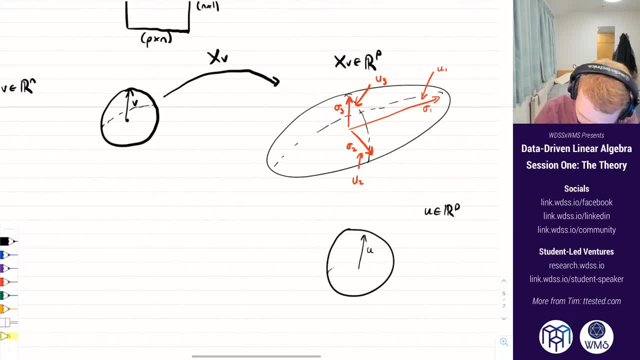 So again just some u here in this unit sphere in rp, And then we map this backwards using u pre-multiplied with x And that's going to give us another ellipse Like this And this is going to have a singular. so this is going to have principal axes here. 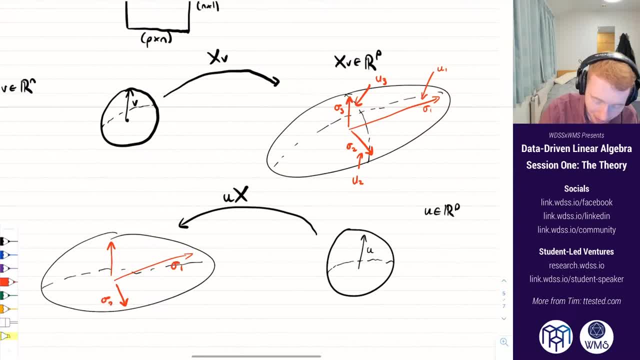 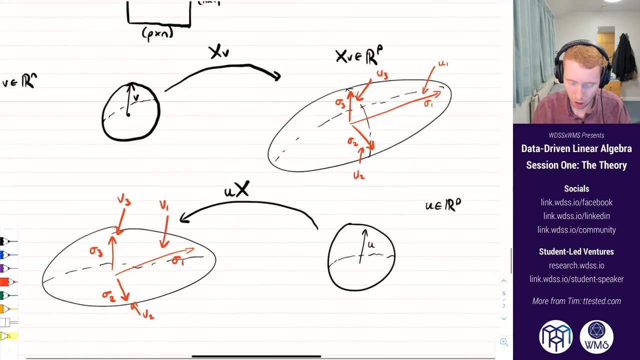 And these are still going to have directions, sorry magnitudes, given by these sigmas, But now their directions are represented by v1,, v2, and v3, etc. So that's kind of the geometric intuition of what the singular value decomposition is doing. 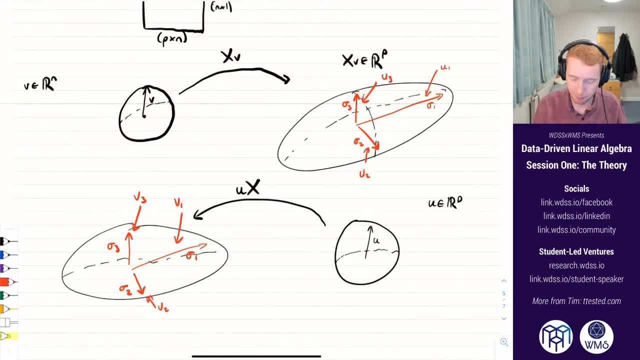 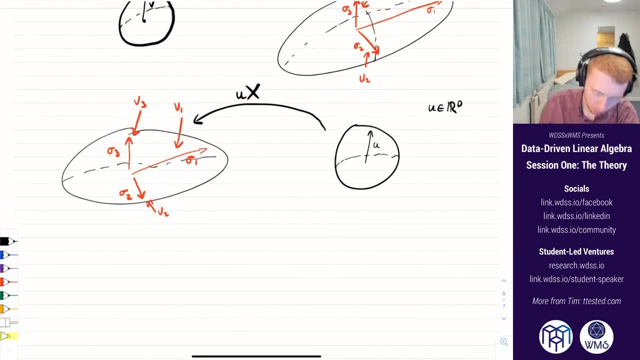 It's telling us when we're mapping forwards and backwards, mapping these spheres, you know how do we rotate things and how do we stretch them, And so we're coming close to wrapping up now, But the final point I want to leave you with is that we've represented x. 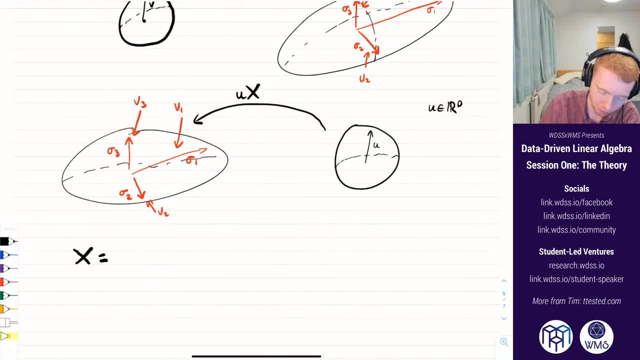 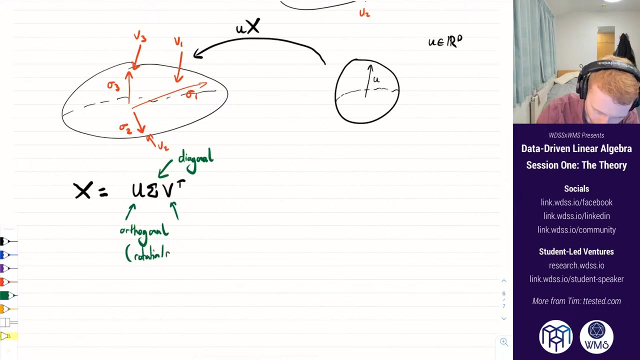 which was any matrix. remember that the singular value decomposition exists for any matrix. as u, sigma and v transpose, These are orthogonal And this matrix sigma is diagonal. In other words, geometrically, u and v are rotations or reflections. 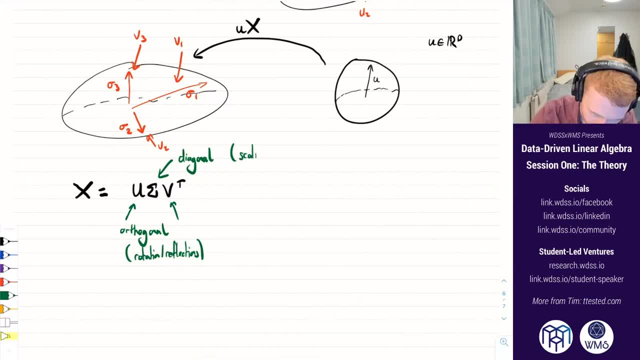 And sigma is a scaling. You know, you might want to think for a moment why that is the case. But if we times by a diagonal matrix, all we do is stretch out our space. We don't rotate, skew or anything like that. 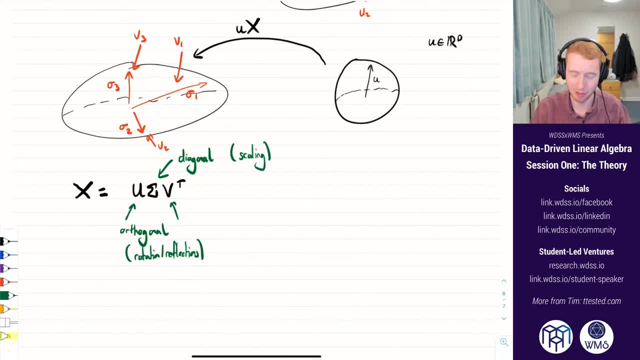 Sorry, we might skew if you scale by different amounts in different dimensions. And so what the singular value decomposition tells us in a geometric sense is that any matrix can be represented, any transformation can be represented, as a rotation onto the right axis, then a scaling along the kind of the principal axes of our dimension. 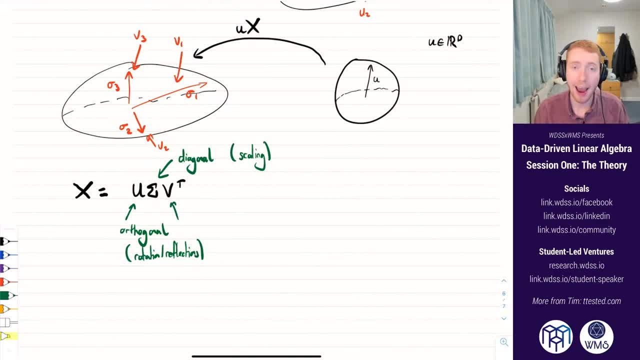 so along the actual x, y, z axes or whatever, and then one more rotation to get things back in line. So every single transformation can be represented in that form And you know that's a pretty beautiful idea, Although you know. 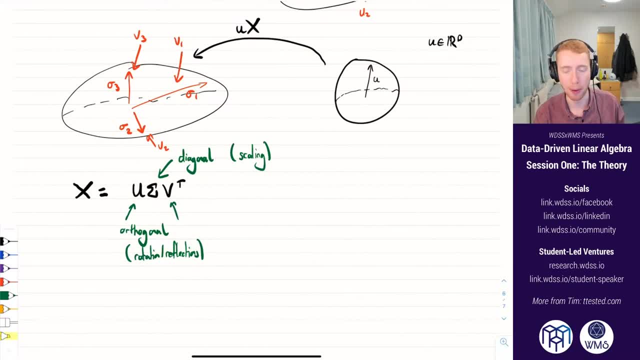 we're not here to talk about the whole thing. We're not here to talk about the whole thing. We're not here to talk about the whole thing, We're not here just for the mathematical beauty. And so that's where the next two sessions come in. 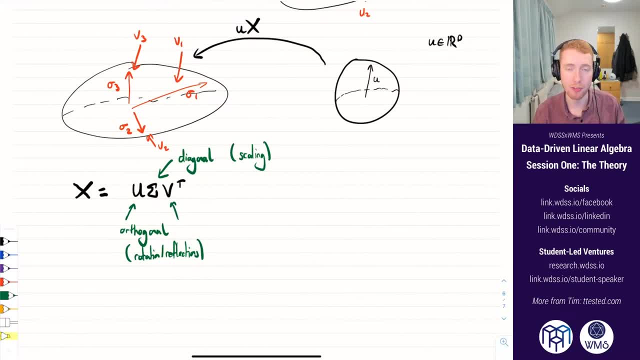 So in session two we'll talk about how to actually compute the singular value decomposition and kind of a bit more about what that actually tells us about the data and then how we can optimally truncate things. And in the third session, which is the really exciting bit, 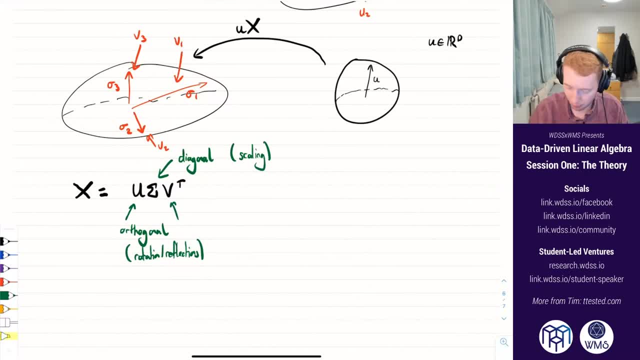 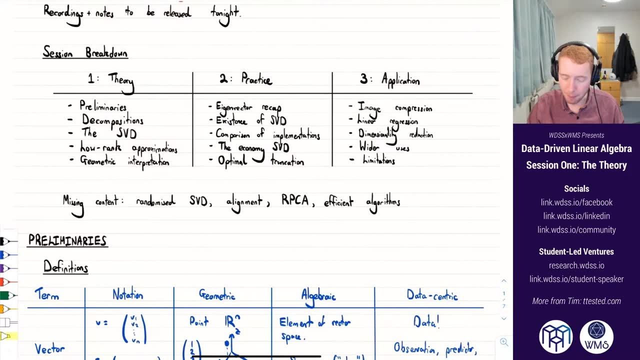 we're going to actually be coding things up for the purposes of- if we go back to the start here, three different main things to look at: So compressing images, how we can do linear regression, how we can reduce the dimension of our data.